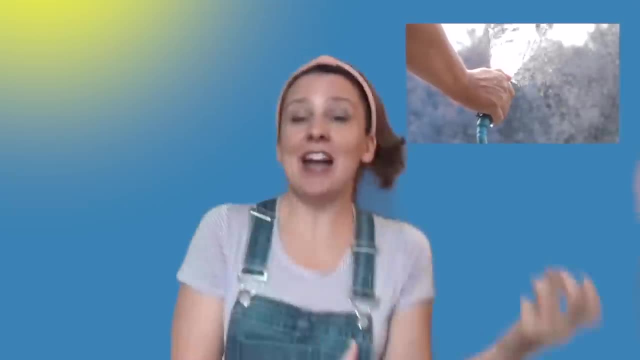 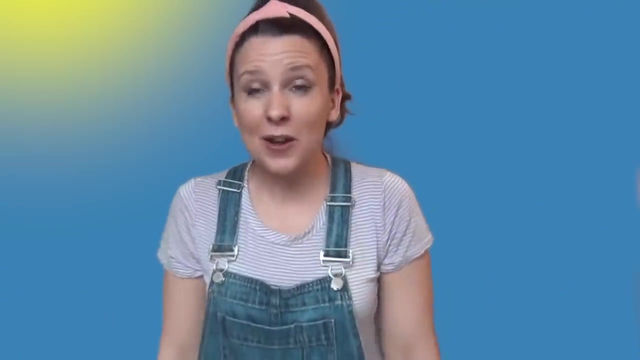 Hurry, hurry squirt the water. Hurry, hurry squirt the water. Hurry, hurry squirt the water. Ding ding, ding, ding ding. We did it. We put out the fire. Great job. Now we're gonna go back to the station slowly. 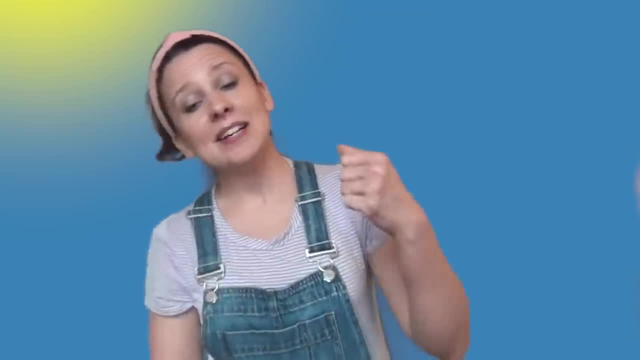 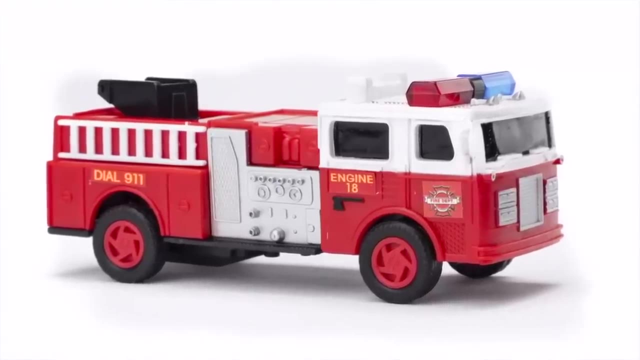 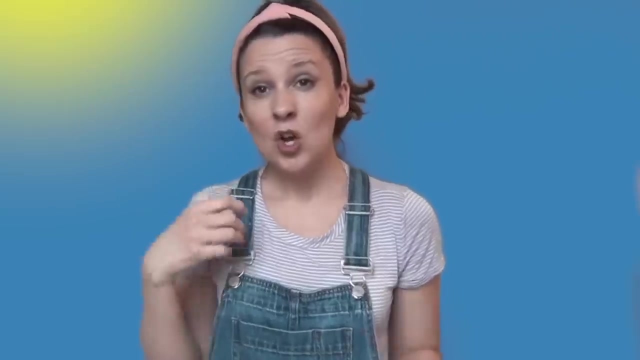 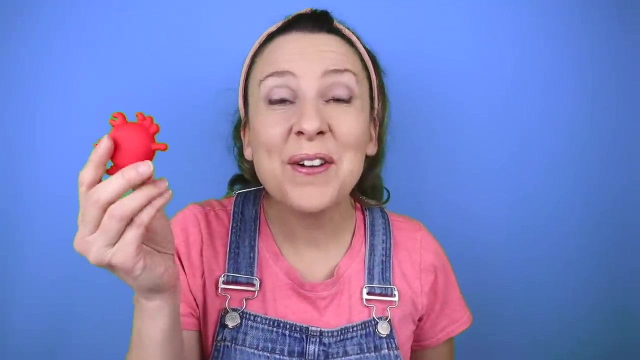 Slowly, slowly back to the station. Slowly, slowly back to the station. Slowly, slowly back to the station. Ding, ding, ding, ding ding. Great job, firefighters, High five, Woo Wow. Next is a crab. 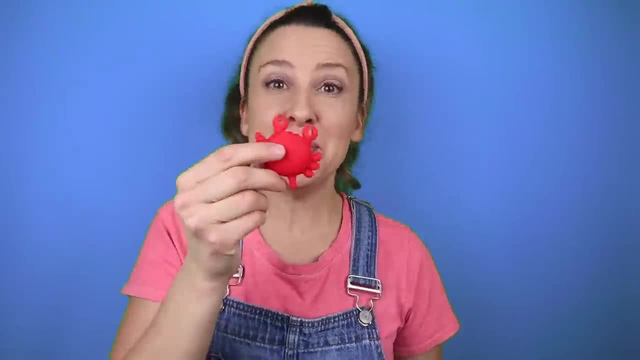 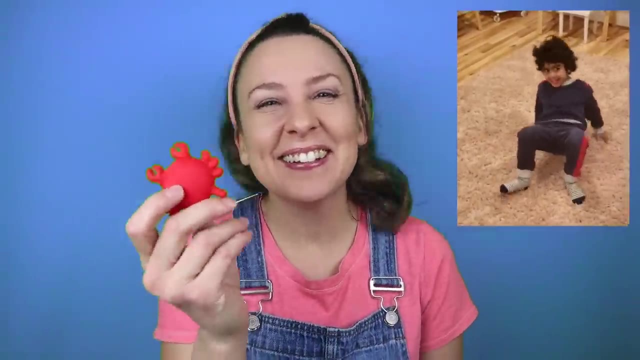 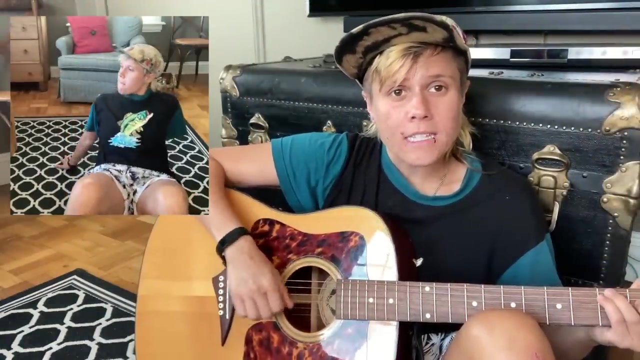 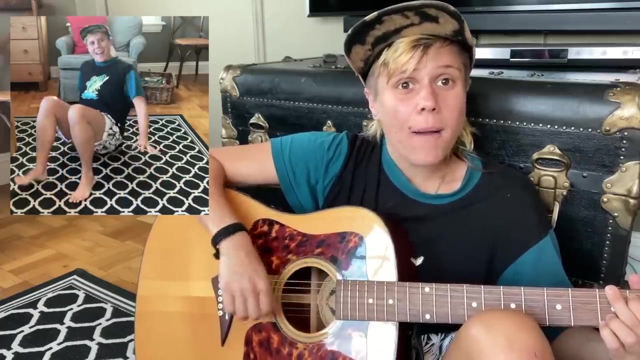 It's a little red crab. Can you walk like a crab? So much fun. Walk like a crab In the ocean blue. Yes, I'll put one hand back, One leg back. Do it again. Now I'm walking like a crabby crab. 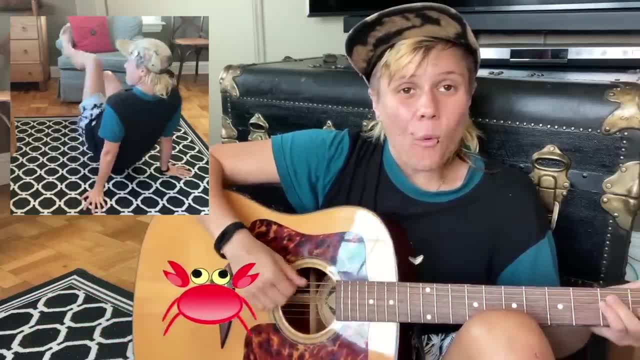 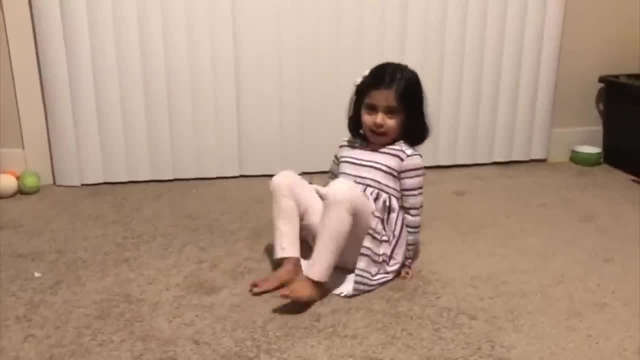 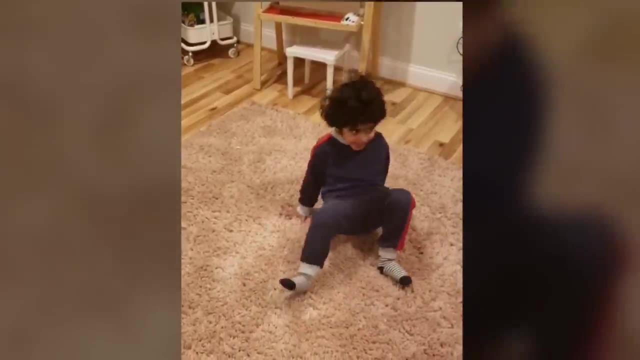 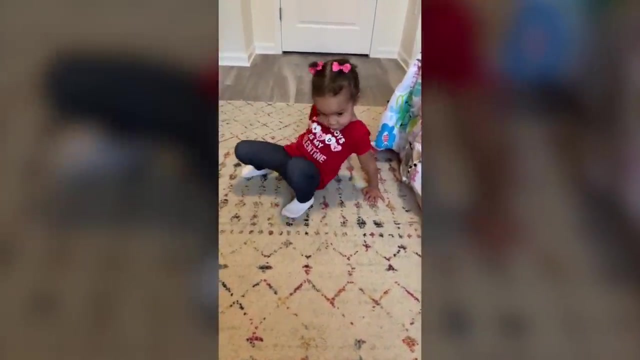 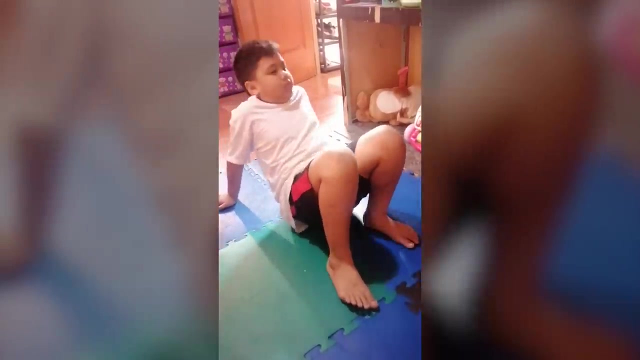 One hand back, One leg back, Do it again. Now. I'm walking like the crabby crabs. do Wow. I feel so much better. Let's keep walking. One hand back, One leg back, Do it again. Now we're walking like the crabby crabs. 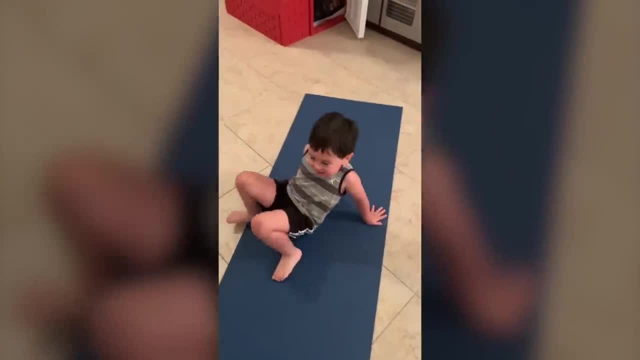 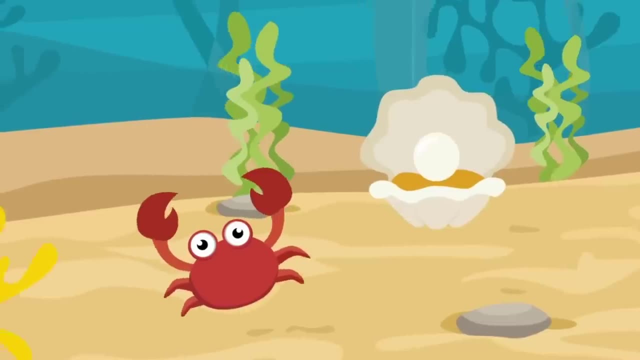 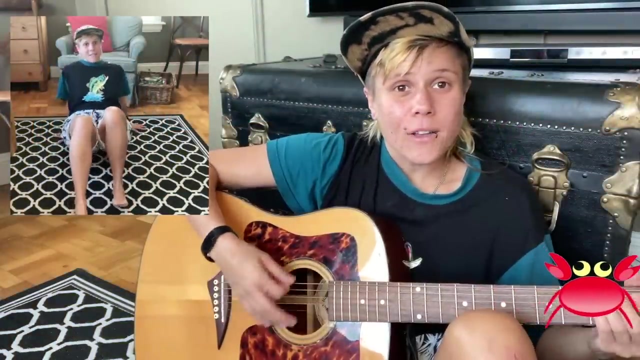 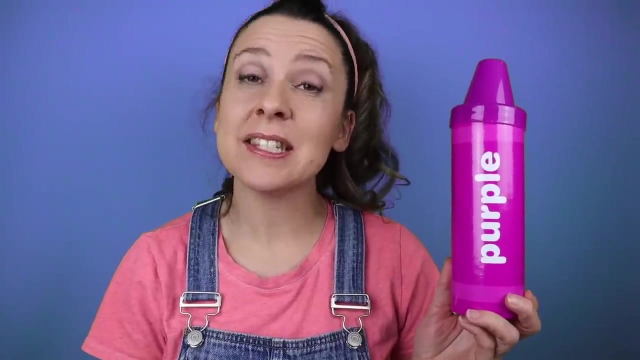 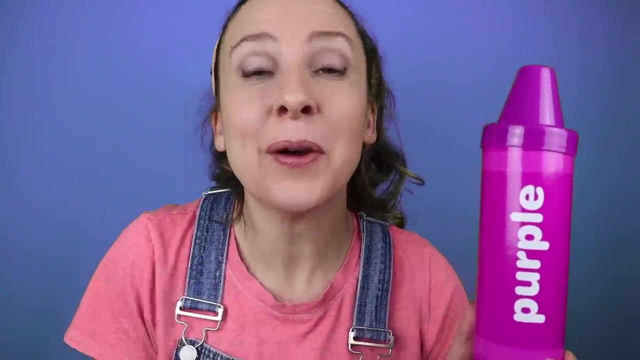 One hand back, One leg back. Do it again Now. we're walking like the crabby crabs do. Walking like crabby crabs do. What's this color? It's purple. Wow, Purple begins with P. Let's do the P sound. 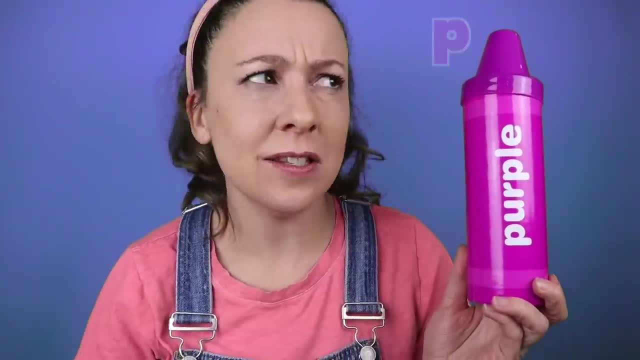 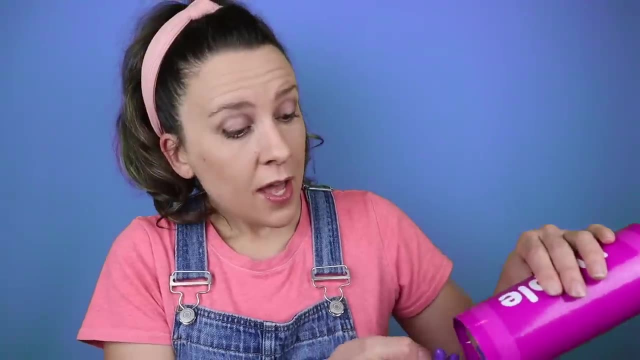 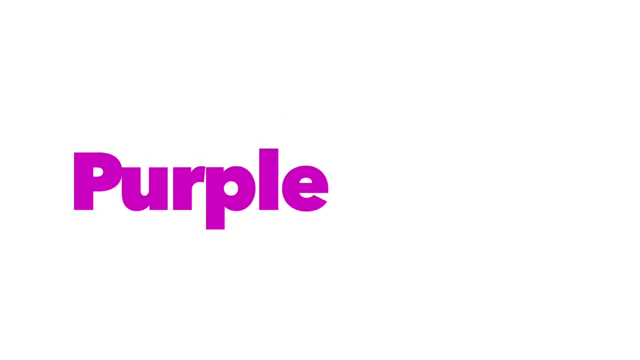 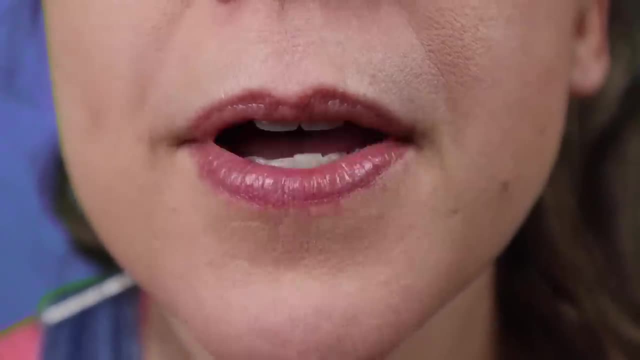 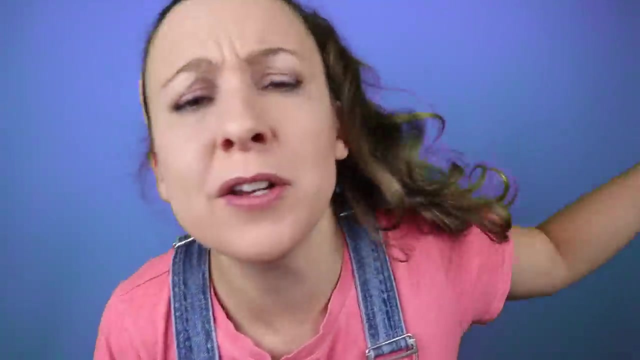 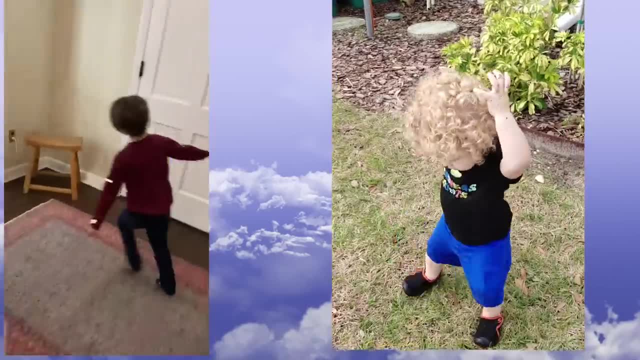 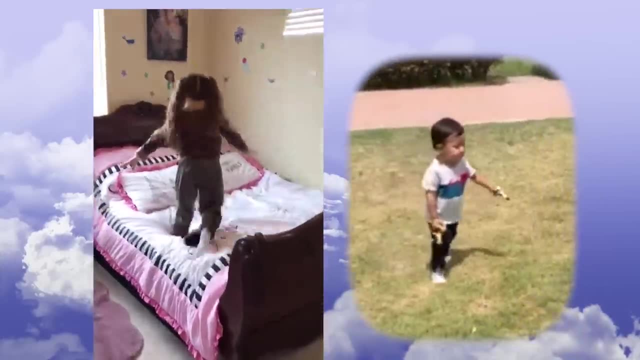 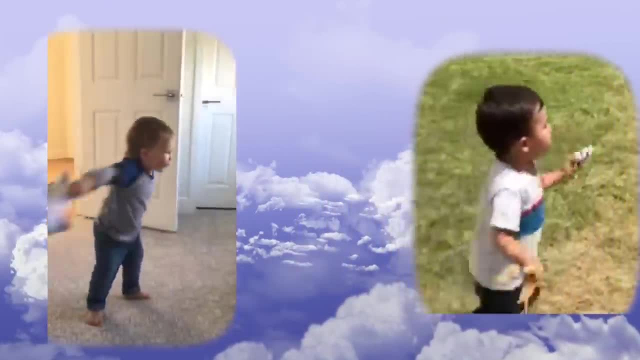 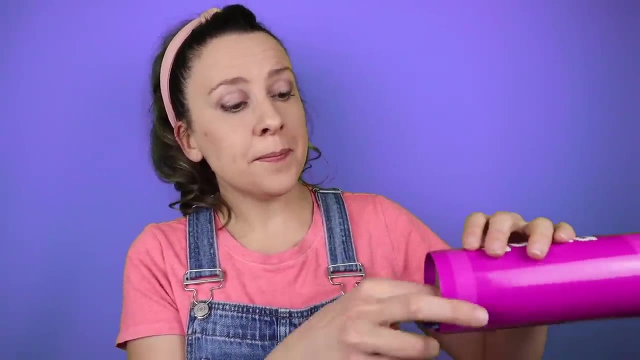 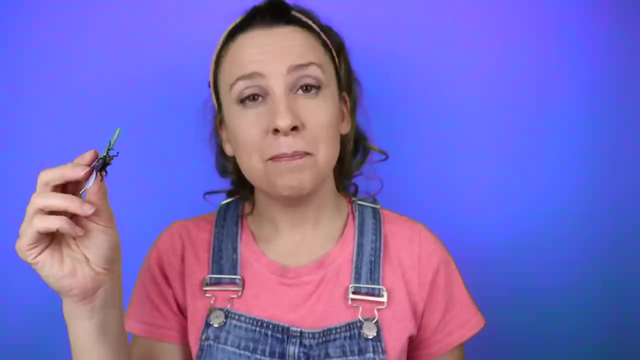 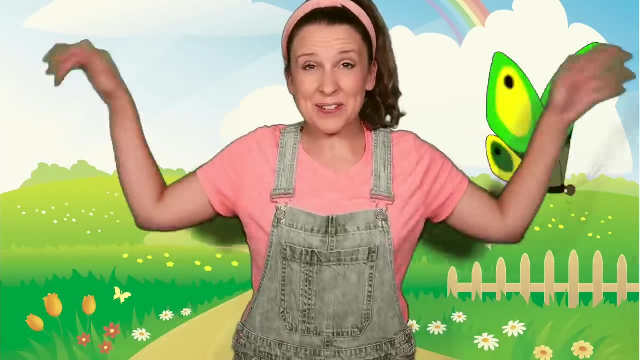 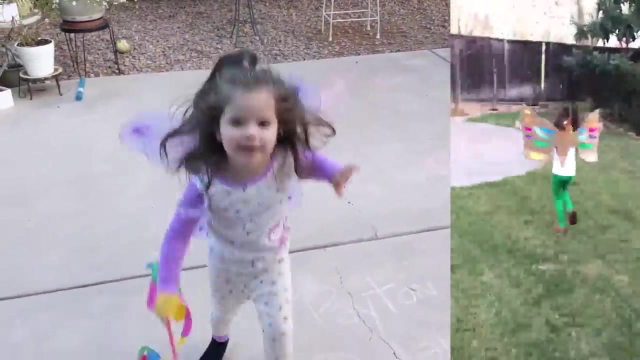 Mwah, Mwah, Mwah. Oh wow, It's a butterfly, A beautiful butterfly. Butterflies also fly. Let's pretend to be butterflies. Can you fly around with me? Good job, Fly, fly like a butterfly. Fly, fly like. 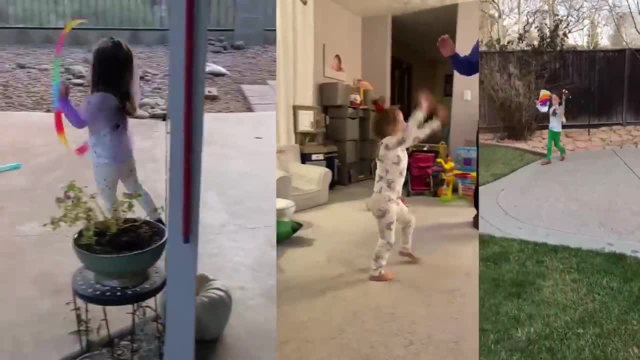 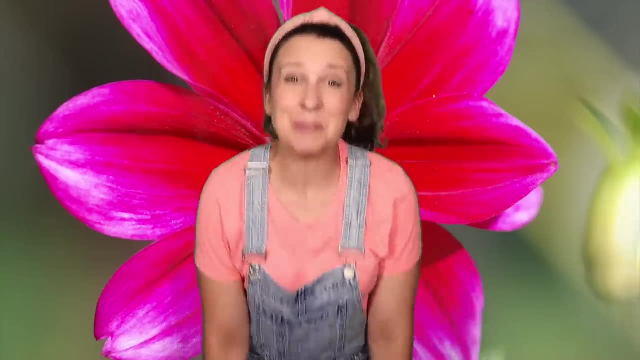 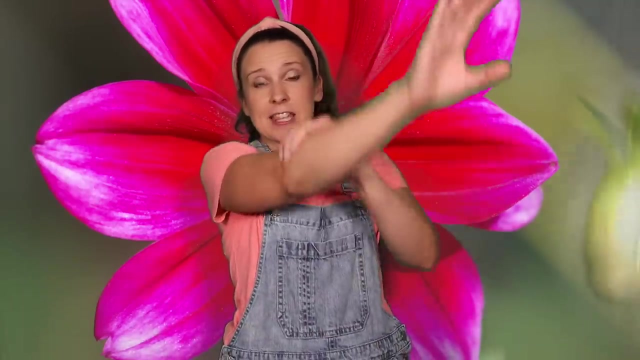 a butterfly Fly. fly like a butterfly Fly around the yard. Now let's pretend we land on a flower. Did you know that butterflies taste with their feet? Yum, yum, yum, This flower tastes yummy. Then they drink the nectar, like this Land on a flower and drink the. 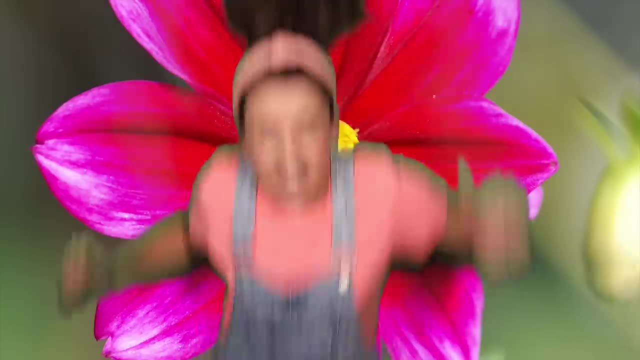 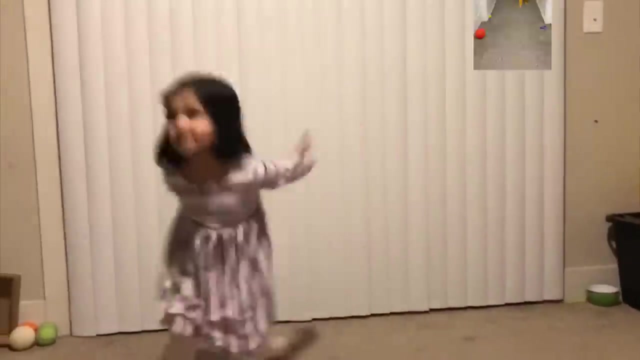 nectar. up Land on a flower and drink the nectar. up Land on a flower and drink the nectar up. The nectar tastes so yummy, Good job. Now let's fly around a little more. Are you getting tired? Let's take a rest on a leaf. 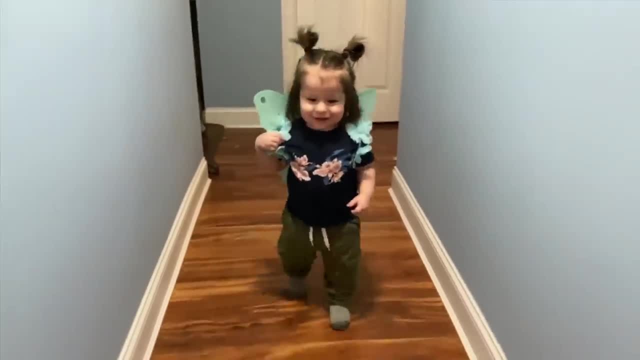 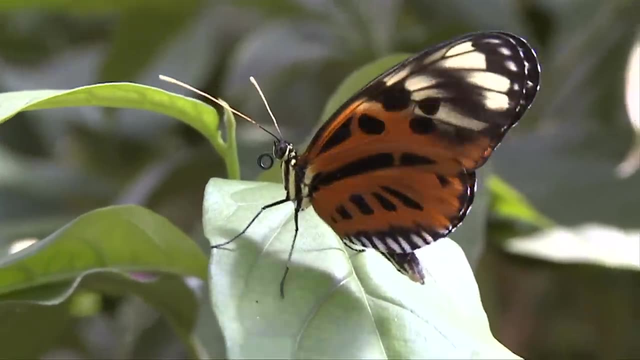 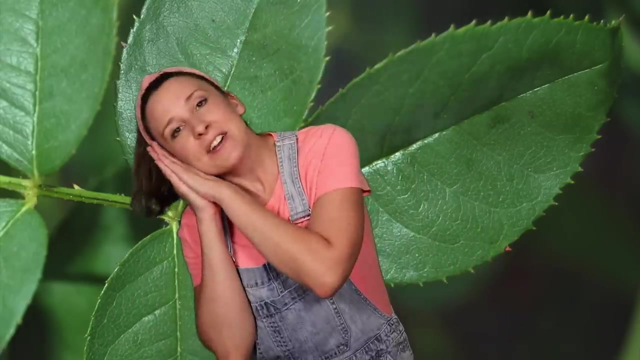 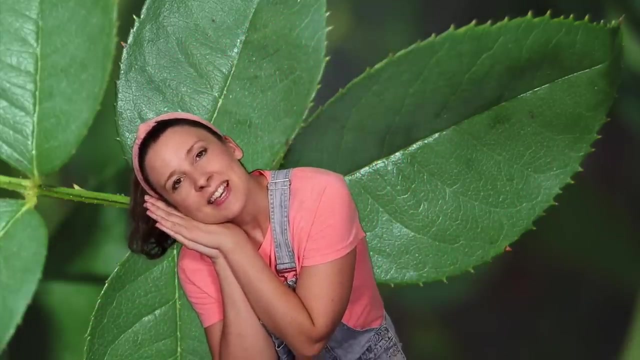 Butterflies don't sleep, but they rest. Let's rest on a leaf. Land on a leaf and take a rest. Land on a leaf and take a rest. Land on a leaf and take a rest because we are so tired. Ah, let's rest on this leaf. So nice to take a leaf. How are you feeling, Can you? 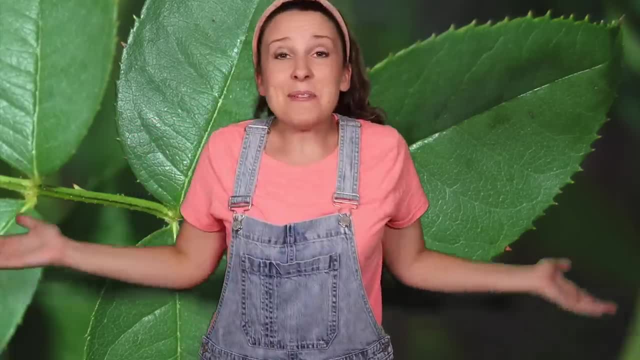 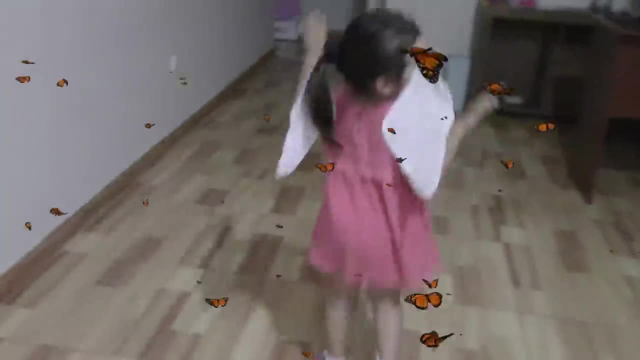 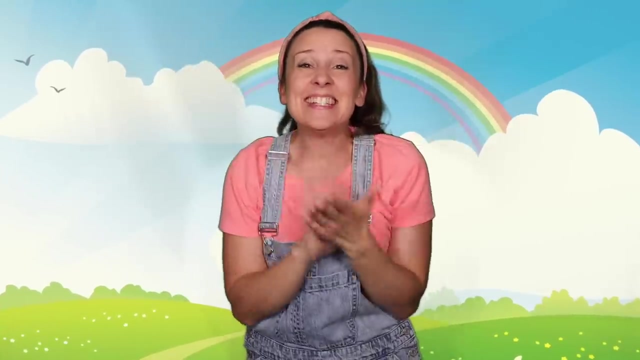 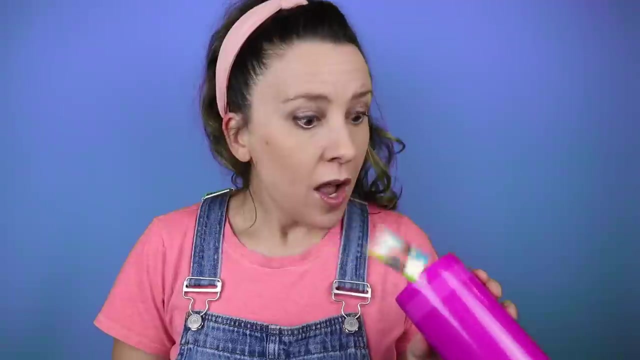 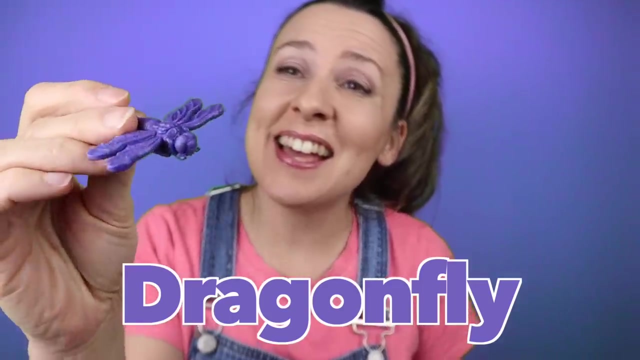 a rest. Let's get up and fly again. Are you ready? Fly, fly like a butterfly. Fly, fly like a butterfly. Fly, fly like a butterfly. Fly around the yard. Great job, Wow, You did a wonderful job being a butterfly. It's another thing that flies, It's a dragonfly. Can you fly? 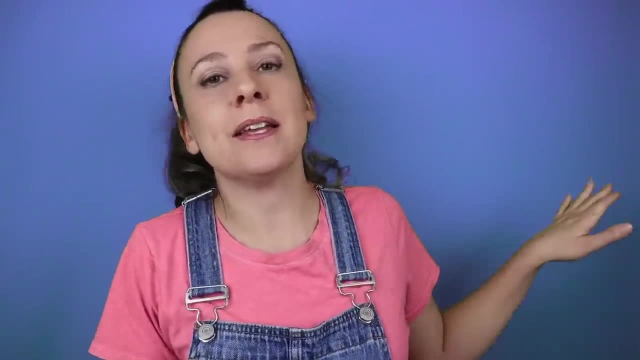 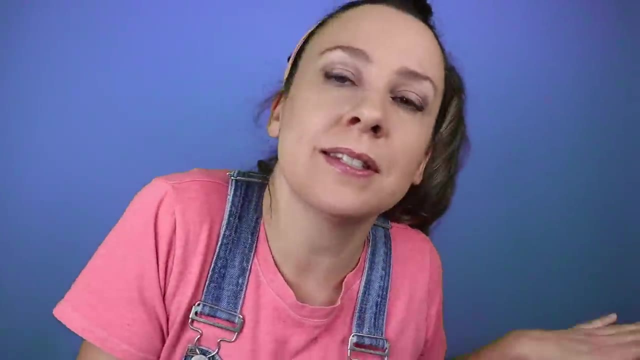 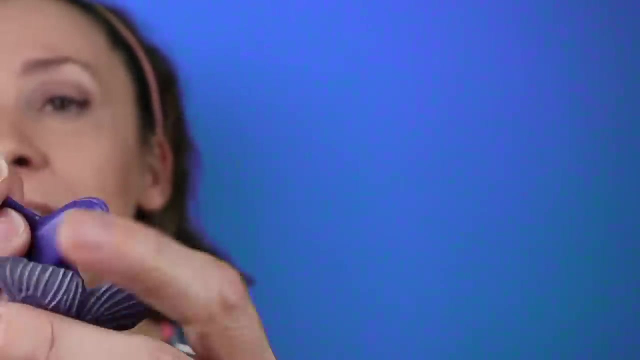 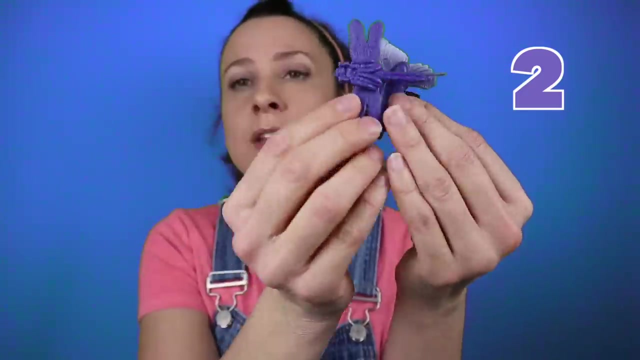 like a dragonfly. Maybe we can buzz a little bit. Can you do that? You're a dragonfly. Wow, I can't believe it. We found three things that fly: A butterfly, a plane and a dragonfly. One, two, three, Three things that fly This. 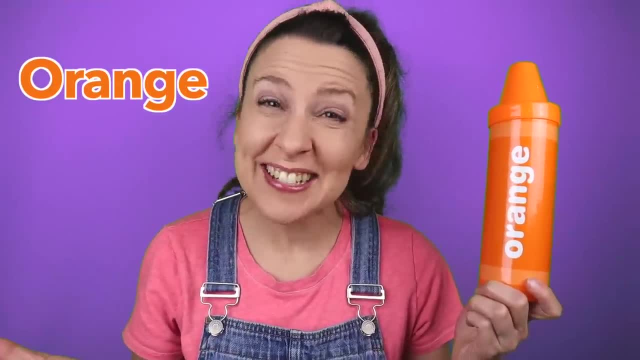 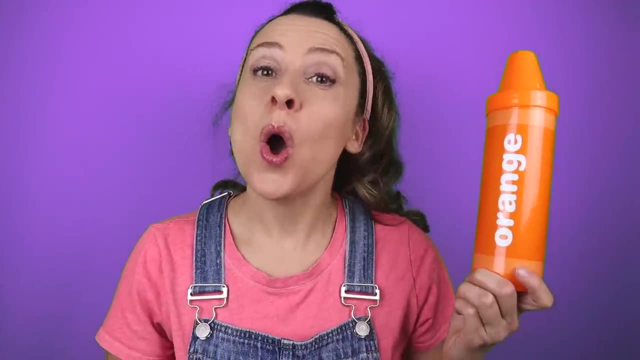 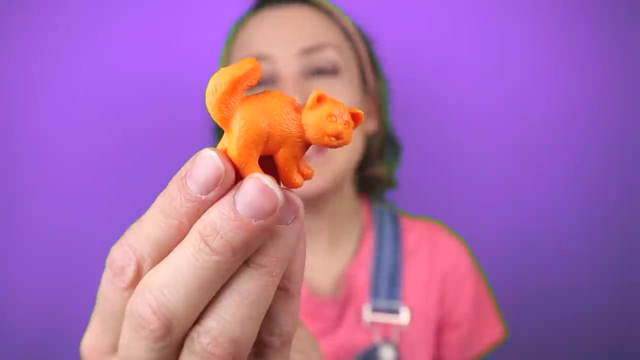 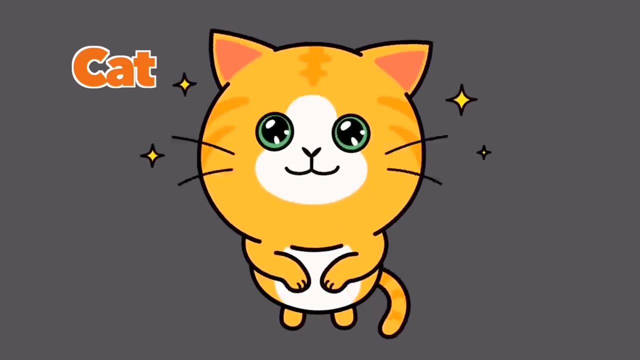 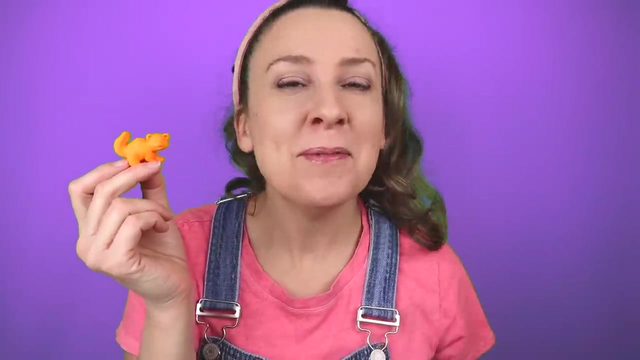 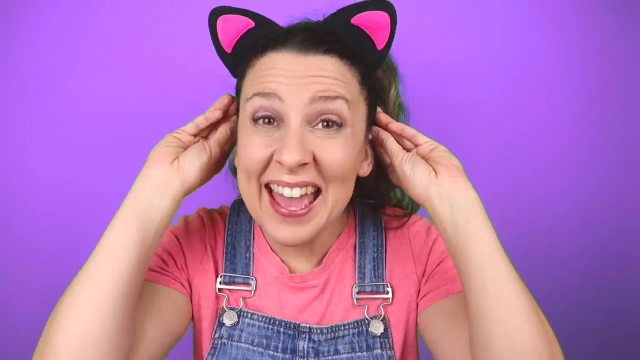 big crayon is orange. Yeah, You say open and it will open and we'll see what surprises are inside. Open, Wow, It's a little orange kitty cat, It's a cat. What does a cat say? I have some cat ears, Can you? 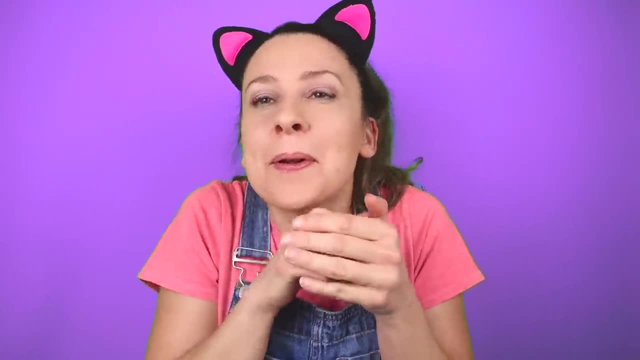 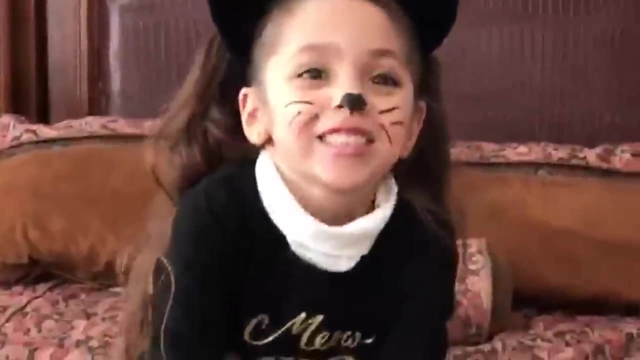 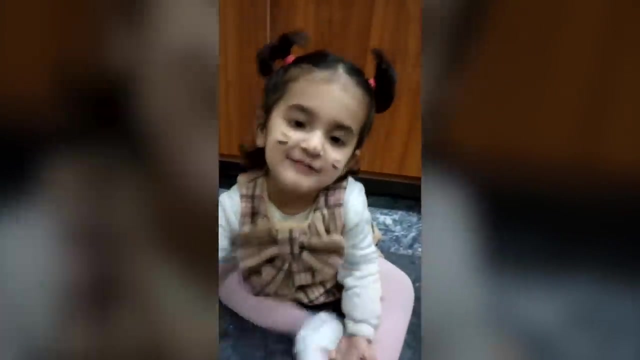 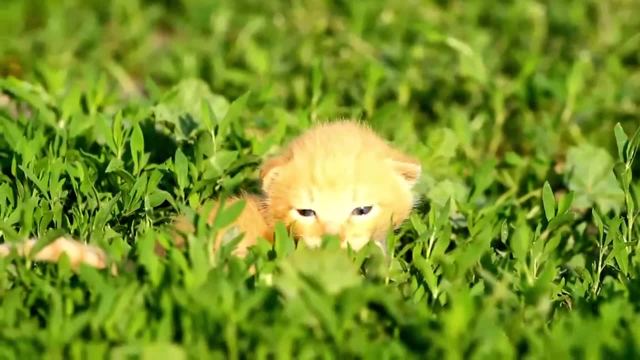 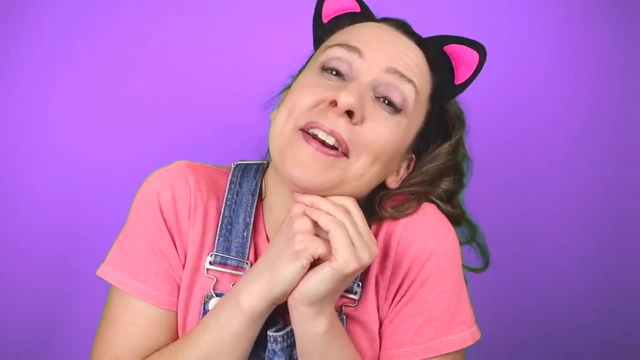 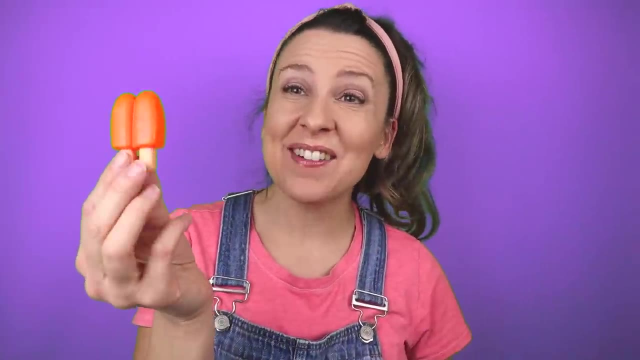 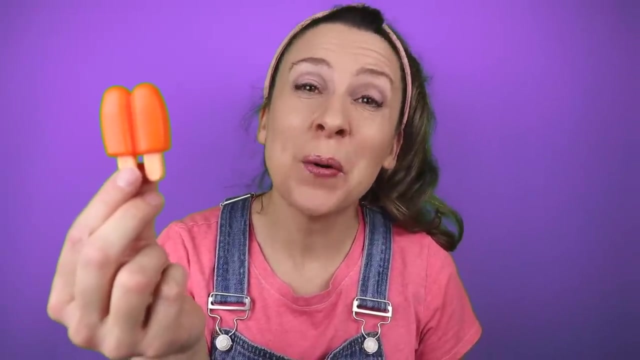 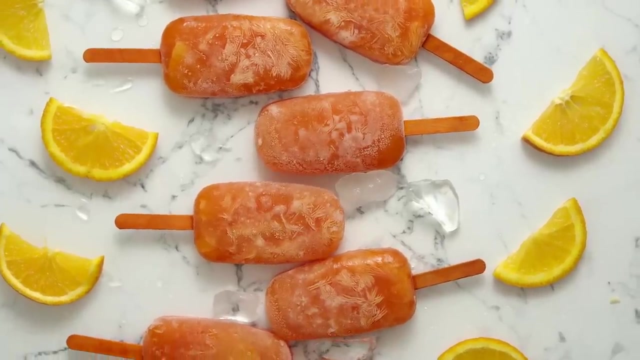 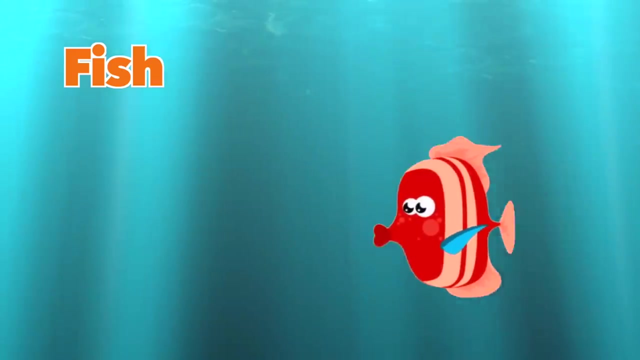 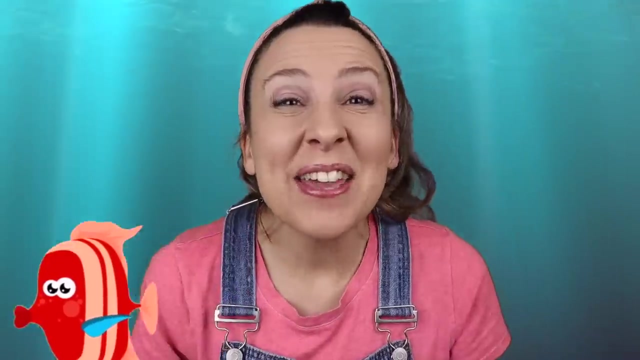 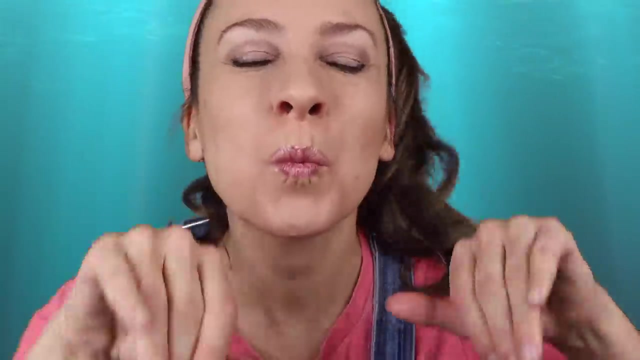 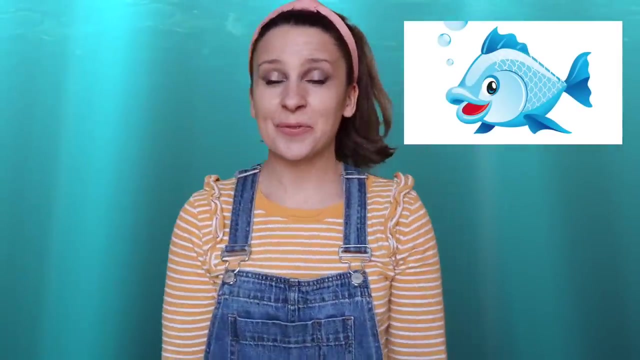 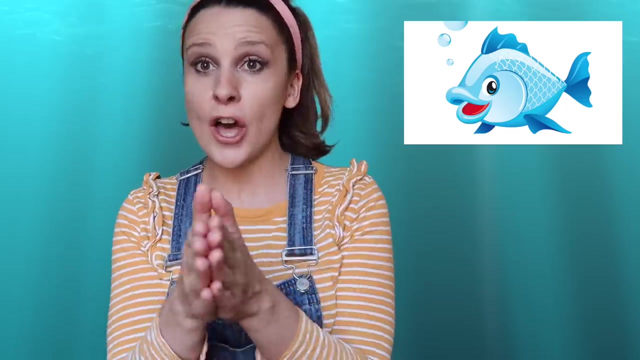 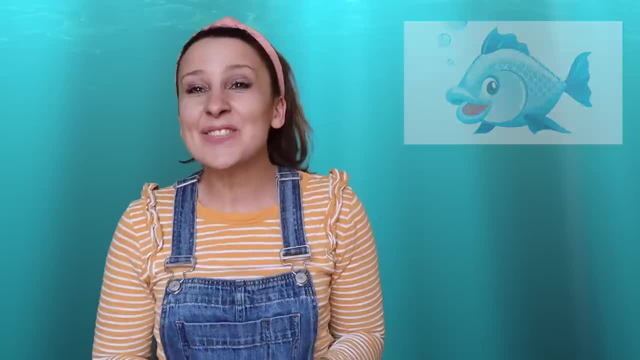 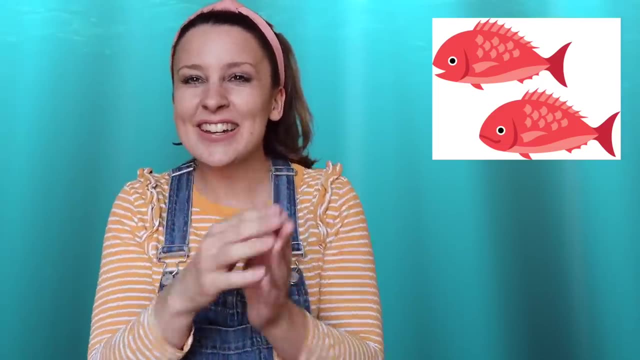 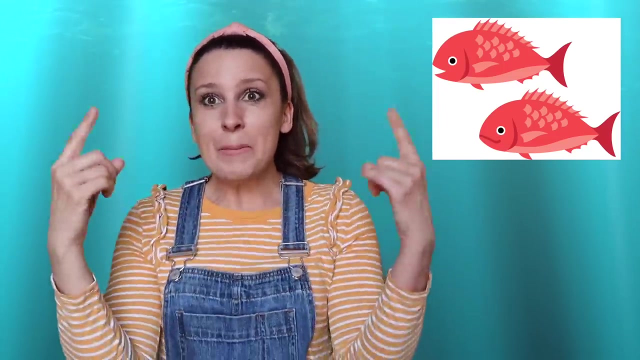 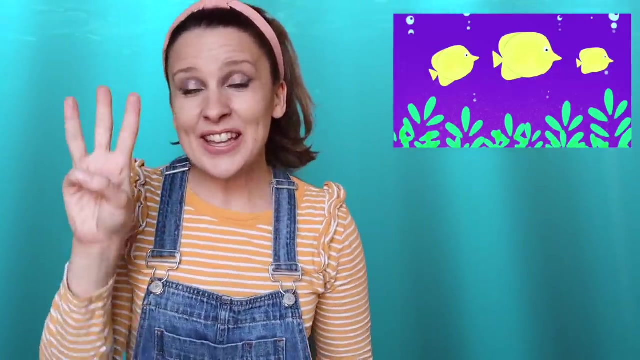 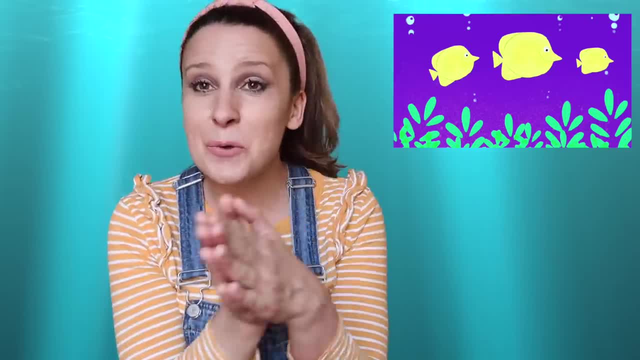 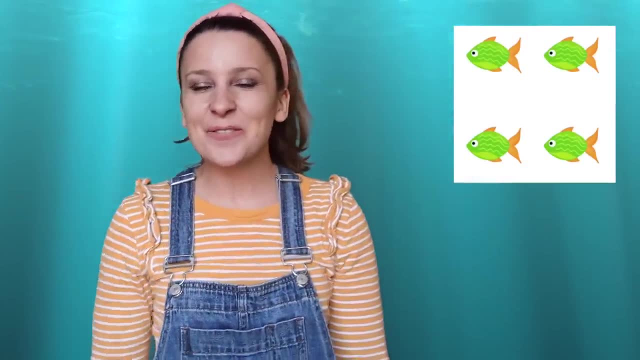 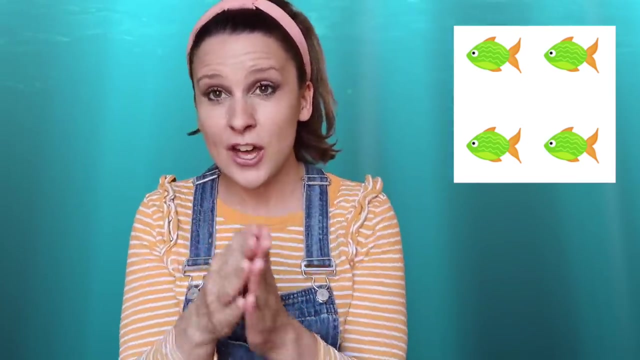 the water. Three little yellow fish swimming in the water- Bubble bubble, bubble, bubble pop. How about four green fish? I'm excited. Four little green fish swimming in the water. Four little green fish swimming in the water. Four little green fish swimming in the water, Bubble bubble. 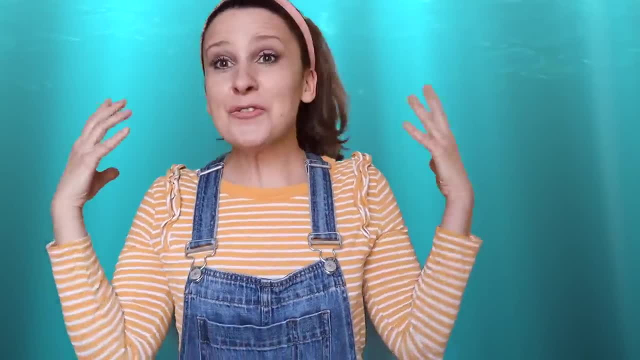 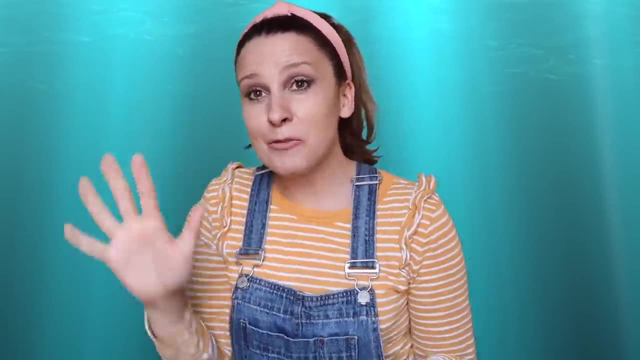 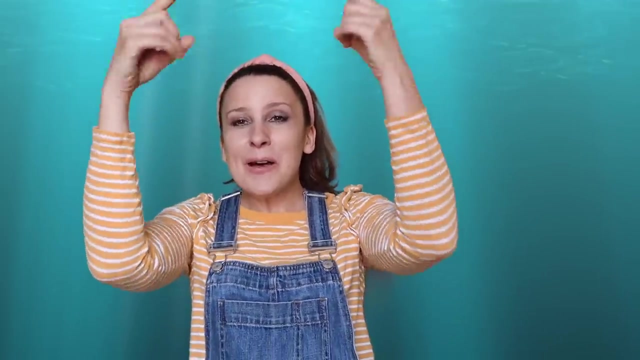 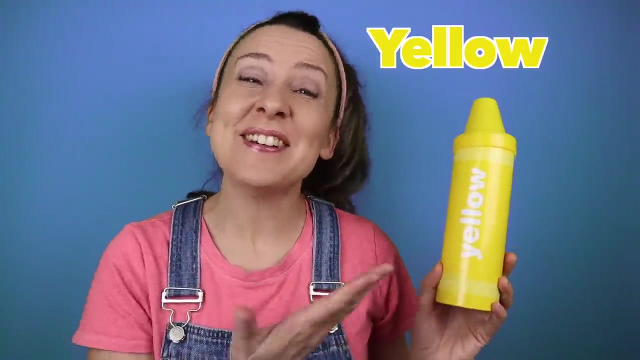 bubble, bubble pop. Now let's do five rainbow fish. Five little rainbow fish swimming in the water. Five little rainbow fish swimming in the water. Five little rainbow fish swimming in the water. Bubble, bubble, bubble, bubble pop. Wow, great job. Let's do our yellow crayon. Yay. 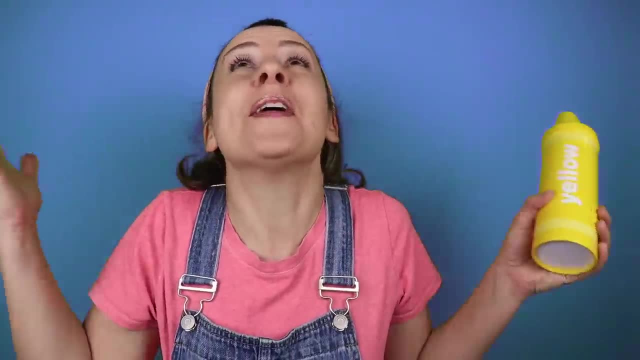 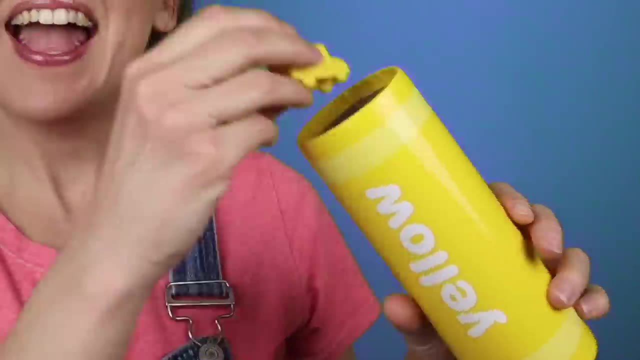 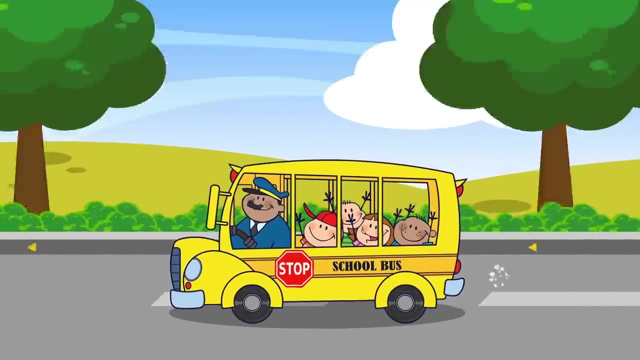 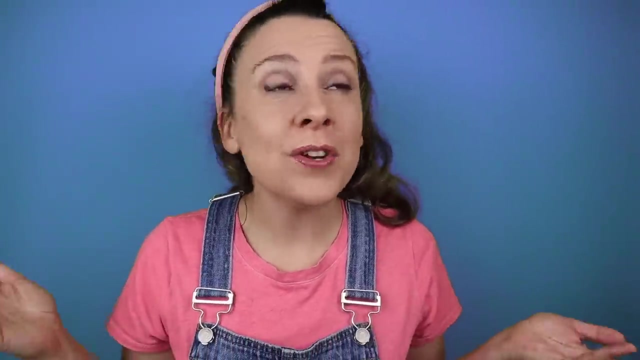 You say open, and it will open And show us the surprises. Open. Wow, it's a little yellow bus. Beep, beep, beep, beep. Can you say beep, beep, Beep, beep? Maybe if we say beep, beep, really loud. 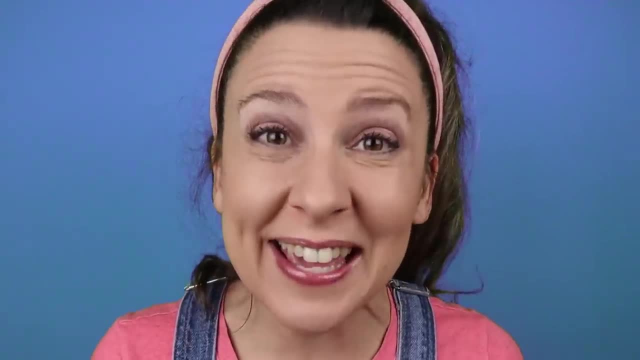 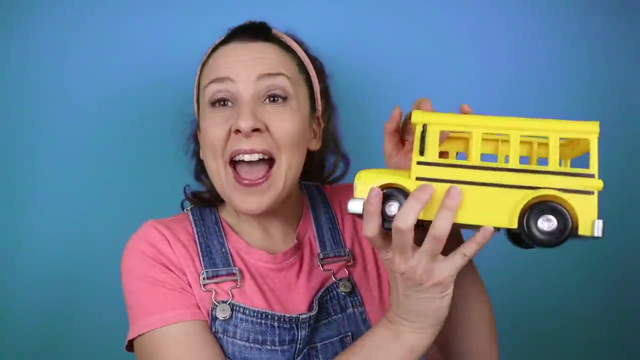 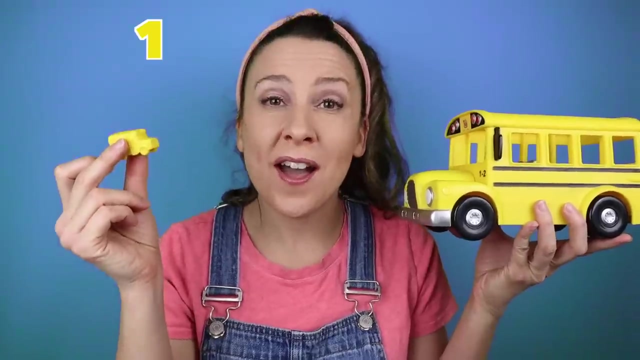 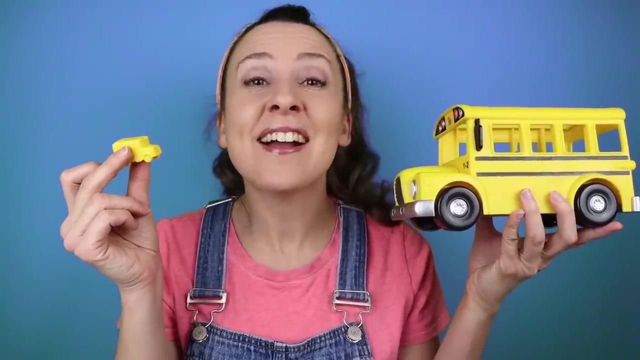 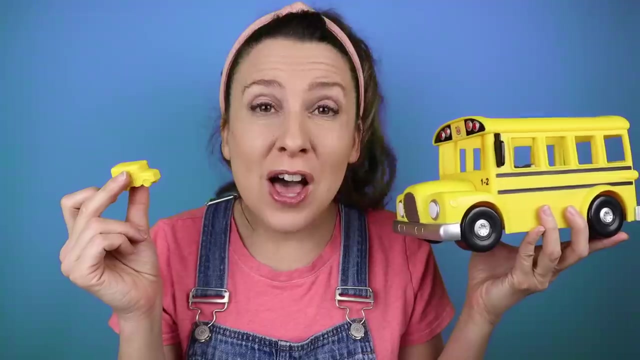 another bus will come out. Can you say that with me? Beep beep, Beep beep. Wow, another bus came out. Now we have two buses, One, two. Which bus is bigger? Yeah, this one is bigger. Which bus is smaller? Yeah, this is a little bus, So little, Such a little bus. 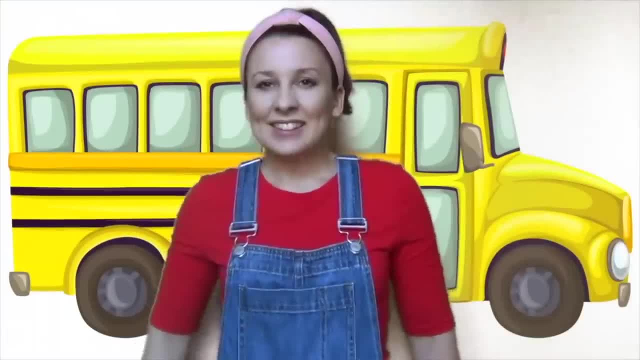 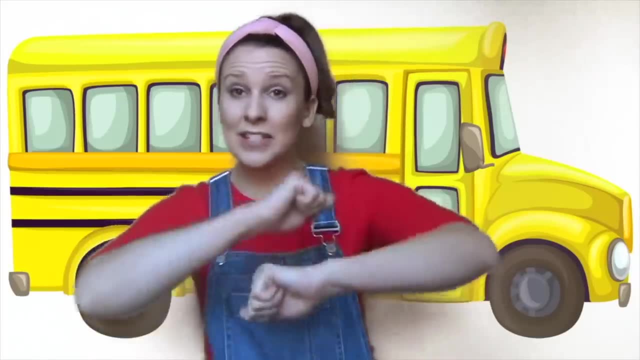 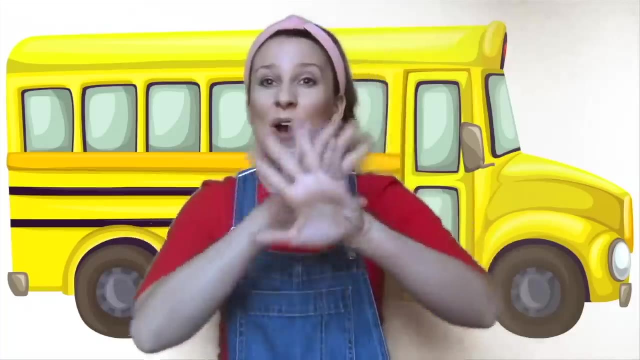 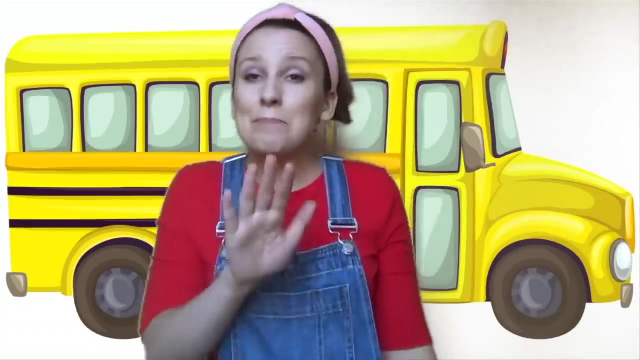 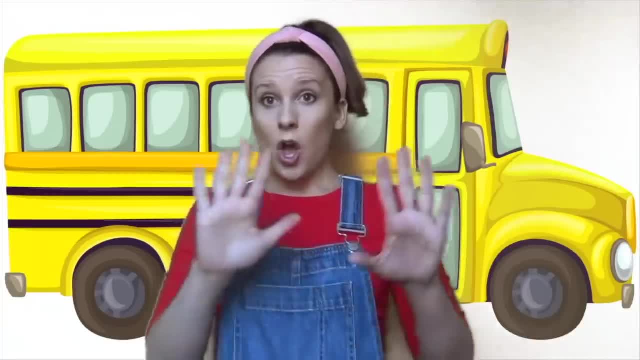 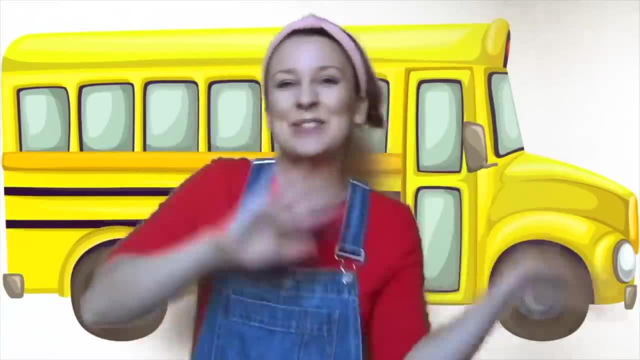 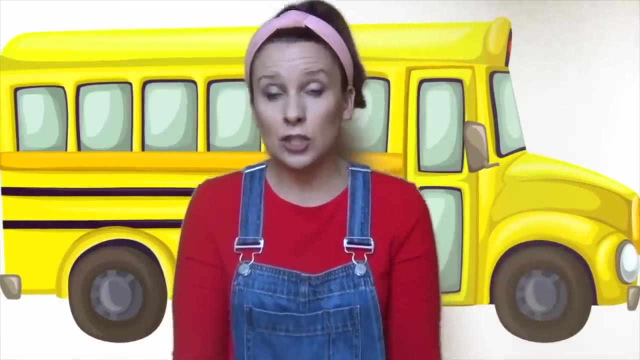 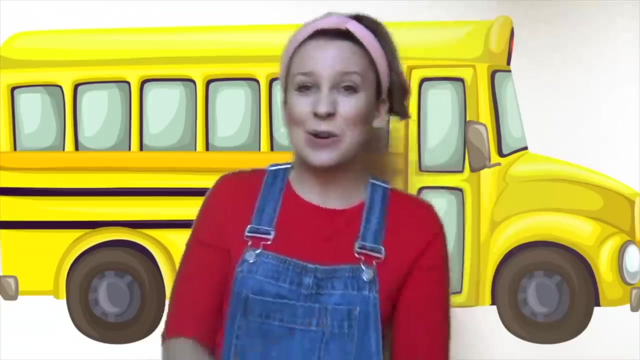 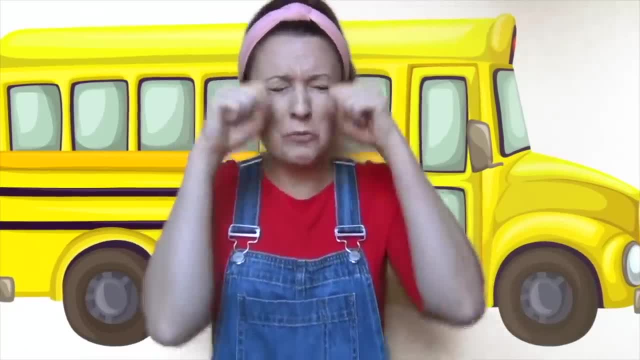 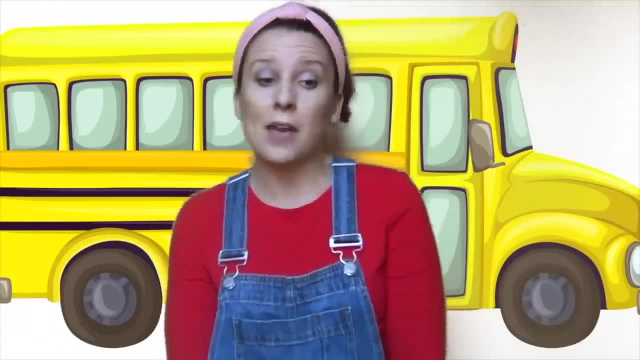 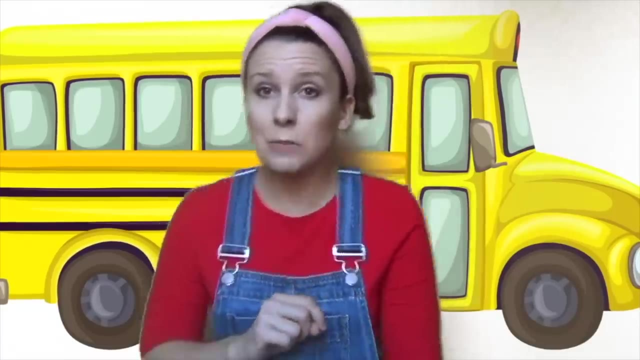 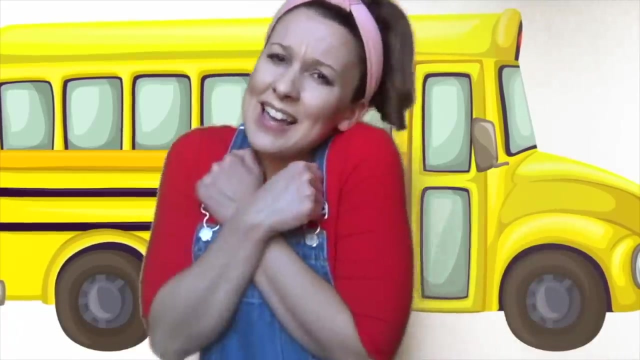 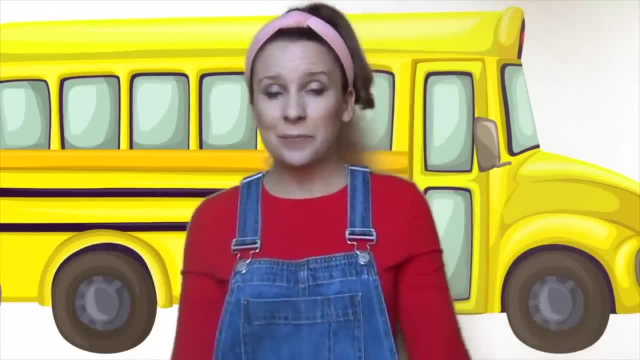 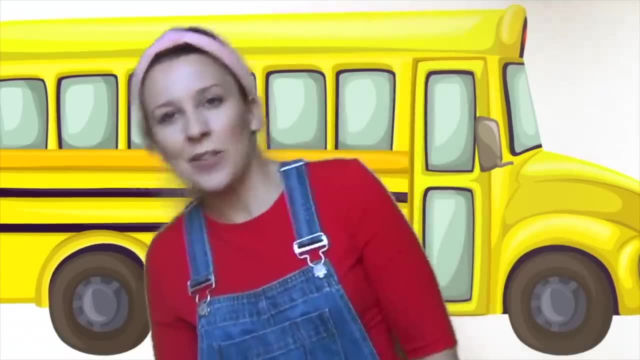 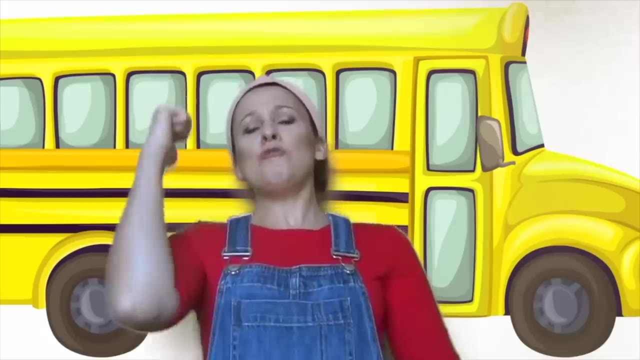 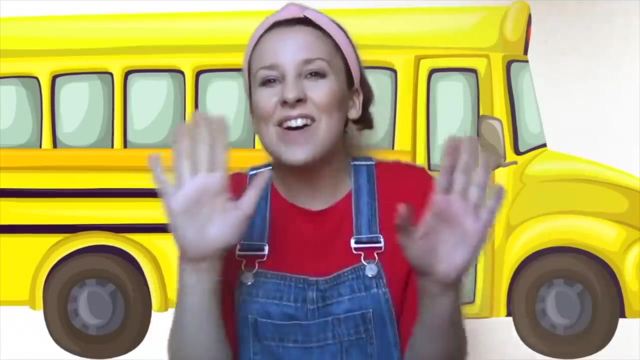 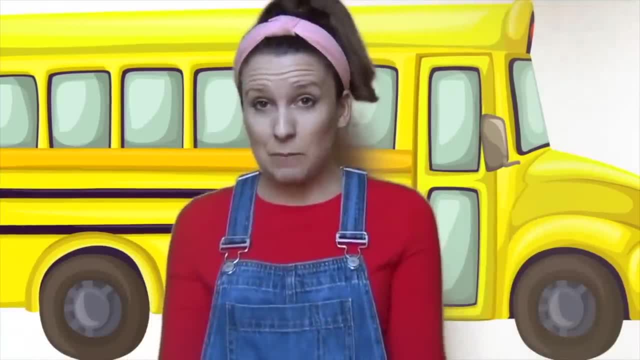 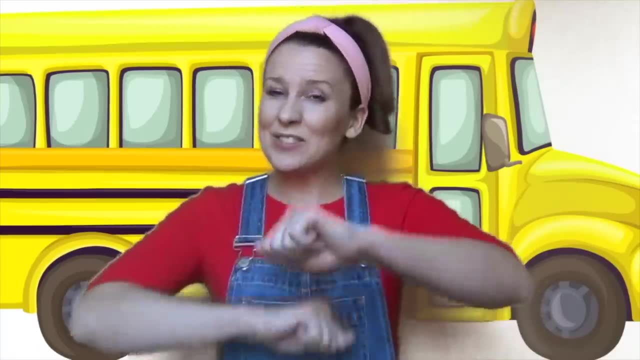 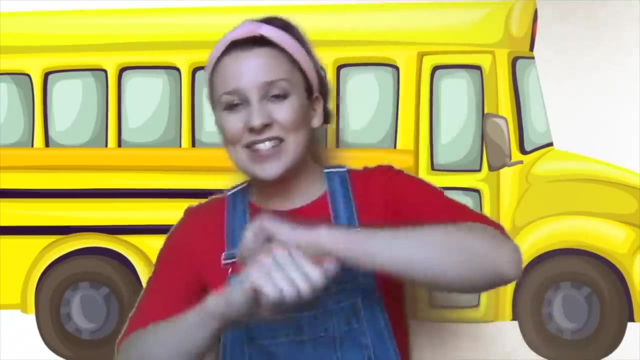 up and down, up and down. the people on the bus go up and down all through the town. Let's go back to the wheels. Can you do the wheels again? Great job. The wheels on the bus go round and round, round and round, round and round. 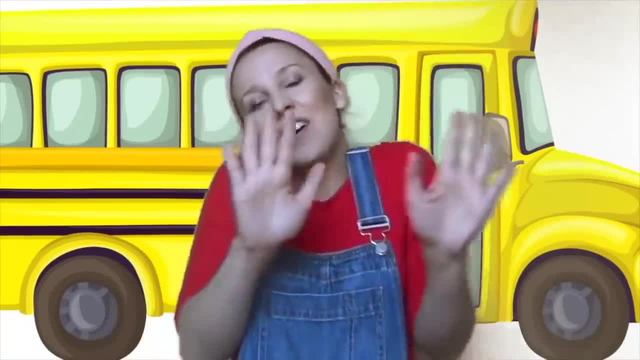 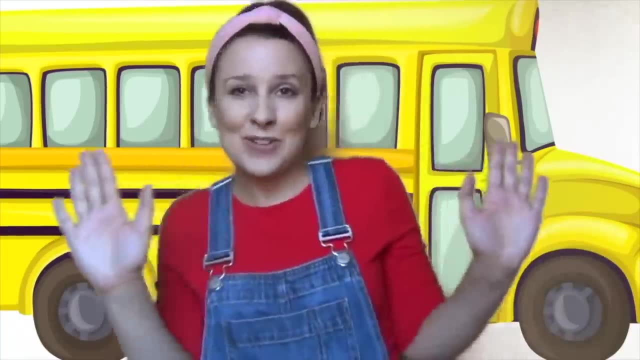 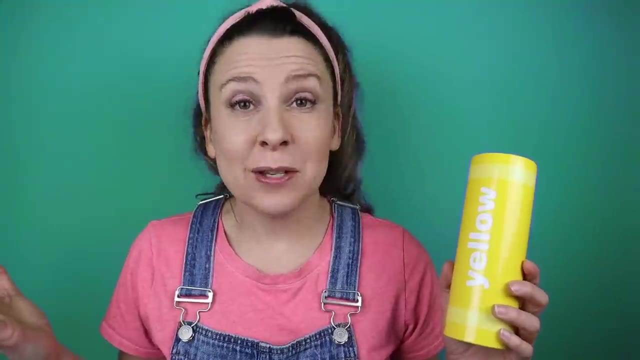 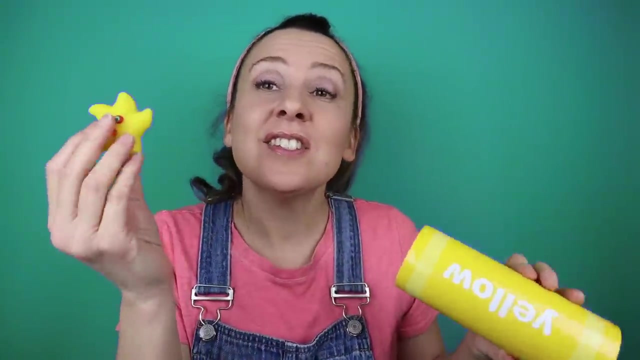 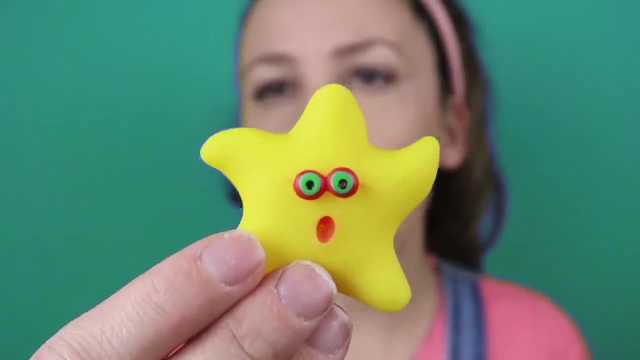 The wheels on the bus go round and round, all through the town, All through the town, All through the town. Yay, Can you clap? Let's see what's next. Wow, It's a little star, So beautiful. Can you help me get back up in the sky? 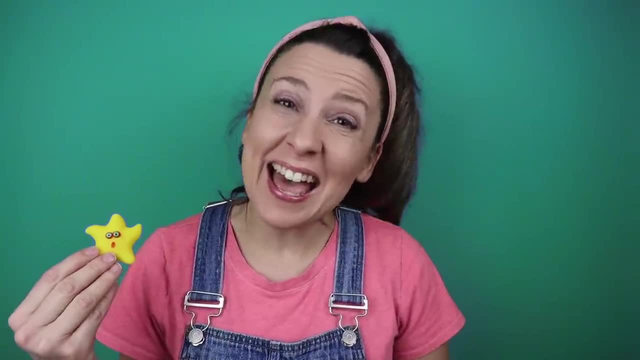 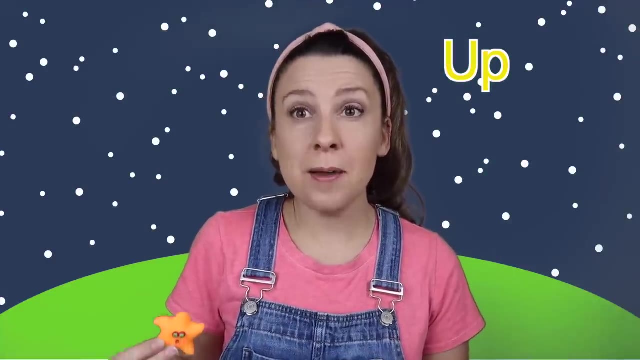 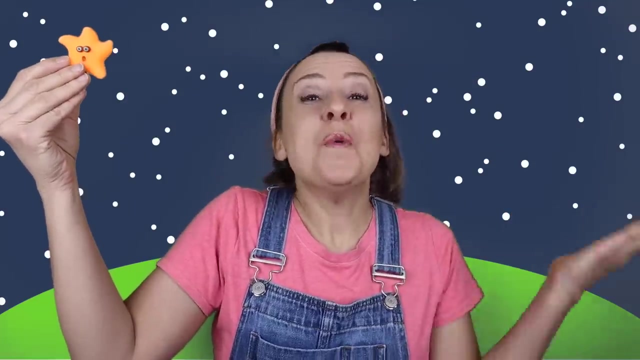 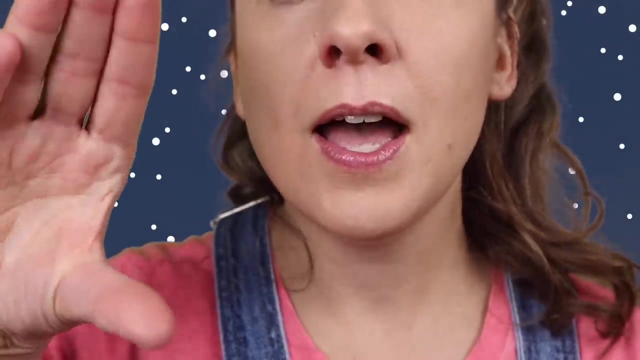 Let's help the star get back up in the sky. Say up and we'll help the star Up up, up, up, up. We got the star back up in the sky. Yay, Up up. Thank you. 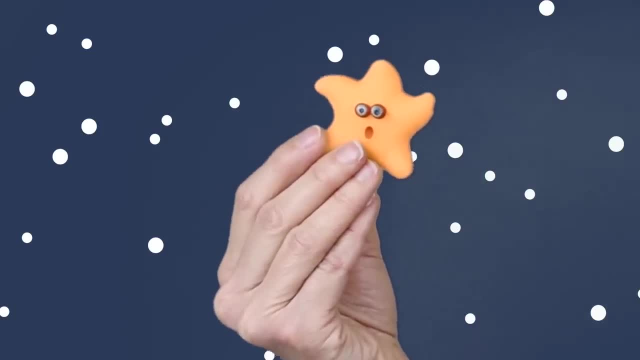 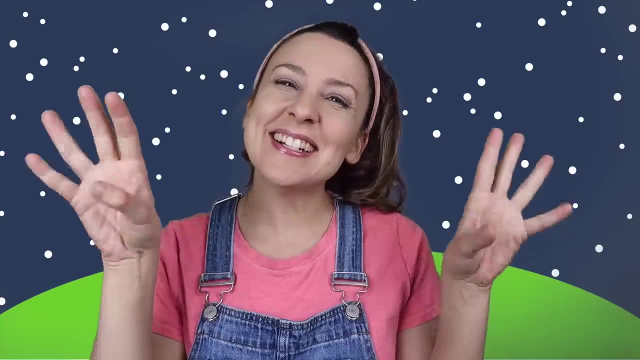 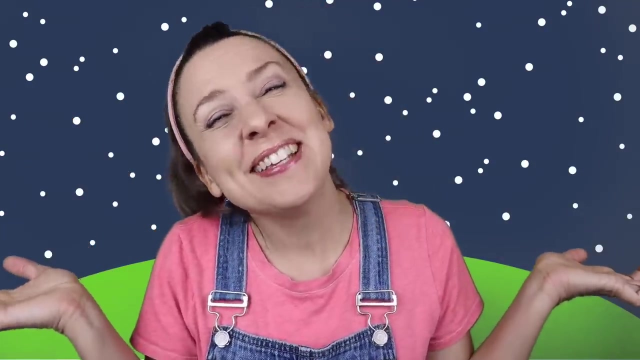 Thank you for helping me get back up in the sky. Let's sing a song. Let's sing Twinkle Twinkle Little Star, Get out your stars. Twinkle twinkle little star. How I wonder what you are Up above the world so high. 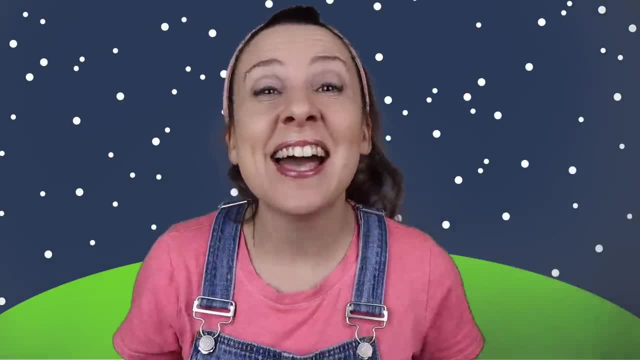 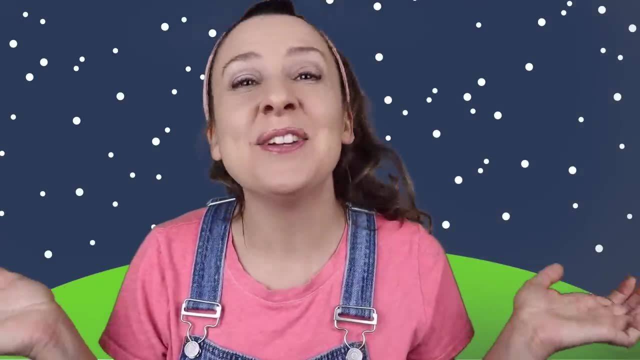 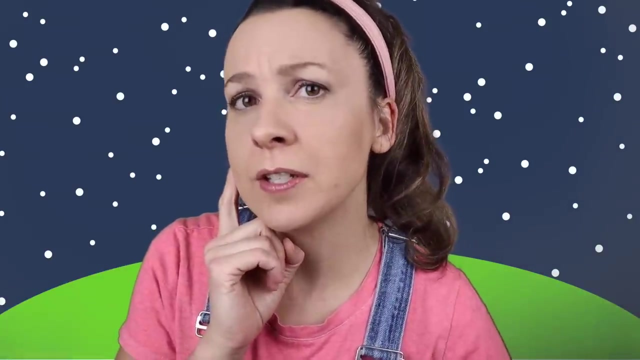 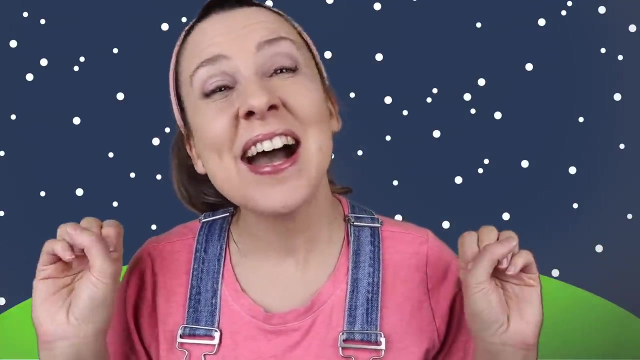 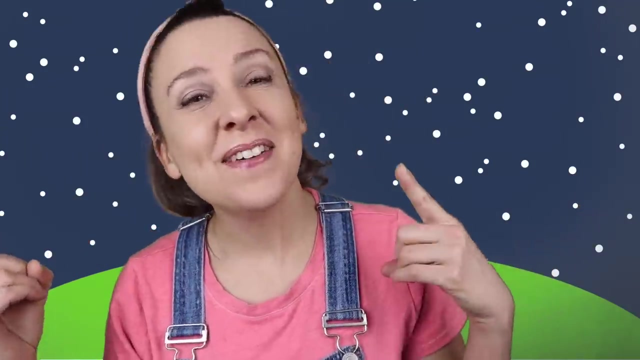 Like a diamond in the sky. Twinkle, twinkle, little star. How I wonder what you are. Good job, Can you fill in the words Twinkle, twinkle, little star? How I wonder what you are, Up above the world so high? 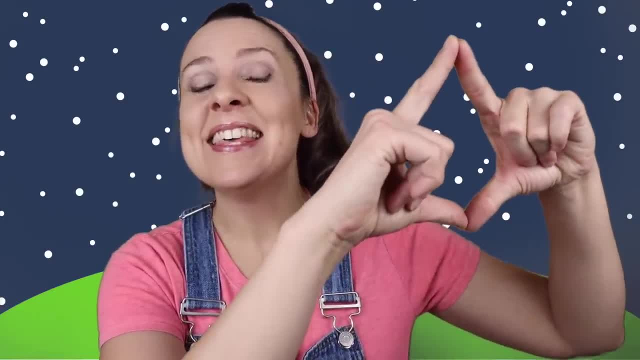 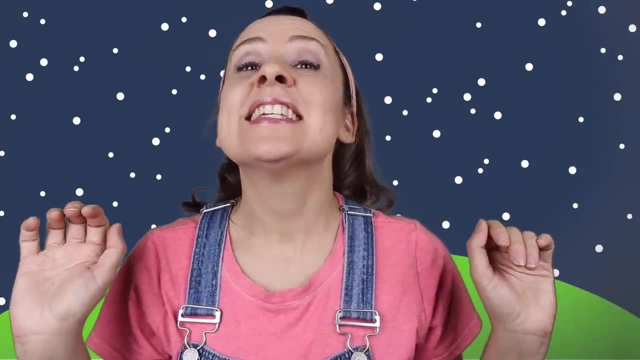 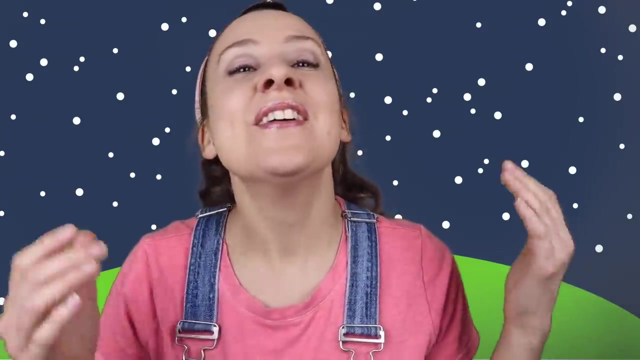 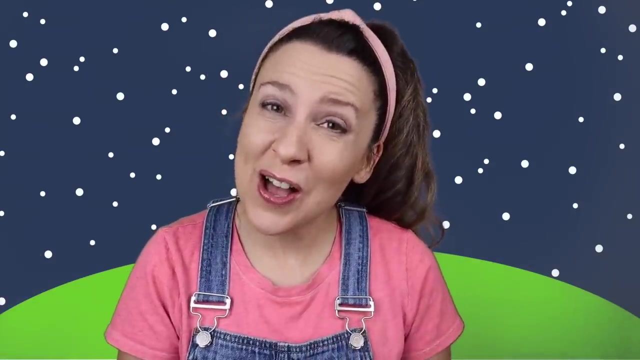 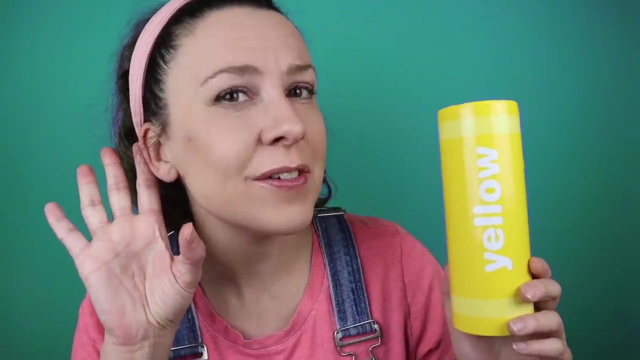 Like a diamond in the sky. Twinkle, twinkle, little star. How I wonder what you are. Yay, Wow, Great job. Quack quack, Quack, quack, quack. What was that sound? Did you hear that? 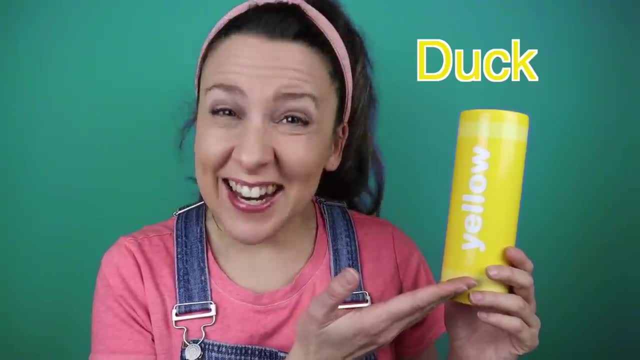 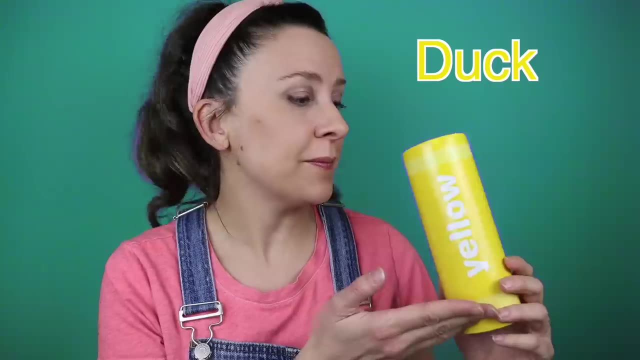 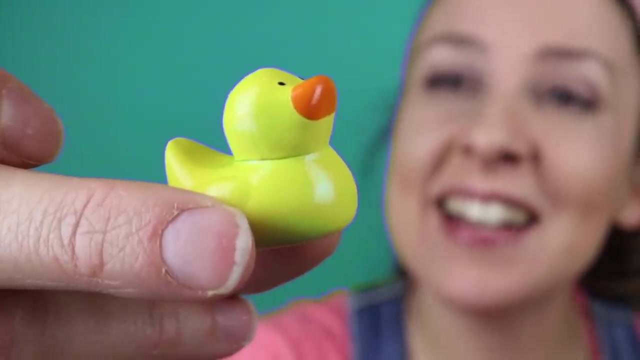 There must be a duck inside of the yellow crayon, Because we hear a quack. Oh wow, It's a little duck, So cute, A little tiny duck, Quack, quack, quack, Quack, quack, quack. 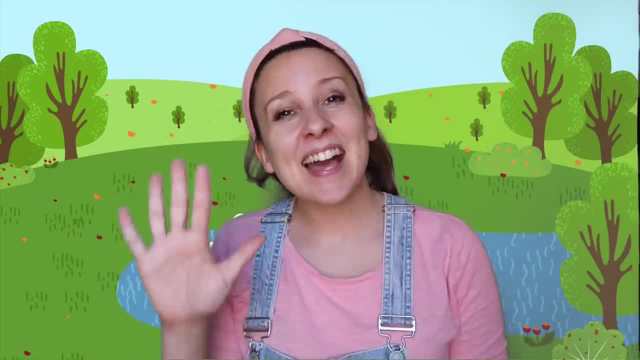 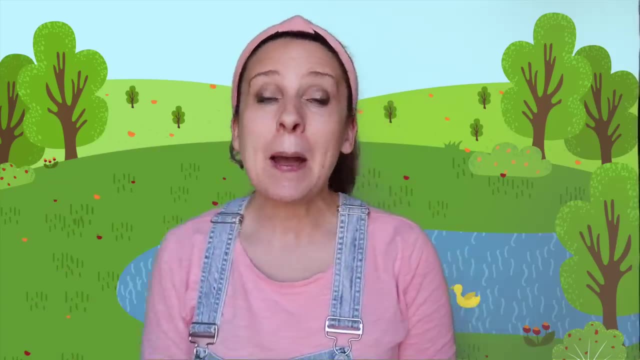 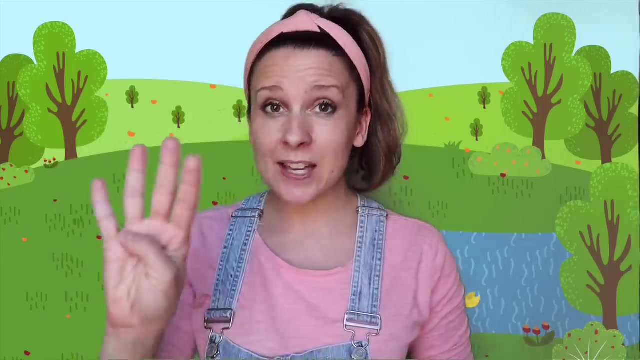 quase a duck. Quack, quack, quack, quack. What was that Little duck found a quack. How good it is, How cool, You know. quack, quack, quack. Wait, What is quack quack? 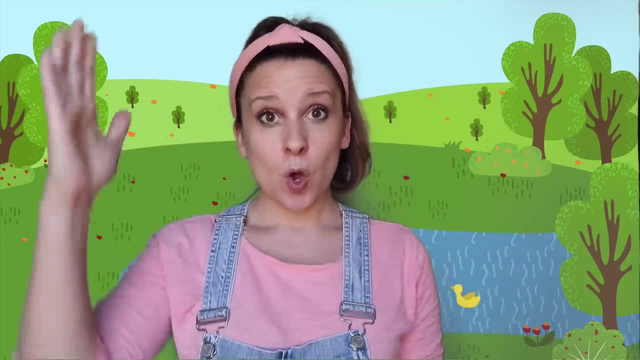 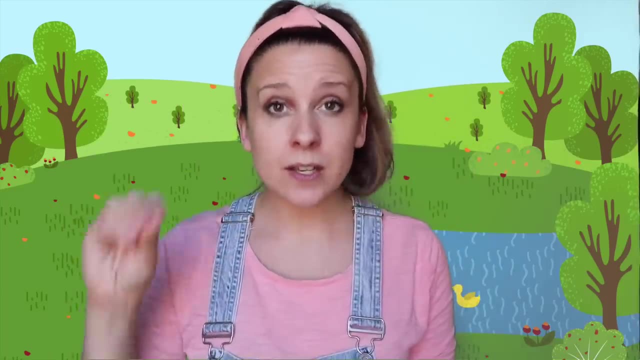 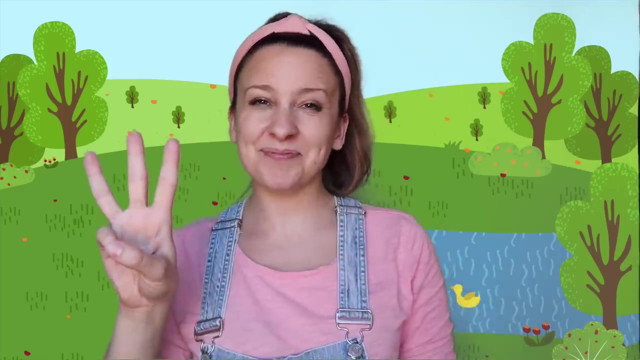 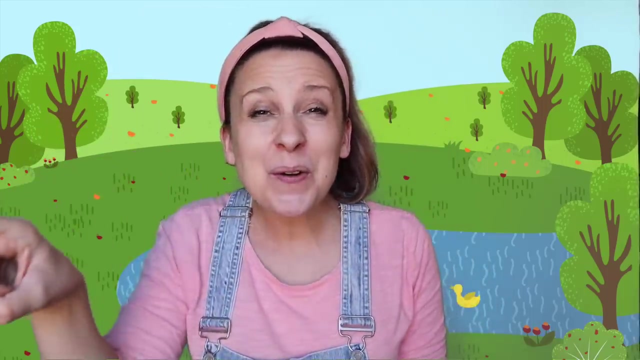 One explicit quack. Wait, Quack, quack, quack. What is quack quack away? mother duck said quack quack, quack quack. but only three little ducks came back. one, two, three, three little ducks went out one day, over the hill and far away. mother duck said: quack, quack, quack. 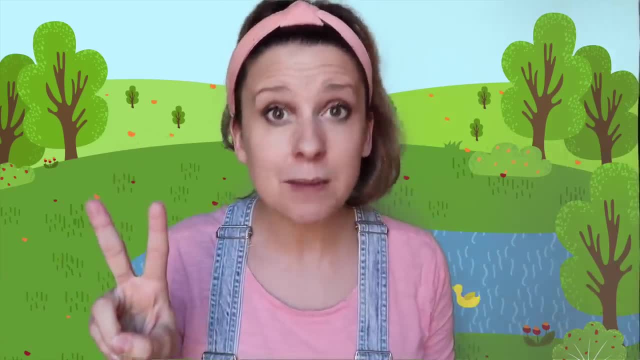 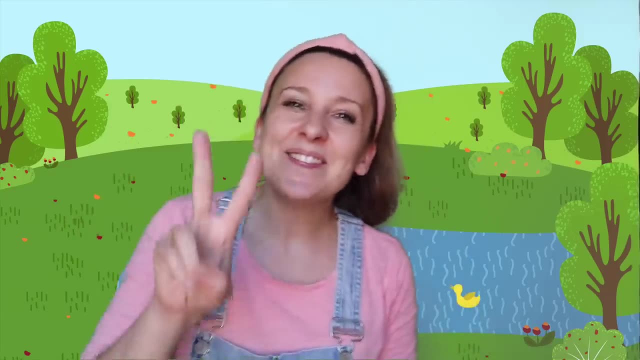 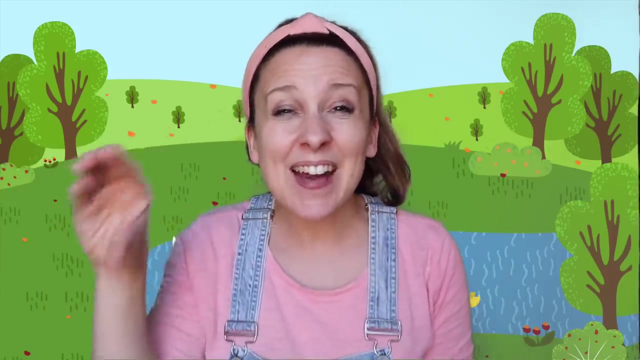 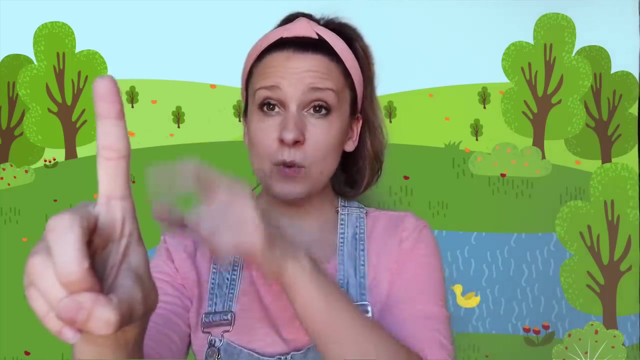 quack, but only two little ducks came back. one, two, two little ducks went out one day, over the hill and far away, mother duck said quack quack, quack, quack, but only one little duck came back. can you show me one, just one, one finger. one little duck went out one day. 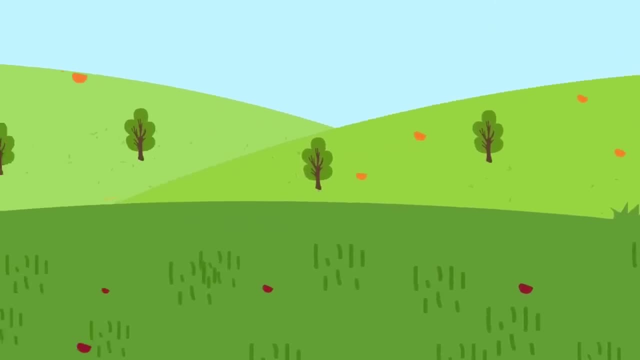 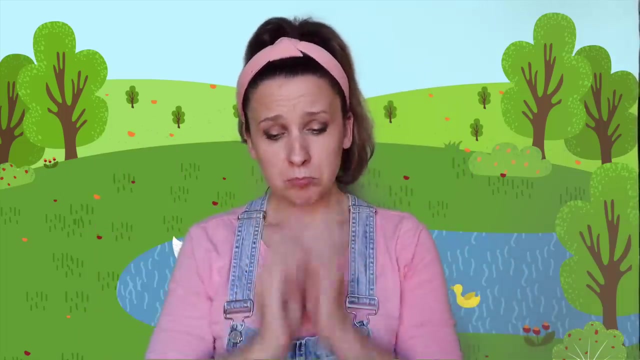 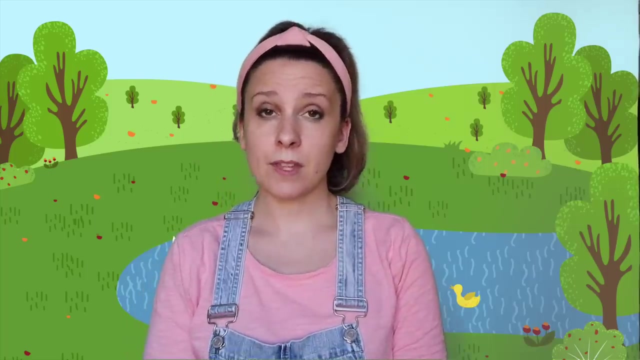 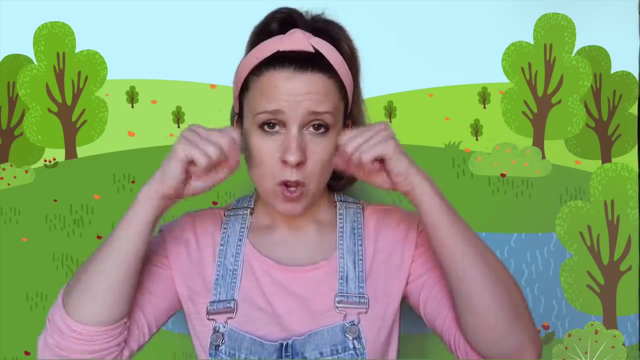 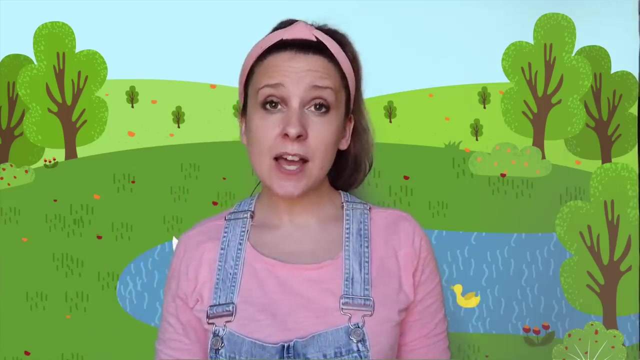 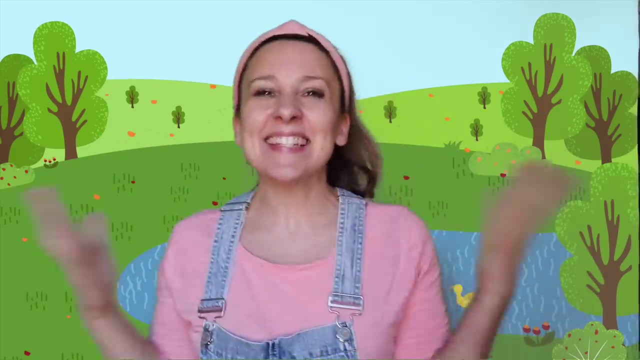 over the hill and far away, mother duck said quack, quack, quack, quack, but none of the five little ducks came back. mother duck is feeling very sad, sad mother duck went out one day, over the hill and far away, mother duck said quack, quack, quack, quack, and all of the five little ducks came back. 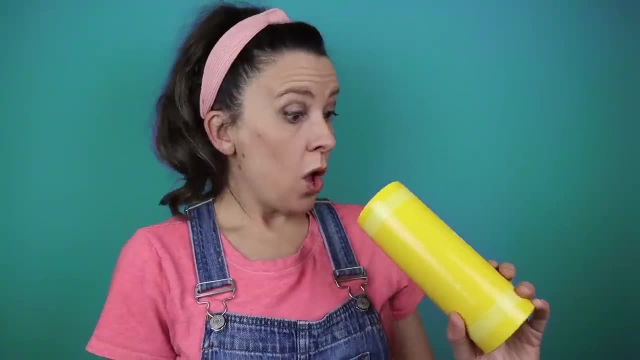 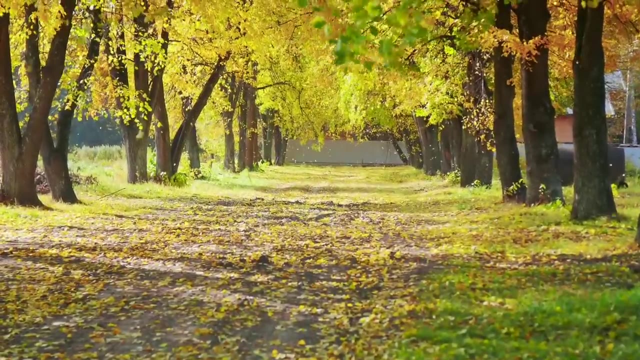 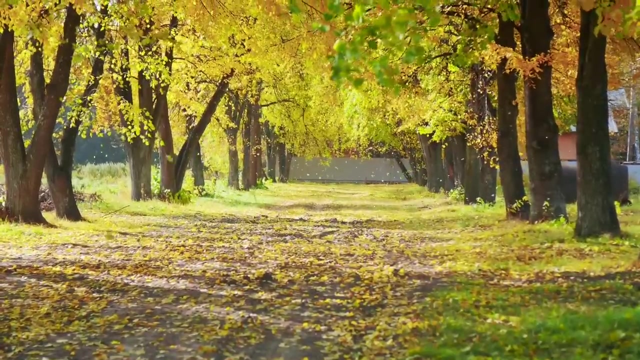 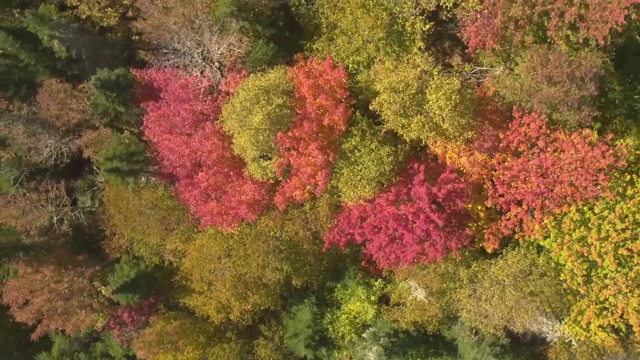 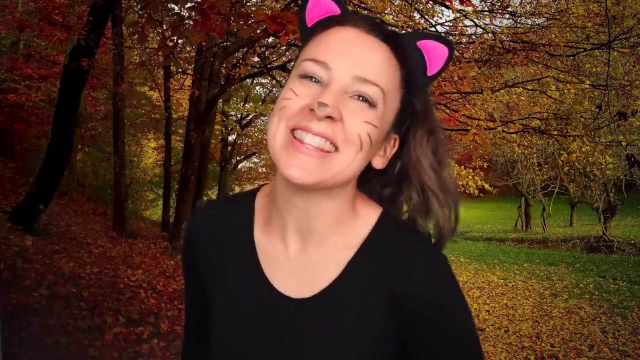 the duck found its mama. oh wow, it's a little yellow leaf. how beautiful. in the fall, the leaves change colors. they change from green to yellow and red and orange and brown. It's so beautiful. For the next song, get out some scarves or dish towels or even clothes and we'll pretend they're leaves. The leaves are. 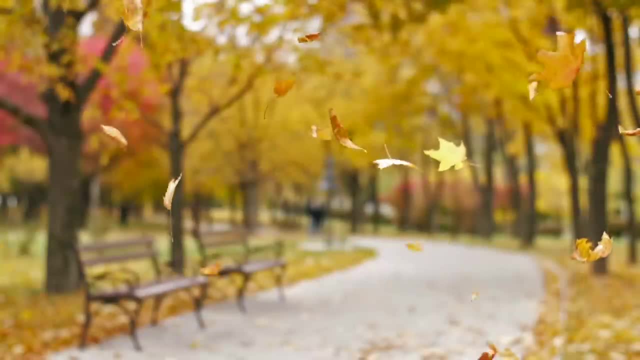 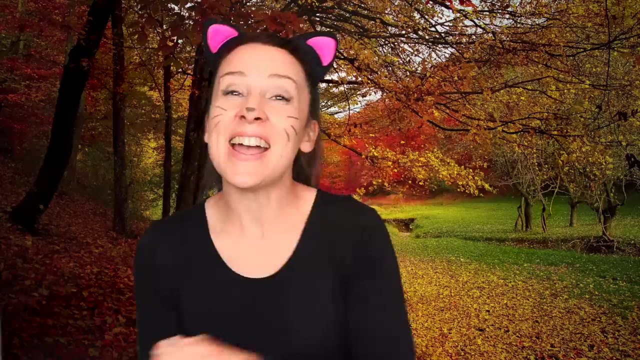 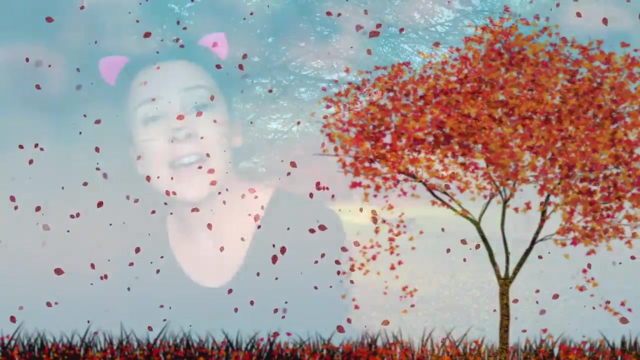 falling down. The leaves are falling down. Down, down to the ground. The leaves are falling down. Good job. Now let's pretend they're blowing around. okay, They're blowing in the wind. The leaves are blowing all around. They're blowing all around, Blowing up and blowing. 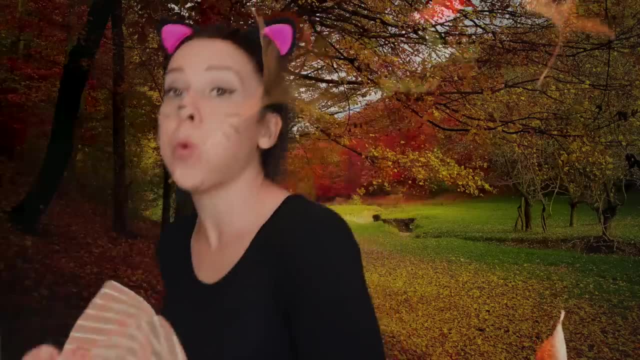 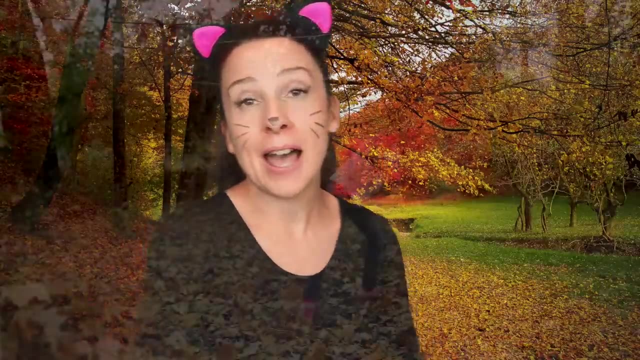 down and blowing all around. Wow, good job. Now let's rake them. We're gonna rake them in a pile. We'll rake them in a pile. Rake the leaves, rake the leaves. We'll rake them into a pile. 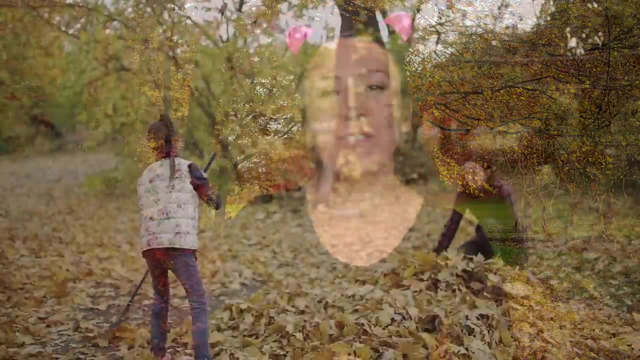 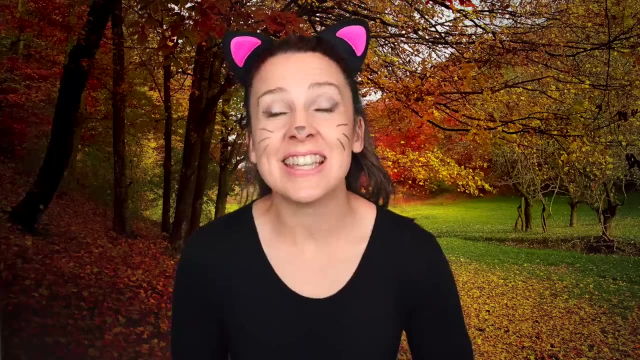 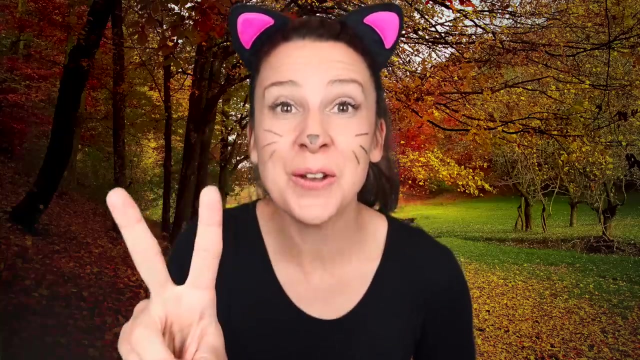 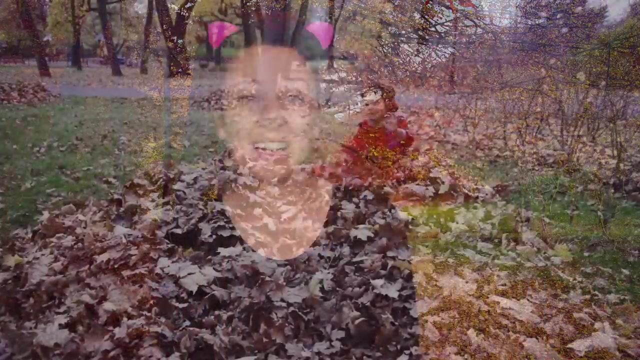 Oh, rake your leaves into a big pile. What should we do now that the leaves are in a pile? We're gonna jump into the leaves. We're gonna jump into the leaves When I count to three. we're gonna jump into the leaves. One, two, three. We jumped into the leaves, Yay. 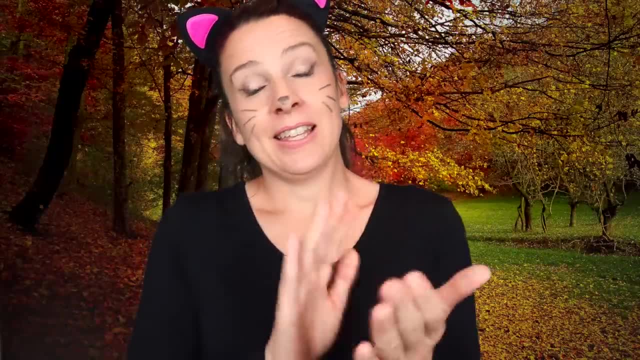 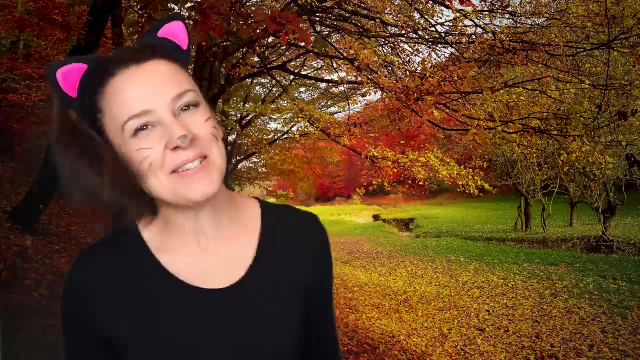 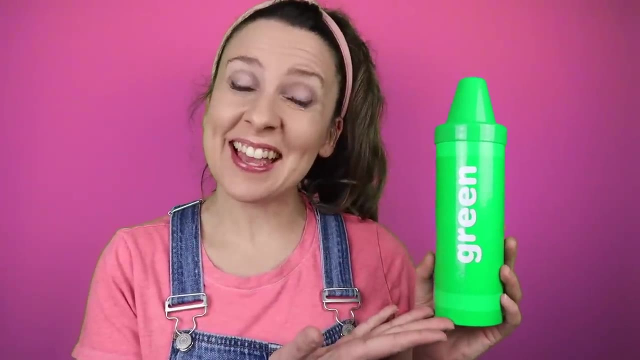 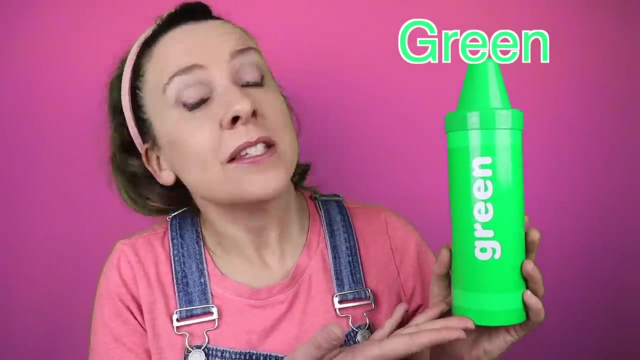 good job. When I was a little girl, I used to like to rake our leaves in my yard into a pile and then I'd jump in them and play in them. It was so much fun. Great job. Do you know what color this is? Yeah, it's green. Good job. Say open and it will open. Open, Wow, it's. 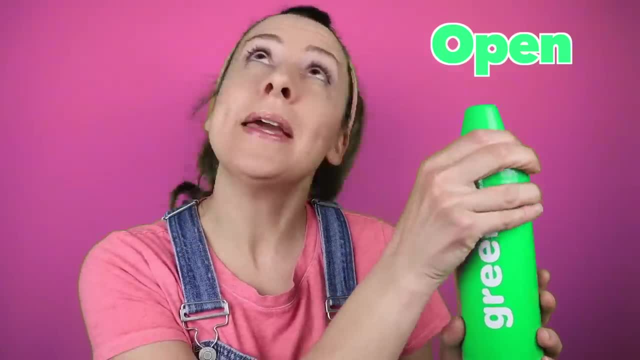 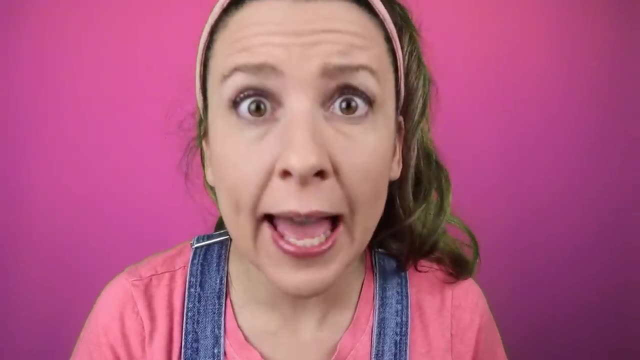 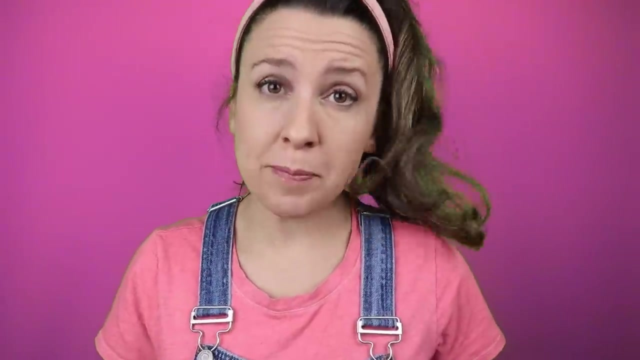 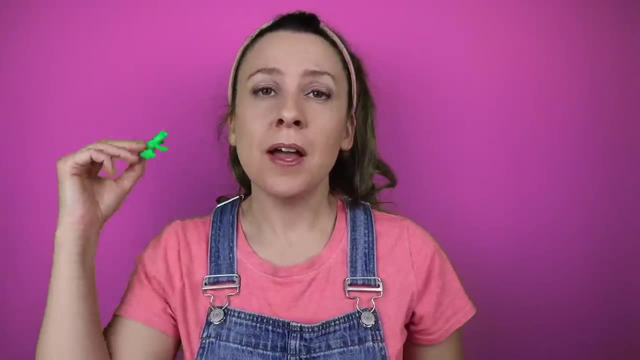 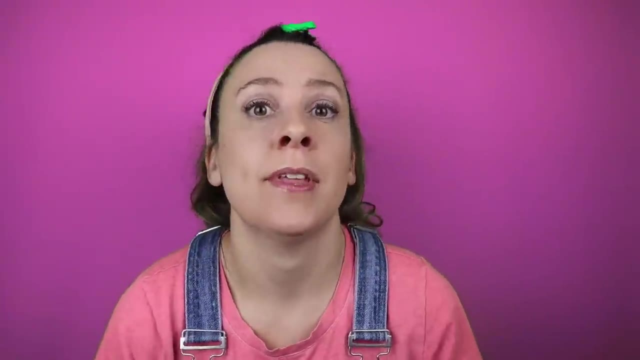 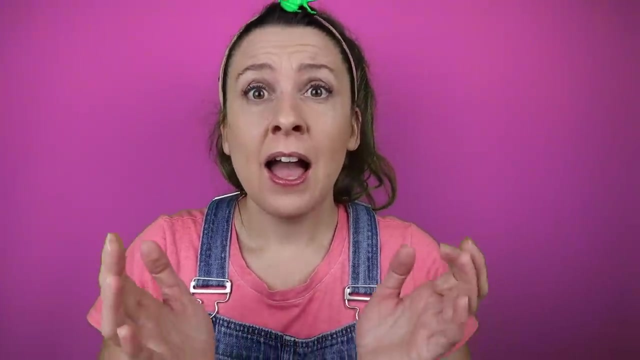 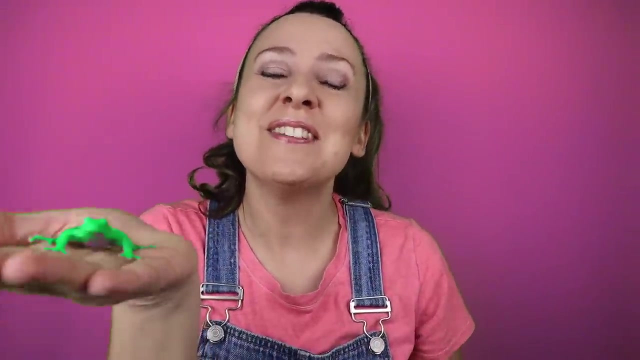 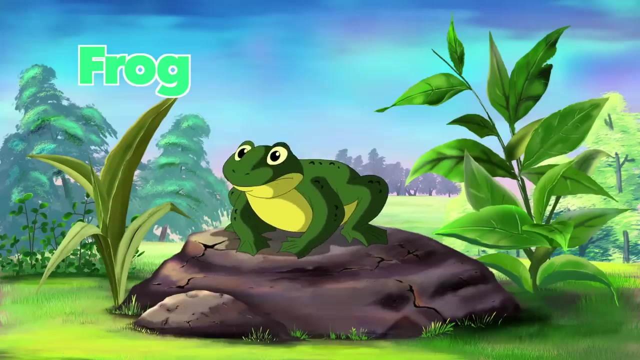 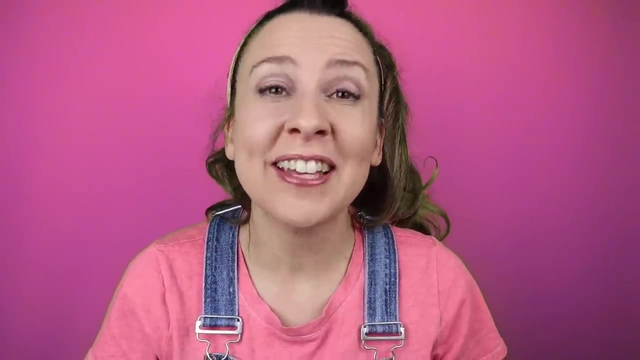 hop, hop, hop, hop, hop, hop. A what? Hop, hop, hop, hop? Where did it go? I don't know, I don't know. Hmm, Do you see it anywhere? see it anywhere? Ah, Ah, Ah, Ah, Ah-choo. Oh, the frog was on my head, It's a little green frog. Wow, Frogs love to hop, hop, hop, hop. I know a great song about a frog, Can you? 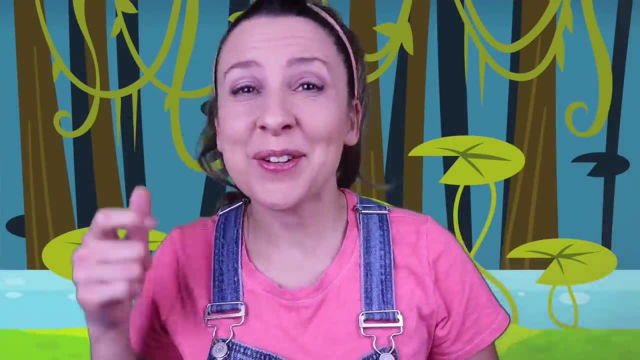 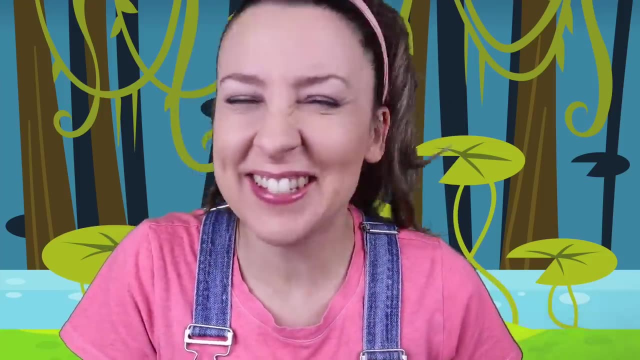 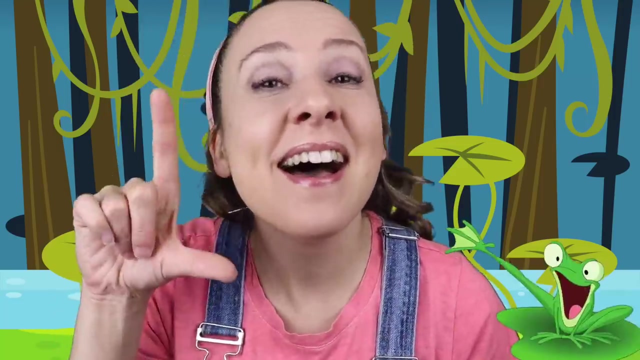 sing it with me. What does a frog say? Ribbit, ribbit, ribbit, ribbit, ribbit. In this song they say something else. It's so silly. Mmm-ah went the little green frog. one day, Mmm-ah. 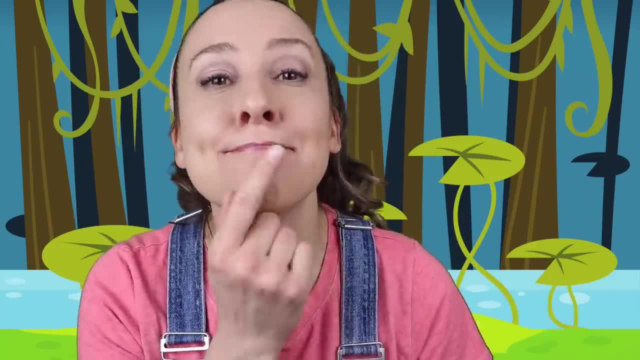 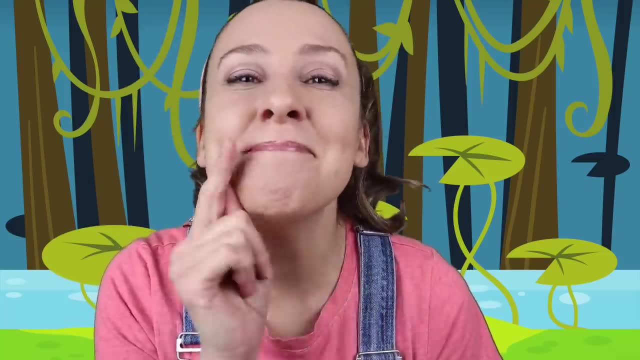 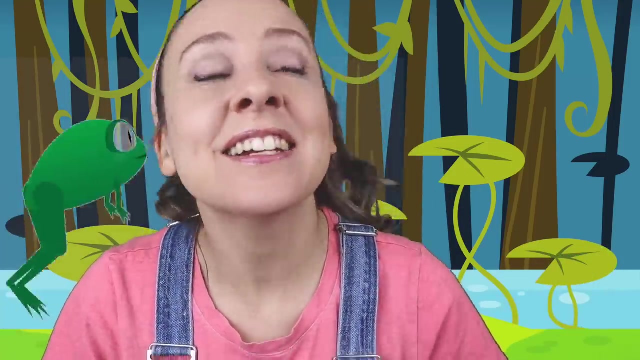 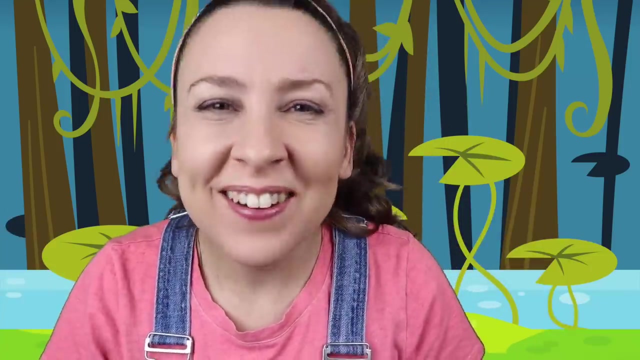 went the little green frog, Mmm-ah, went the little green frog one day And they all went mmm-mmm-ah. But we know frogs go la-dee-da-dee-da, la-dee-da-dee-da, la-dee-da-dee-da, We know frogs go la-dee-da-dee-da. 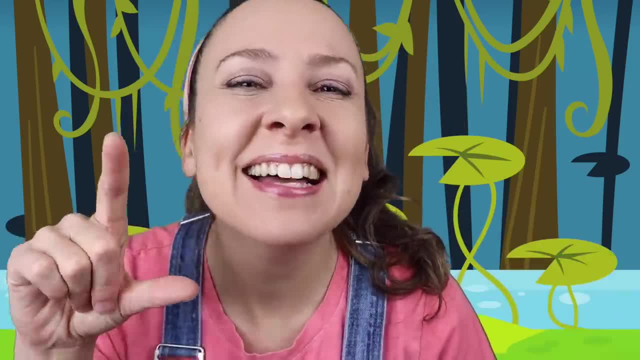 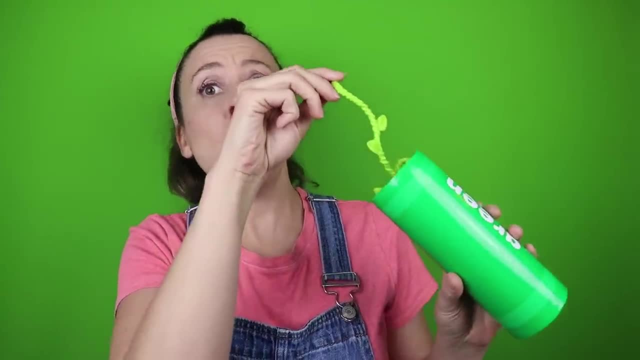 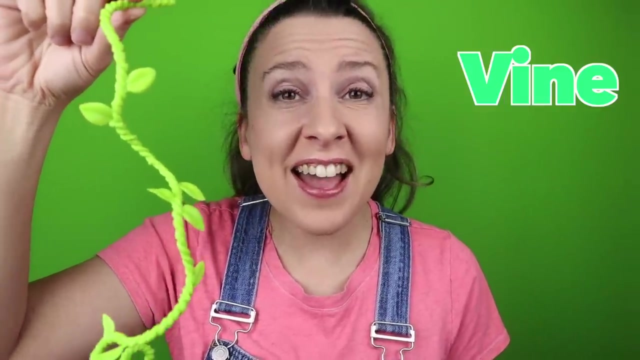 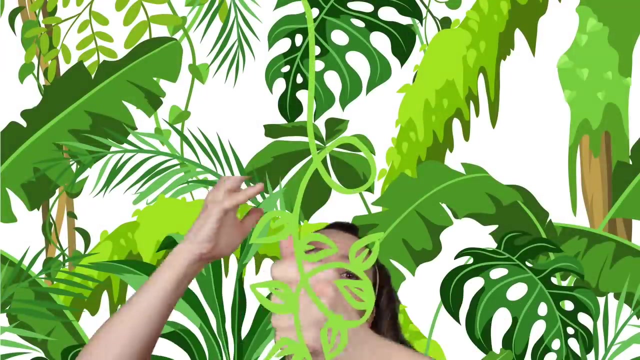 They don't go. mmm-mmm-ah, That was so silly, Good job. Let's see what else is inside. Whoa, Whoa, Whoa, Whoa, It's a green frog Vine. Wow, Can you pretend to climb up a vine? Climbing up a big vine, Up Up, Wow. 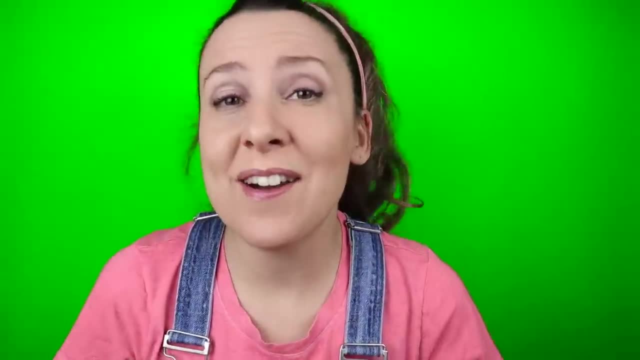 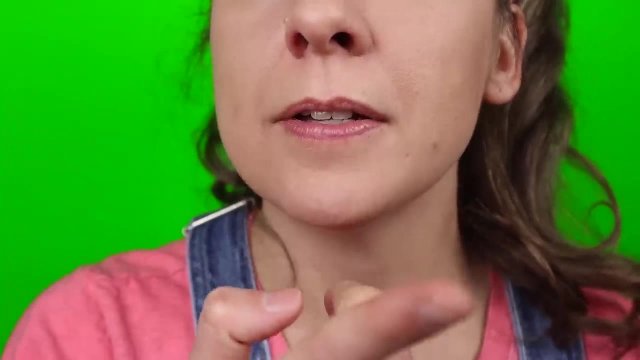 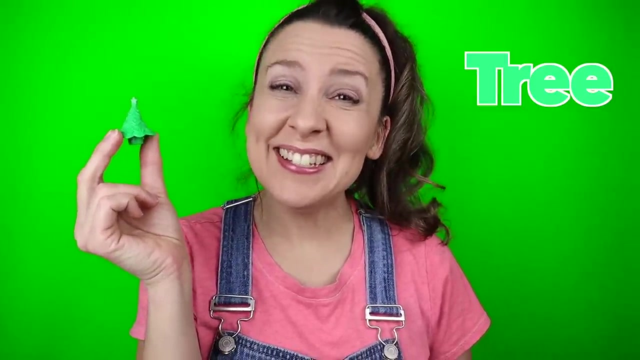 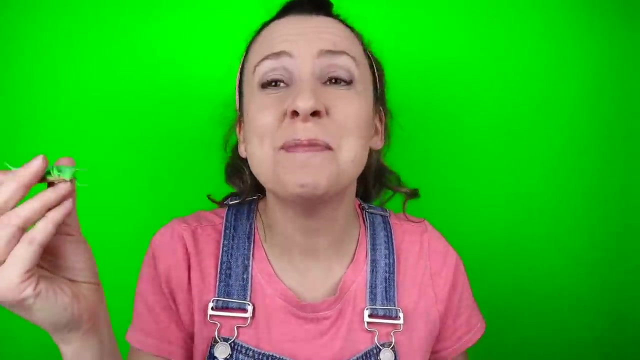 You're so strong, Up Up. Wow, It's a little tree. Good job, Great, Good job. Up, Yeah, Up, A little tree, hop, hop, hop. another thing that hops: It's a little grasshopper. 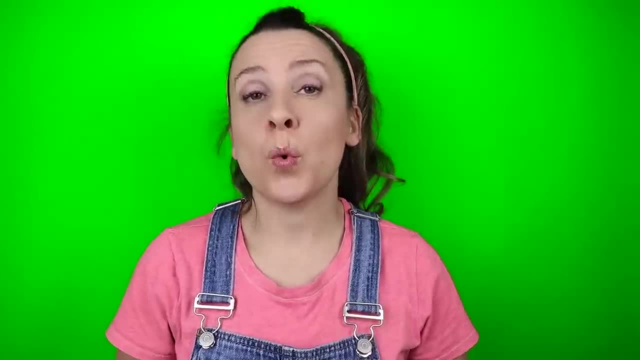 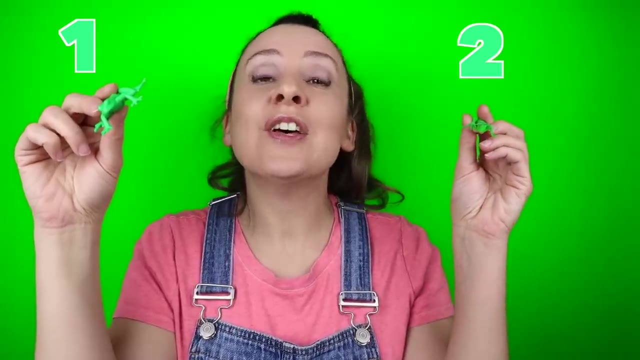 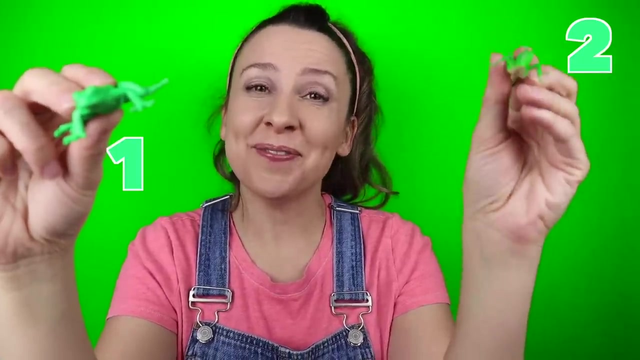 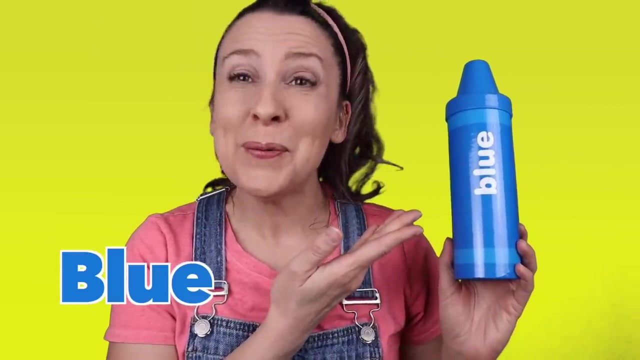 How many things did we find that hop One, the little frog and two the little grasshopper. Two things that hop one, two, two things. Our next color is blue. wow, Blue begins with B. Can you do a B sound? 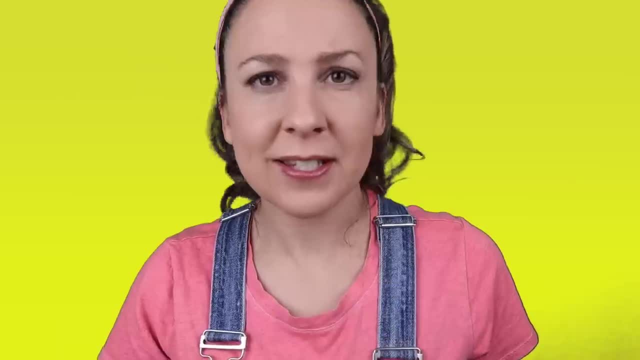 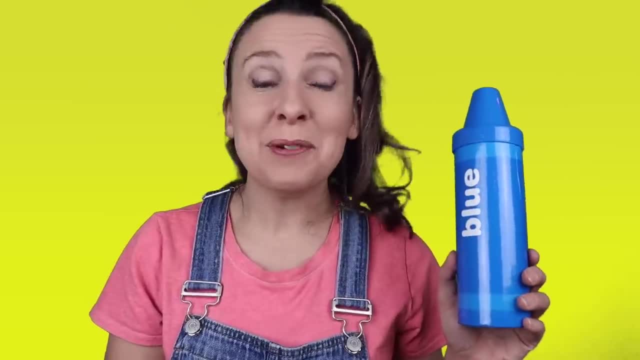 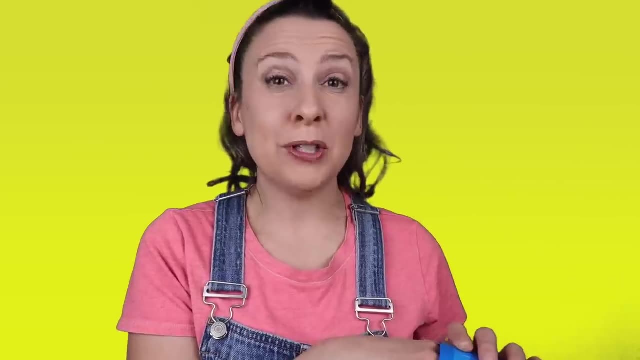 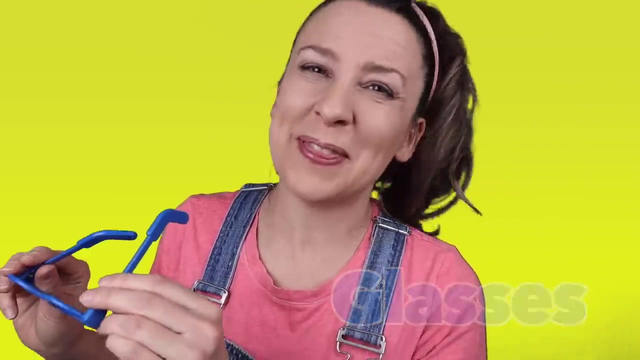 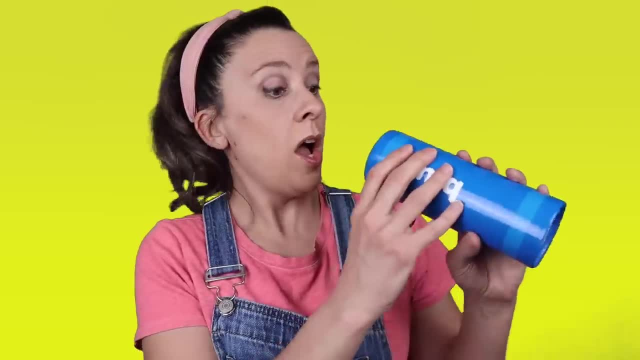 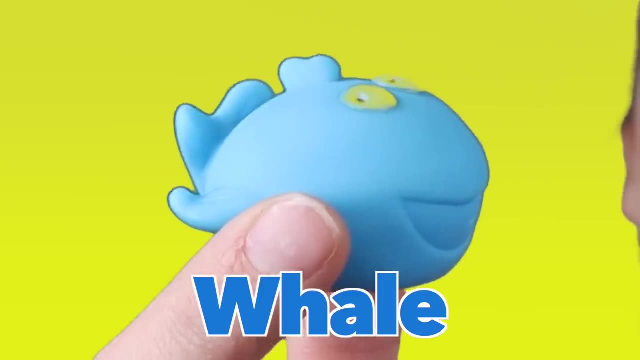 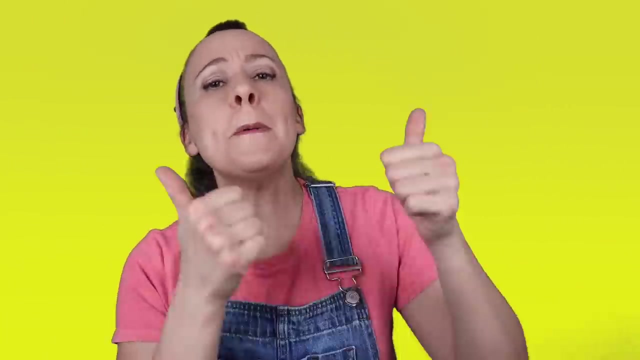 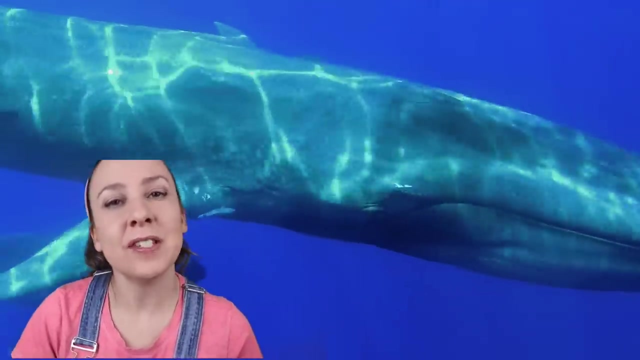 Blue glasses. whoa, it's a blue whale. wow, The blue whale is the biggest animal in the world. It's so big. Whale begins with W. Can you do the W sound? Wuh, wuh, wuh. 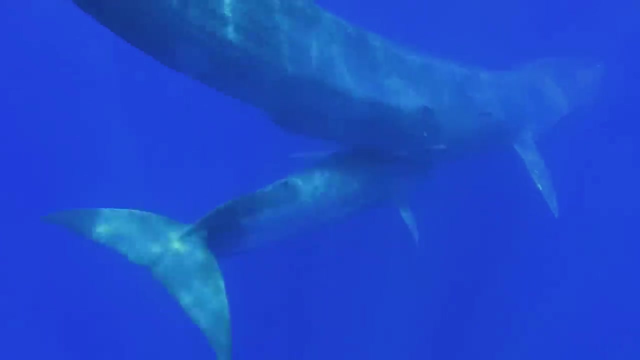 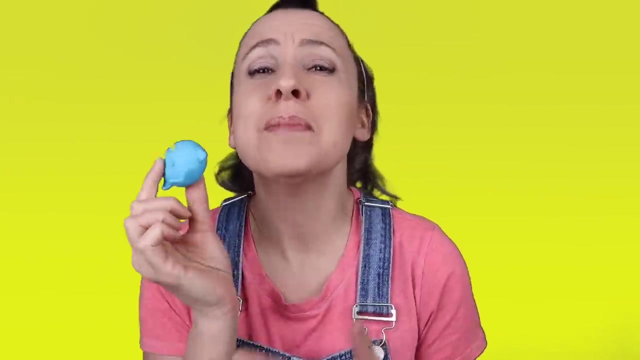 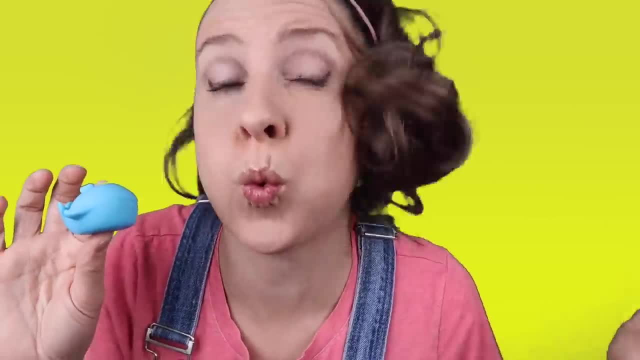 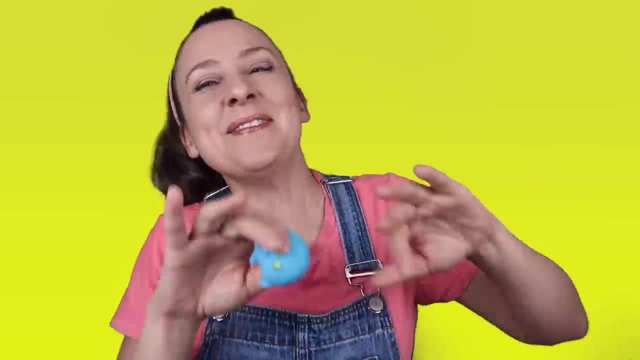 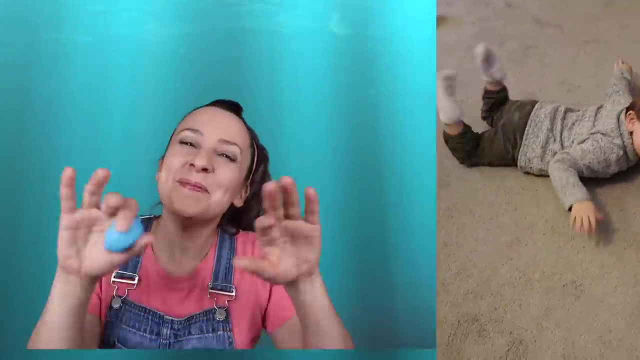 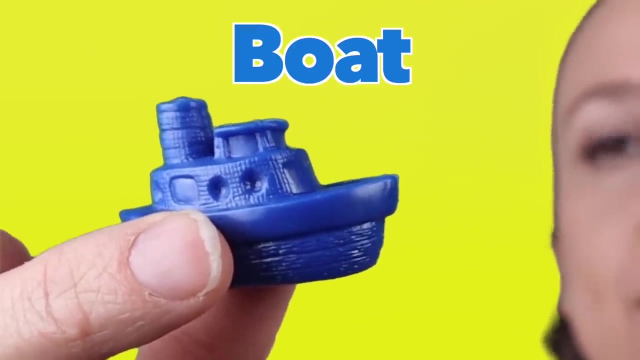 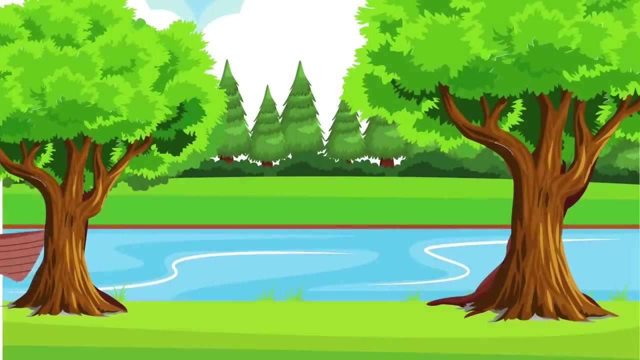 Good job, Swim, swim, Can you swim around the room? Swim, Wow, a blue boat, Blue and boat both start with B. Blue boat Row row. row your boat Gently down the stream, Merrily, merrily, merrily, merrily. life is but a dream. 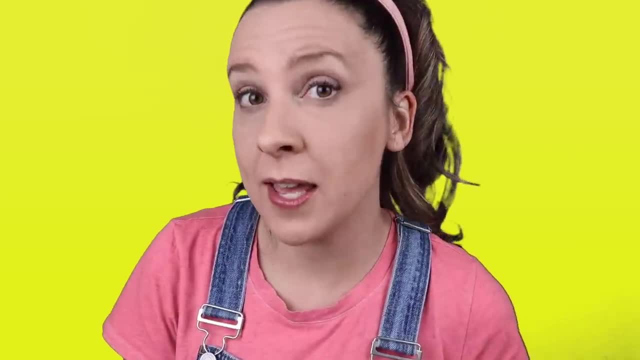 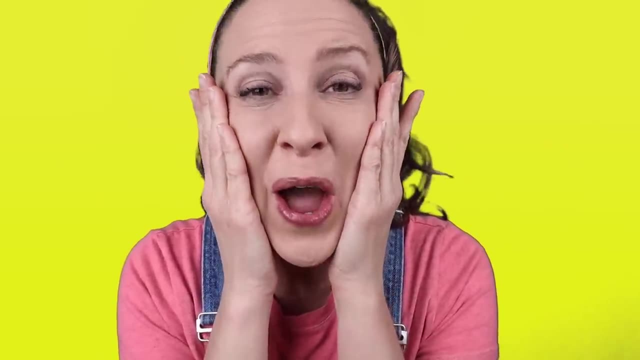 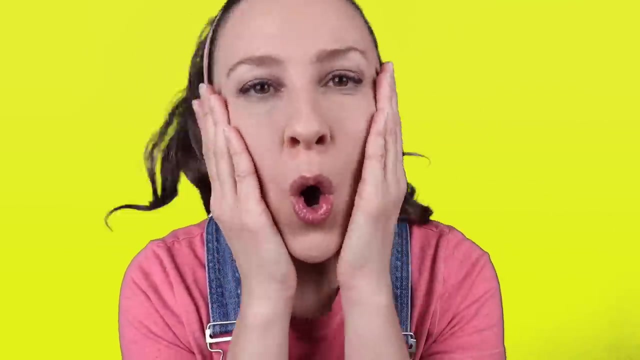 That was so fun. Now you fill in the words and we'll pretend to see a crocodile. Oh no, Uh, oh. Can you say that? Uh, oh, uh, oh, uh oh, Row, row, row your boat. 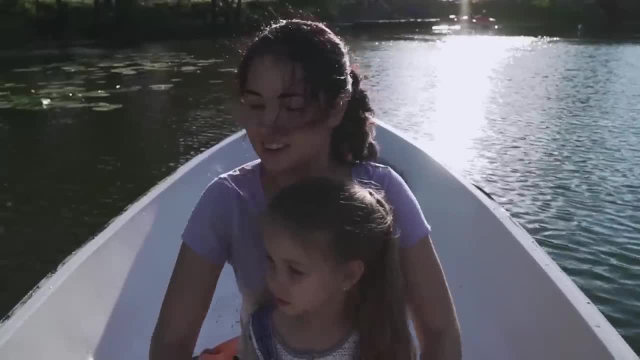 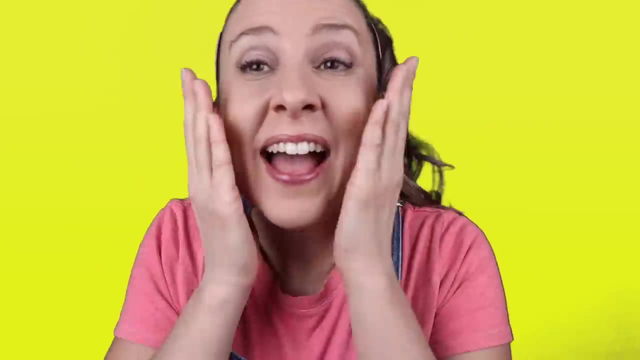 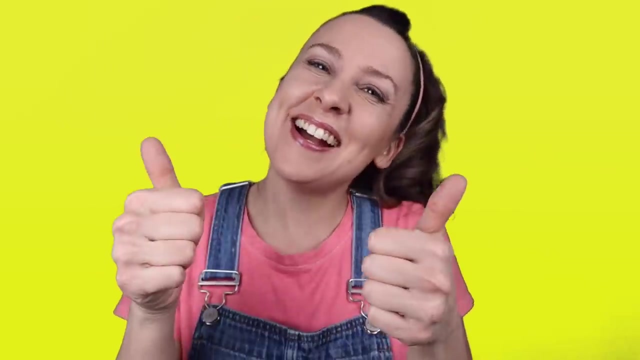 Row row, row your boat Row row, row your boat Gently down the stream. If you see a crocodile, don't forget to scream: Ahh, Can you do that? Ahh, Good job, A blue bear. 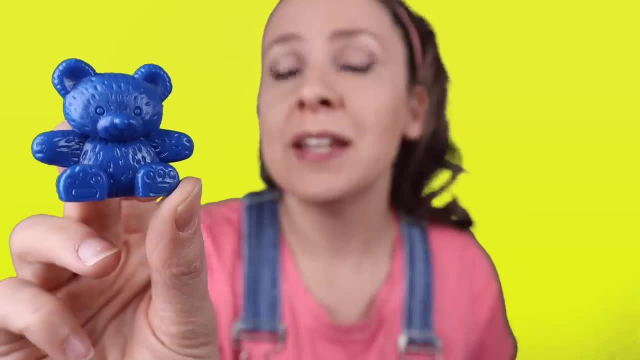 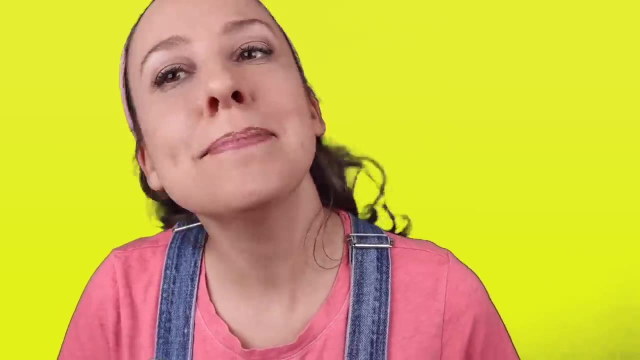 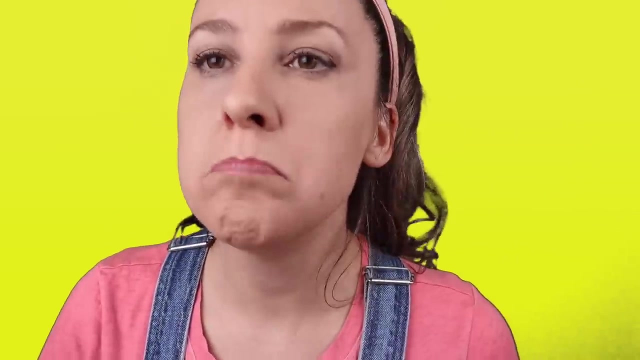 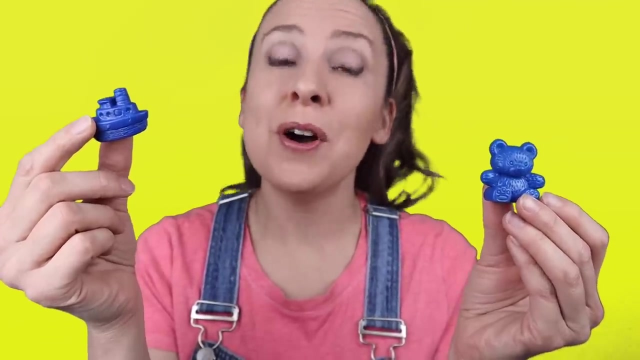 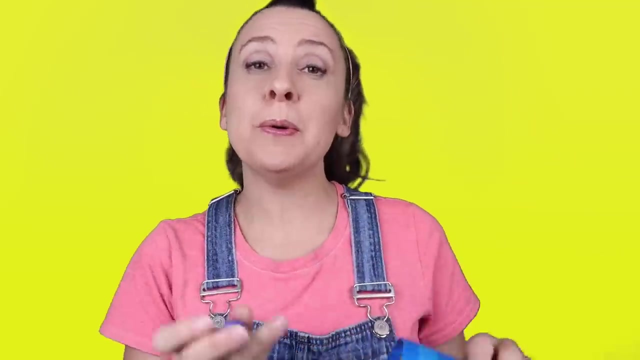 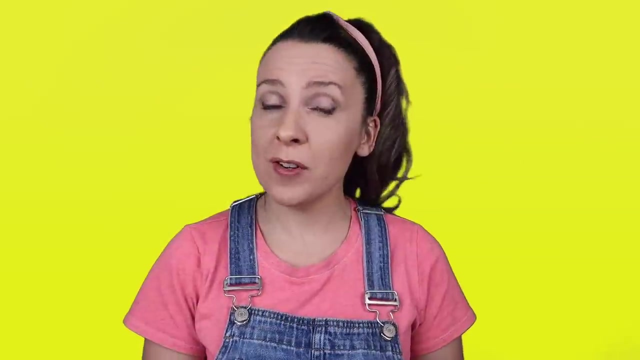 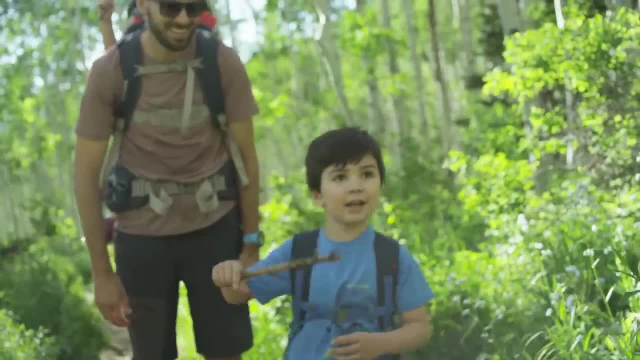 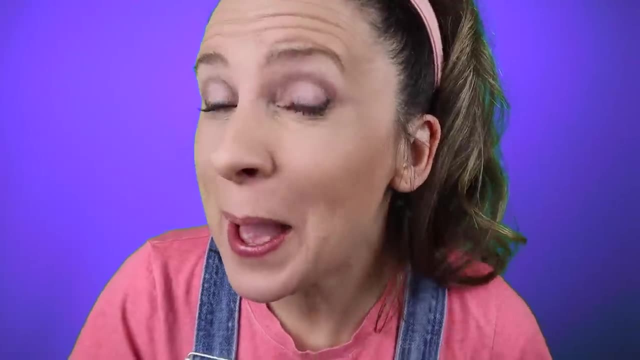 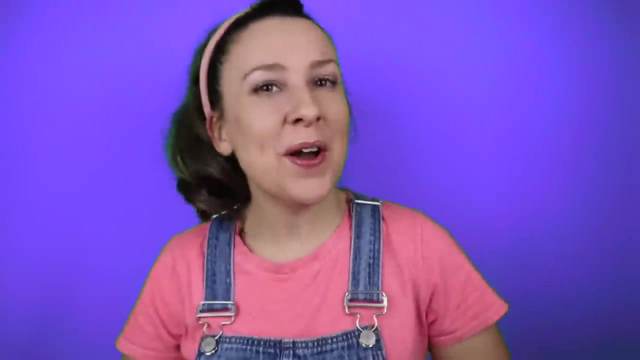 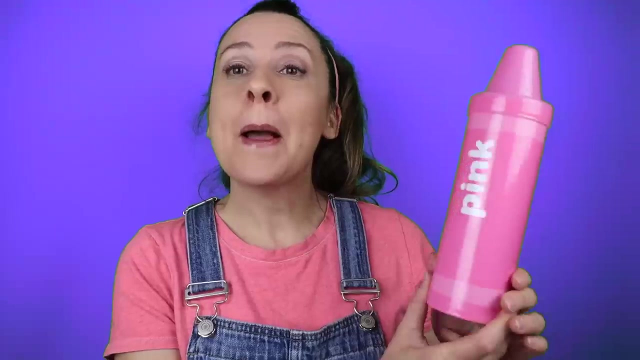 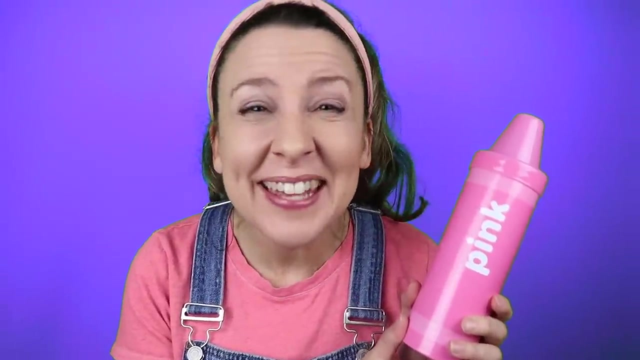 a backpack. B-b-backpack also starts with the letter B: B-b-b-backpack. Guess what My favorite color is next? It's the color of my shirt and the color of my headband. What color is that? Hmm, Yeah, it's pink. Good job, Say open and it will open. Open. 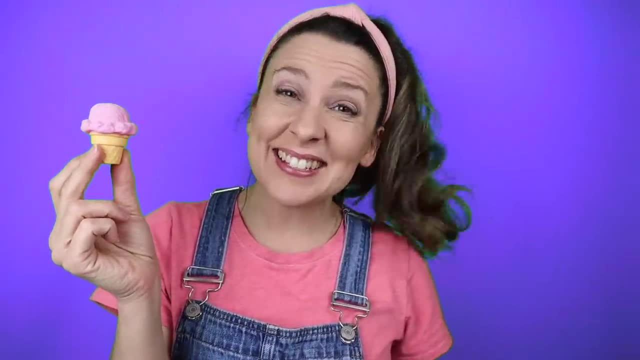 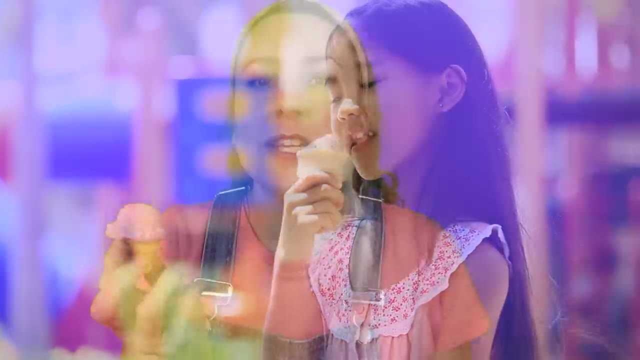 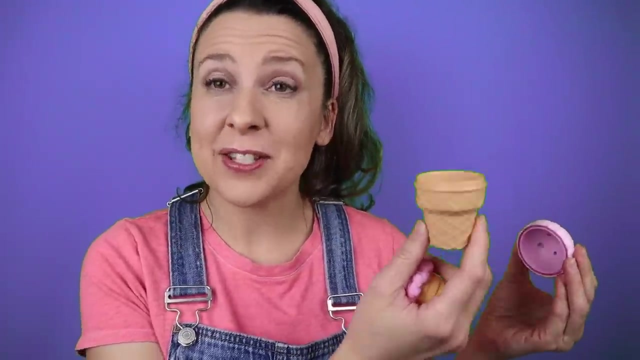 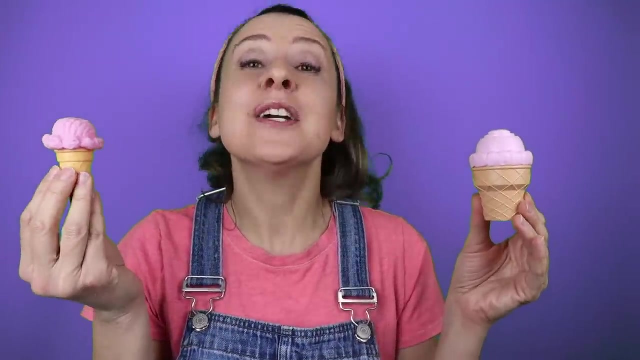 It's a pink ice cream. Aww, I love ice cream. Let's pretend to lick it. Just pretend Ice cream is cool. Cold- That's the sign for cold. I have another ice cream. Put it on the cone Now I have. 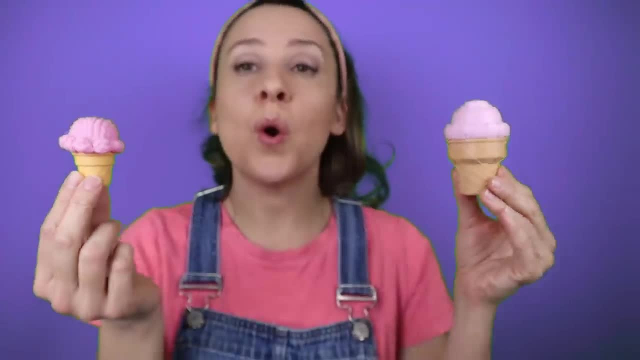 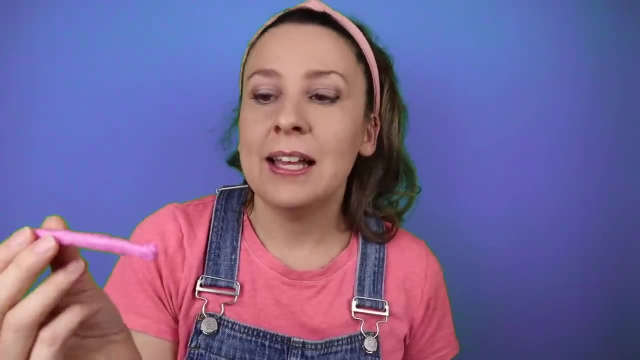 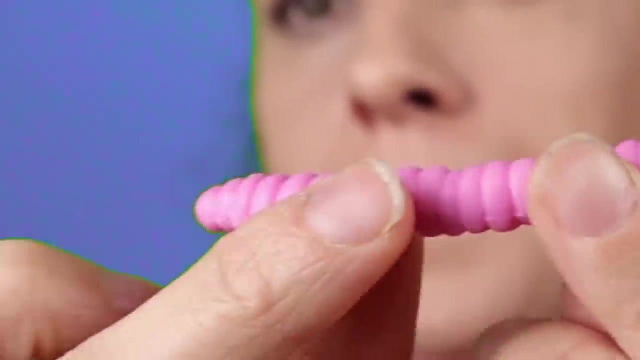 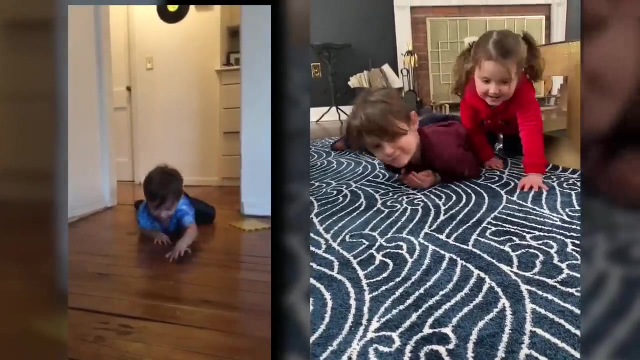 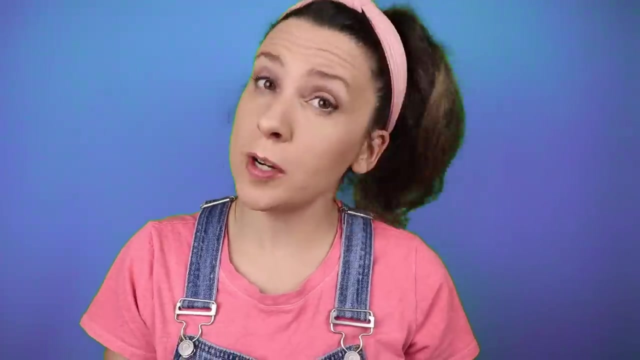 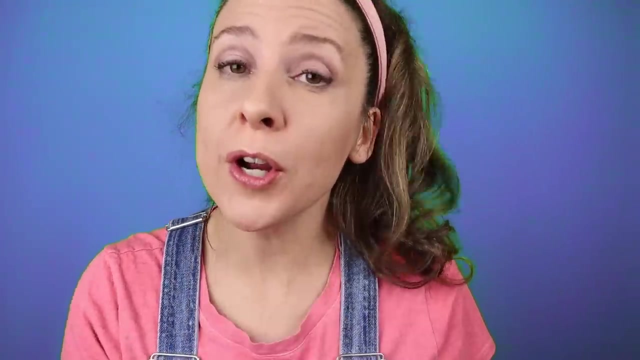 two ice creams, One, two. Oh, it's a slimy, long pink worm. I'm a worm. Can you crawl around your room like a worm on your tummy? That's so silly. Worm starts with our W sound. Can you do it? W-w-w-w-w-w-worm. Good job. Oink, oink. 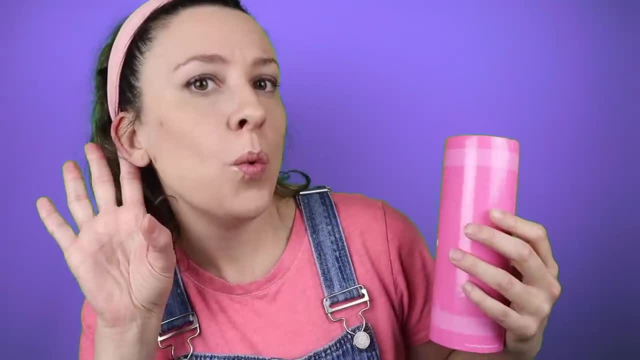 Did you hear that Oink oink W-w-w-w-w-worm? Good job Oink oink. Did you hear that Oink oink W-w-w-w-w-w-worm, Good job Oink oink. Did you hear that Oink oink W-w-w-w-w-worm. 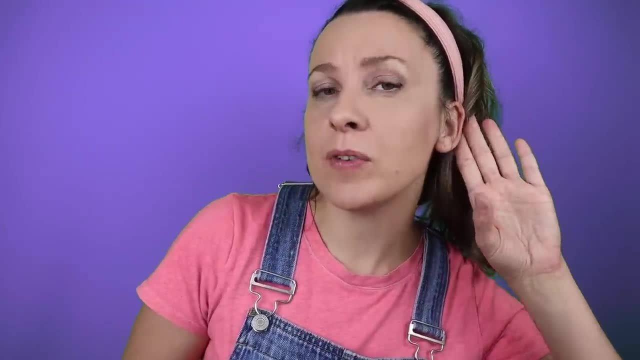 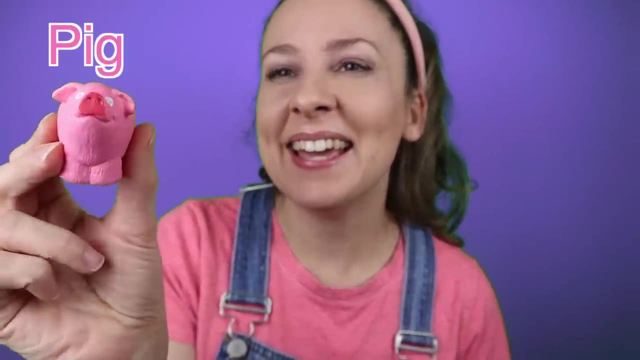 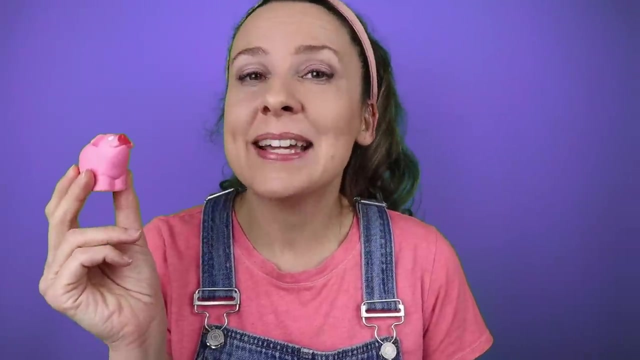 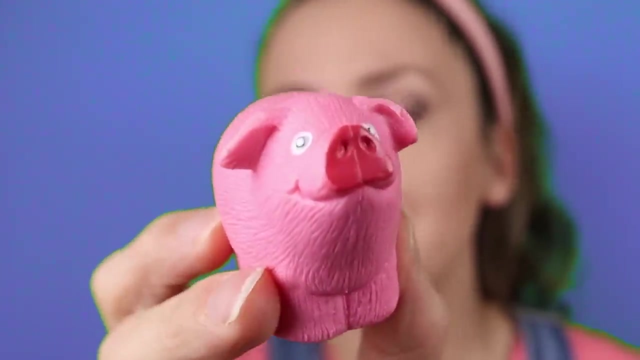 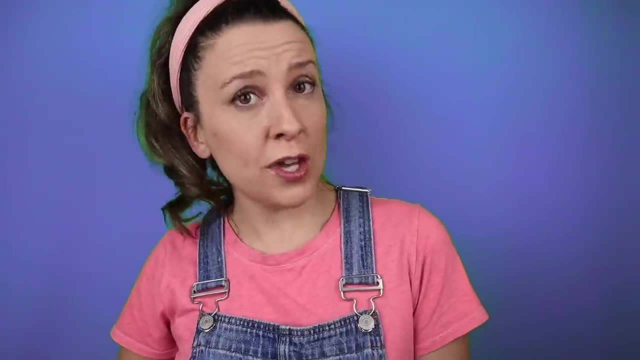 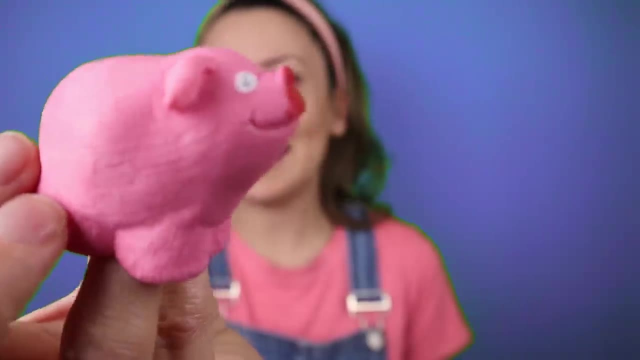 Mwah Mwah, Mwah, Mwah Mwah. Can you blow the pig? a kiss Mwah Mwah. Blow the pig, a kiss Mwah. Thank you for the kiss. 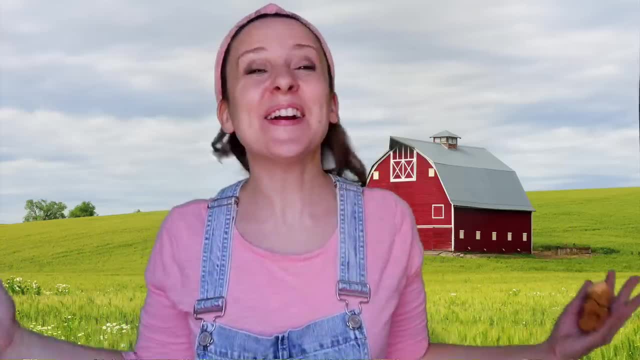 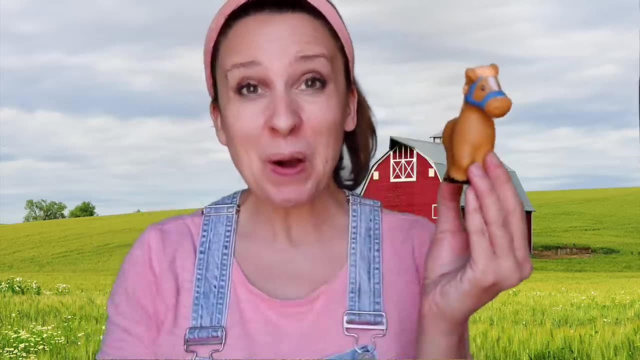 Let's sing: Old MacDonald Had a Farm. Old MacDonald had a farm E-I-E-I-O And on that farm he had a horse E-I-E-I-O With a neigh, neigh here and a neigh neigh there. Here a neigh, there, a neigh, everywhere a neigh. 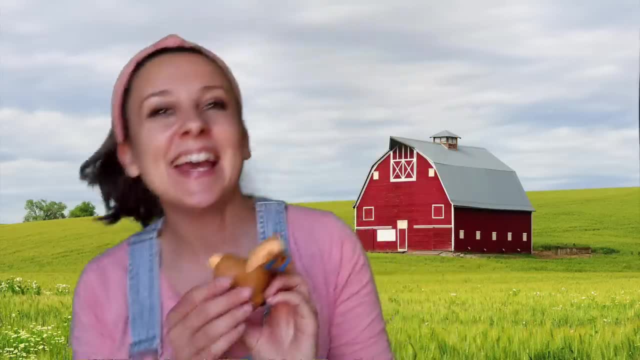 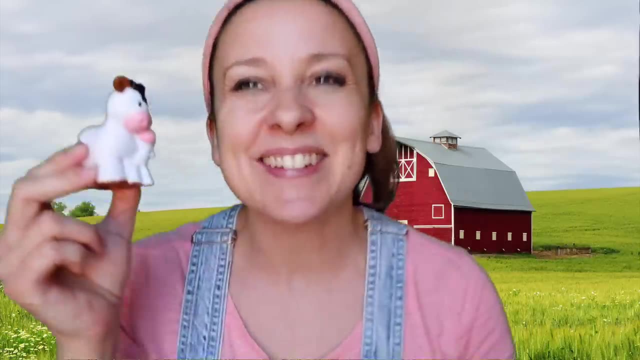 And on that farm he had a horse E-I-E-I-O. And on that farm he had a horse E-I-E-I-O. Old MacDonald had a farm E-I-E-I-O. I wonder what animal will be next. Old MacDonald had a farm E-I-E-I-O. 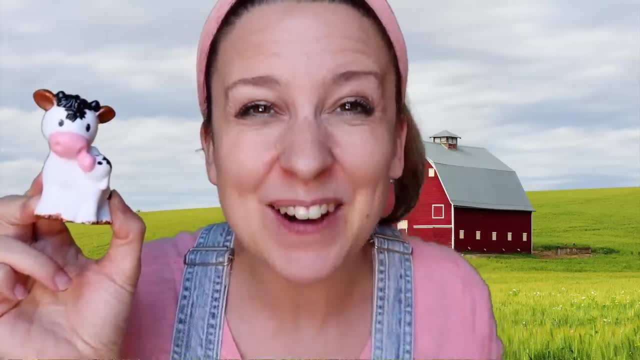 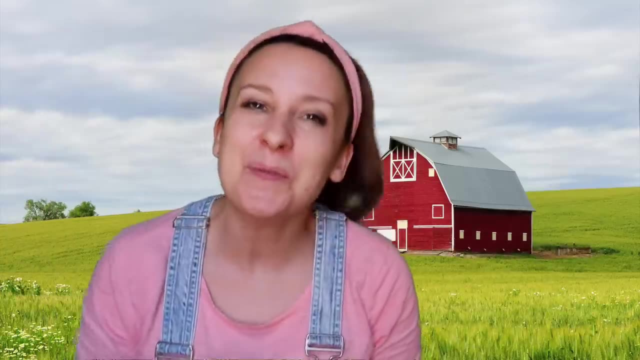 And on that farm he had a cow- E-I-E-I-O, With a moo moo here and a moo moo there. Here, a moo there, a moo, everywhere a moo moo. Old MacDonald had a farm E-I-E-I-O. 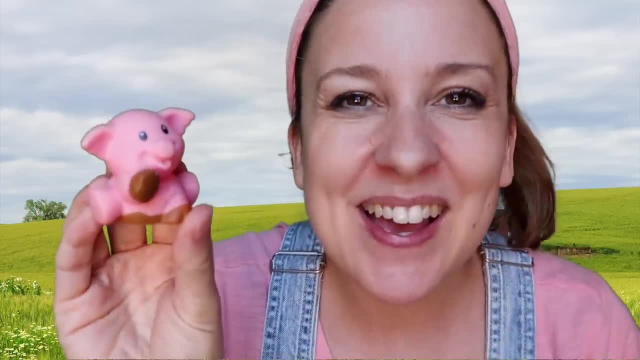 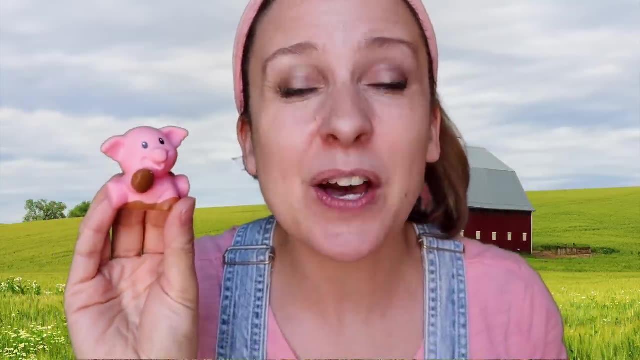 And on that farm he had a pig E-I-E-I-O With an oink oink here and an oink oink there. Here an oink, there an oink, everywhere an oink oink. Old MacDonald had a farm E-I-E-I-O. 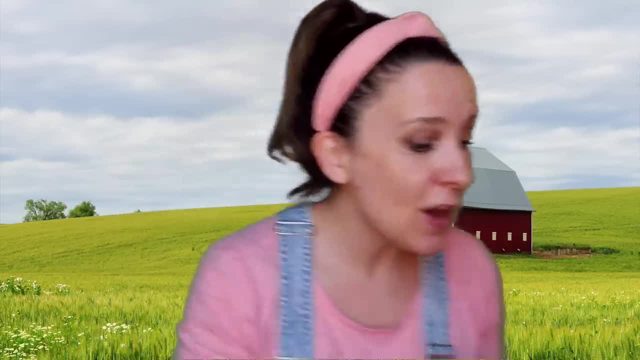 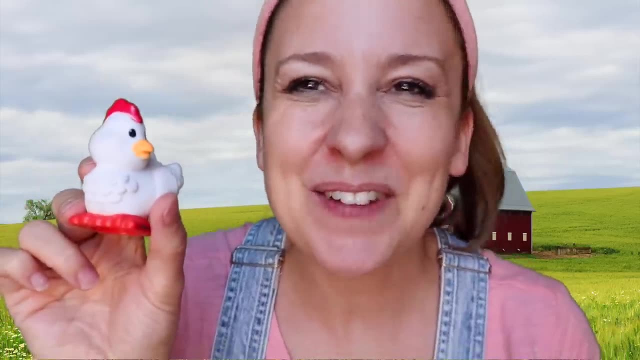 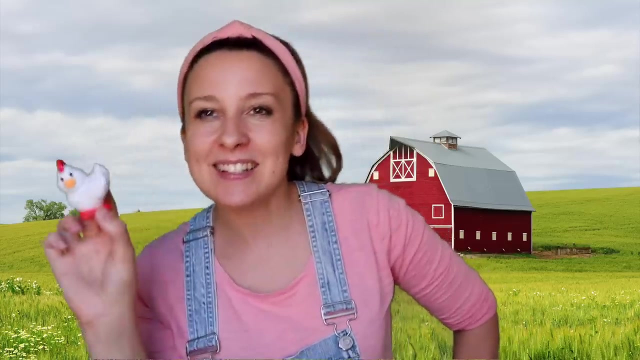 I hear a chicken. Old MacDonald had a farm E-I-E-I-O, And on that farm he had a cow E-I-E-I-O. And on that farm he had a pig E-I-E-I-O, And on that farm he had a chicken E-I-E-I-O. 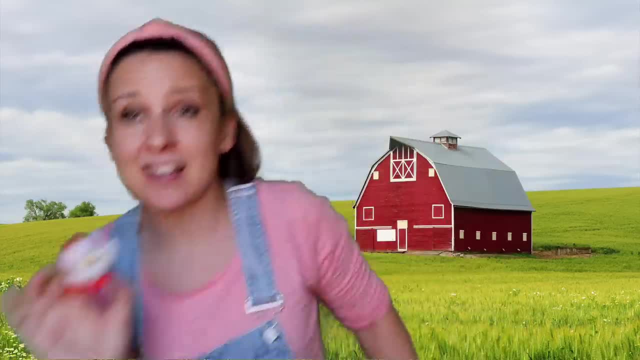 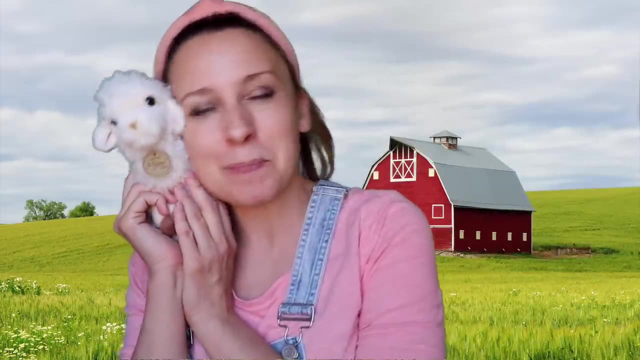 With a cluck cluck here and a cluck cluck there. Here a cluck, there a cluck, everywhere a cluck cluck. Old MacDonald had a farm E-I-E-I-O. Aww, how cute A little sheep. 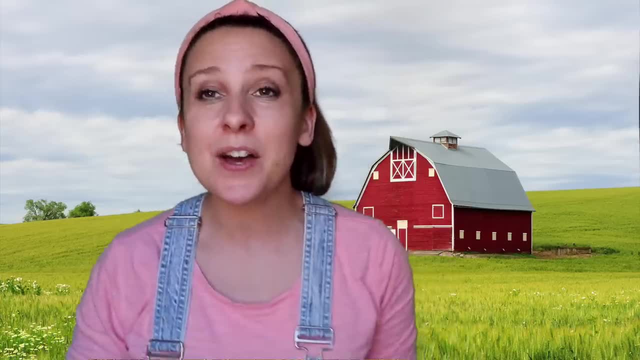 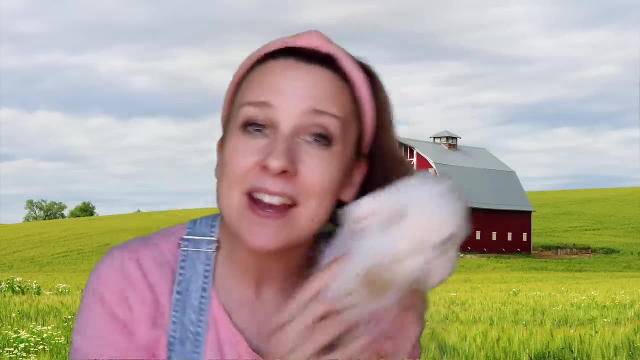 Old MacDonald had a farm E-I-E-I-O And on that farm he had a sheep E-I-E-I-O With a baa baa here and a baa baa there, Here, a baa there, a baa everywhere, a baa baa. 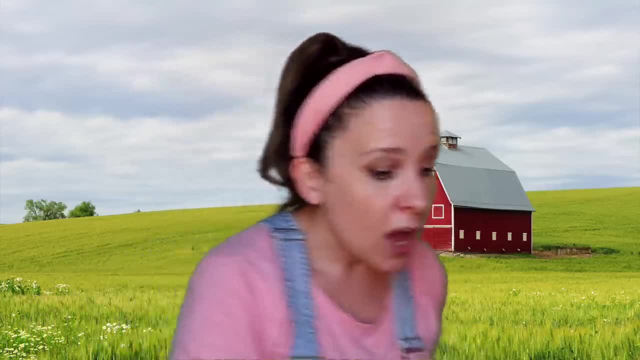 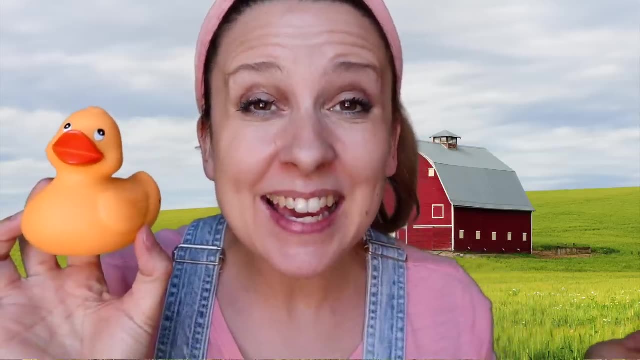 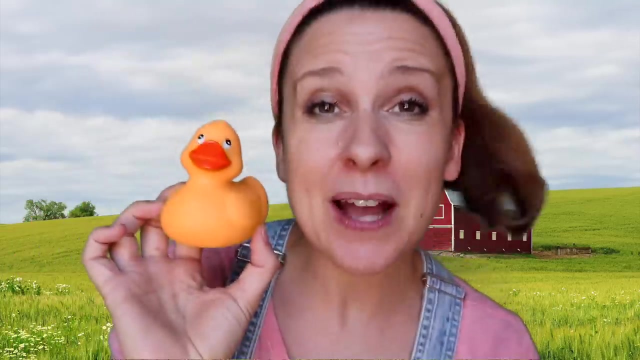 Old MacDonald had a farm E-I-E-I-O, Quack, quack- What says quack? Old MacDonald had a farm E-I-E-I-O And on that farm he had a duck E-I-E-I-O With a quack quack here and a quack quack there. 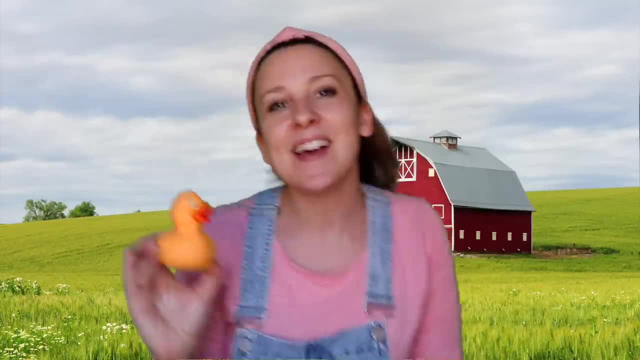 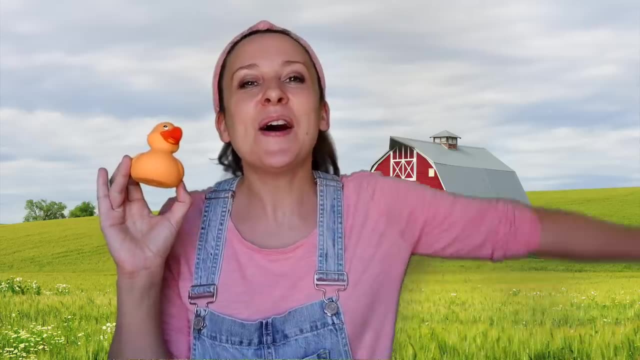 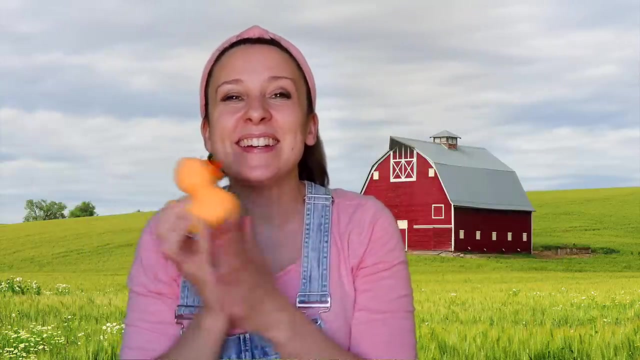 Here a quack, there a quack, everywhere a quack quack. Old MacDonald had a farm E-I-E-I-O, And on that farm he had a sheep E-I-E-I-O. Yay, Great job singing, Old MacDonald. 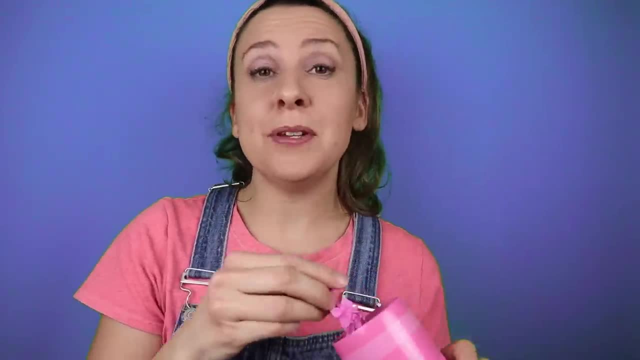 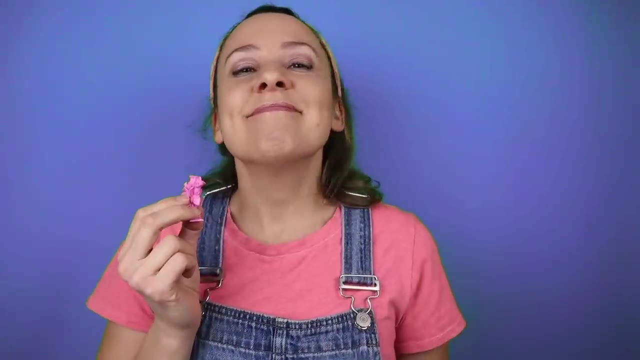 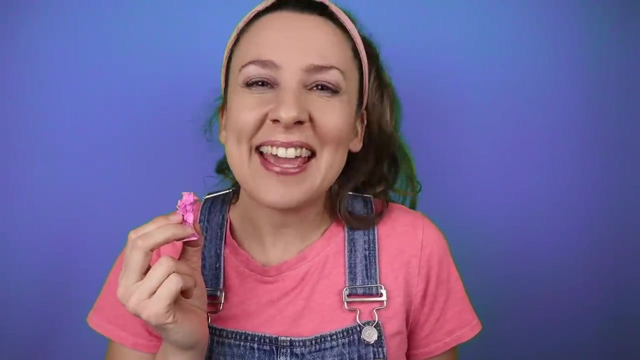 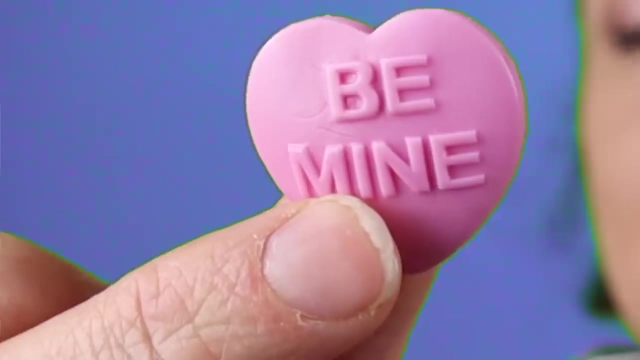 Whoa. next it's some beautiful pink flowers. Let's smell the pretend flowers, Mmm. flowers smell so nice. Flowers smell nice. Aww, Aww, So sweet. It's a pink heart, Skinamarink-a-dink-a-dink. 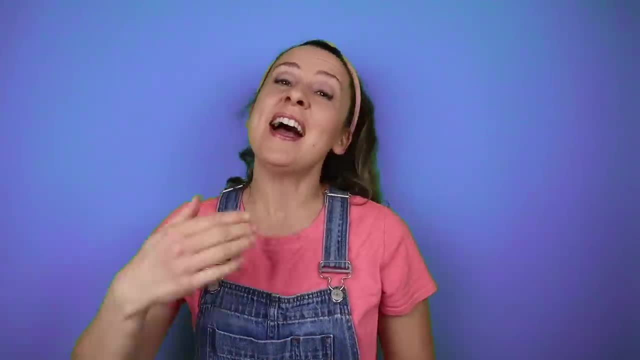 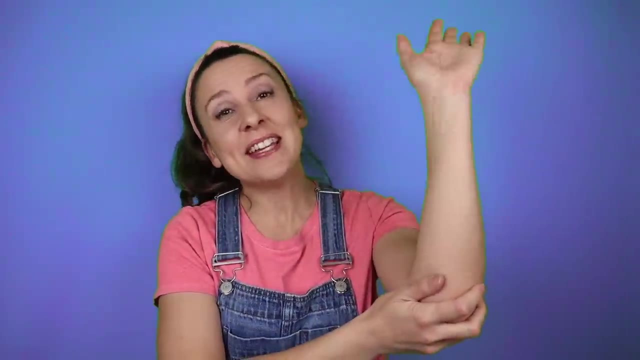 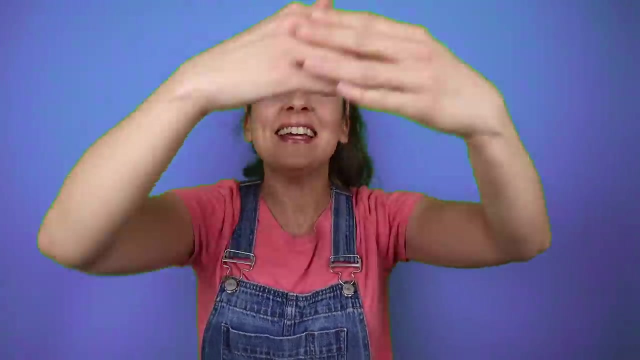 Skinamarink-a-do. I love you. Skinamarink-a-dink-a-dink, Skinamarink-a-do, I love you. I love you in the morning And in the afternoon. I love you in the evening And under the sun. 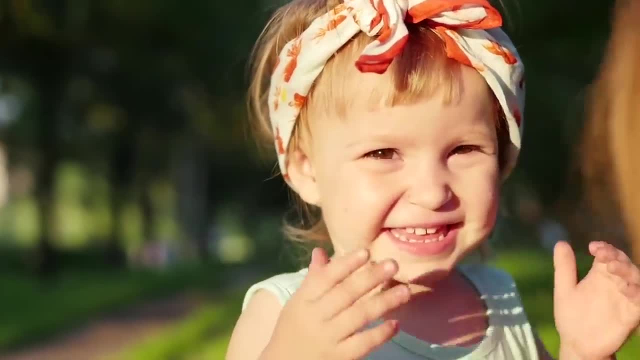 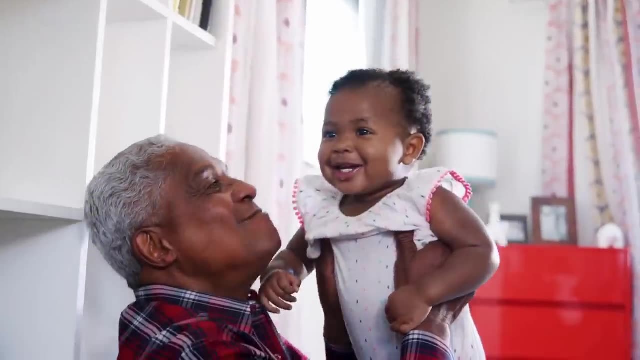 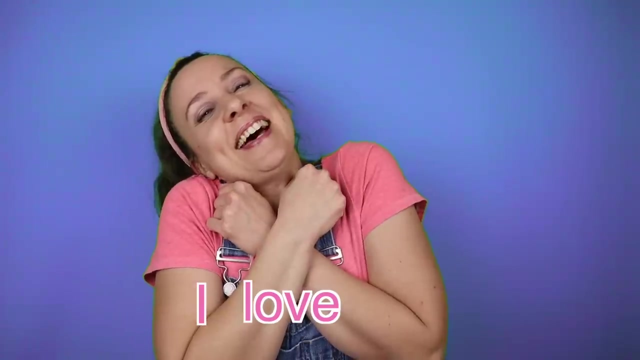 And under the sun, And under the sun, Underneath the moon, Oh, Skinamarink-a-dink-a-dink, Skinamarink-a-do, I love you, I love you. Yay, I love you, I love you. 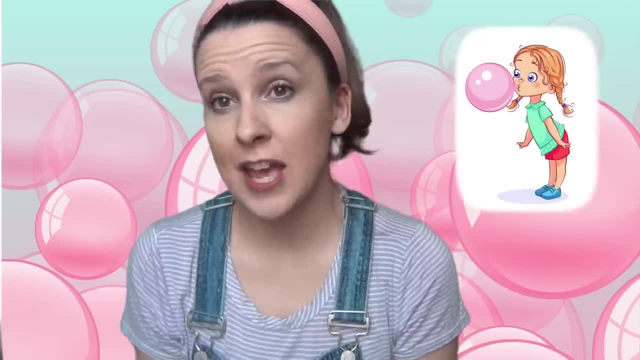 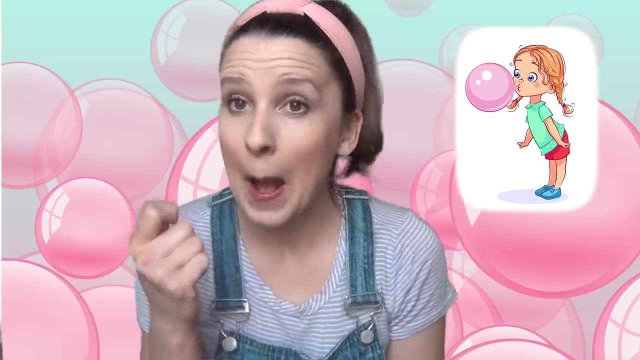 Or you could do this. I love you. We're gonna get out some pretend bubblegum. Okay, so get out some pretend bubblegum. What color is yours? Mine's pink. Put it in your mouth And we're gonna chew it. 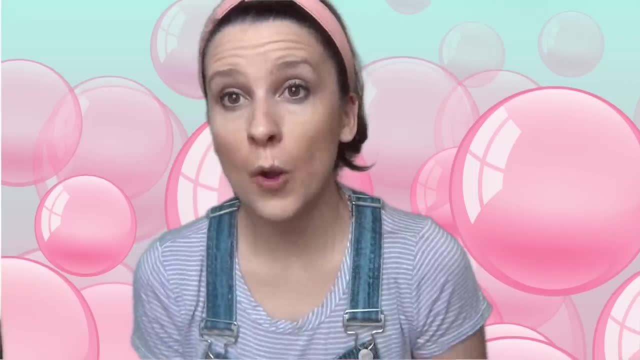 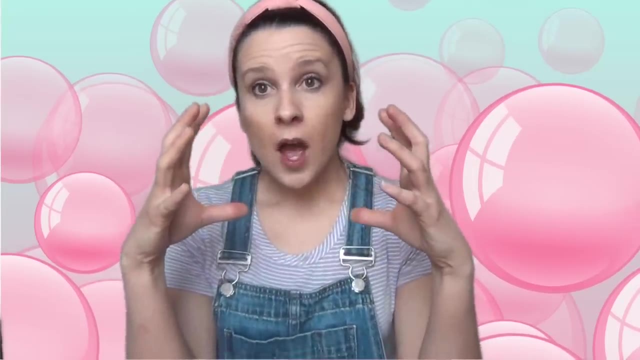 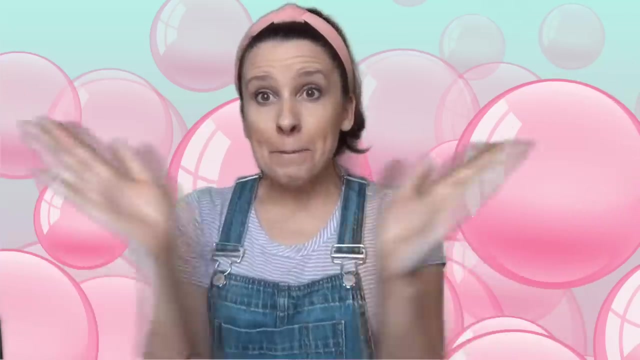 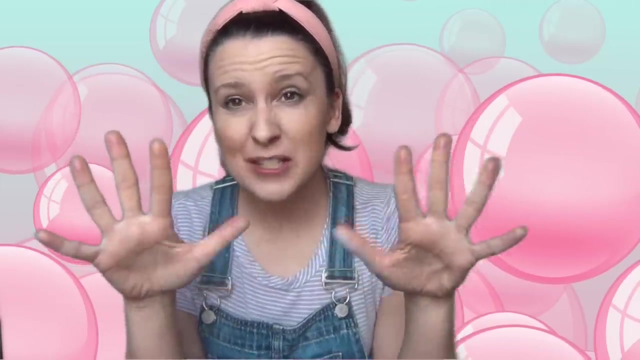 Are you chewing your gum? Okay, now we're gonna blow a really big bubble. Are you ready? Wow, Pop, Oh no, Our bubble popped And the sticky bubblegum is all over our hands. Icky, sticky, sticky, sticky bubblegum. 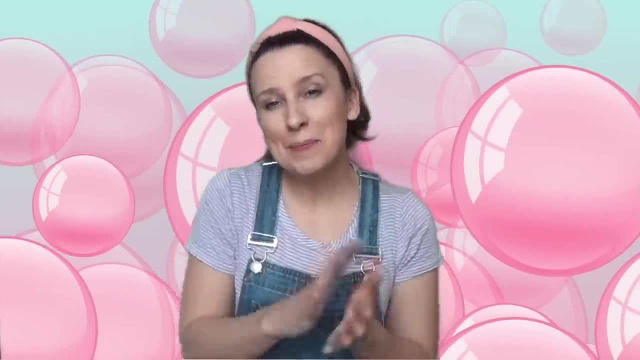 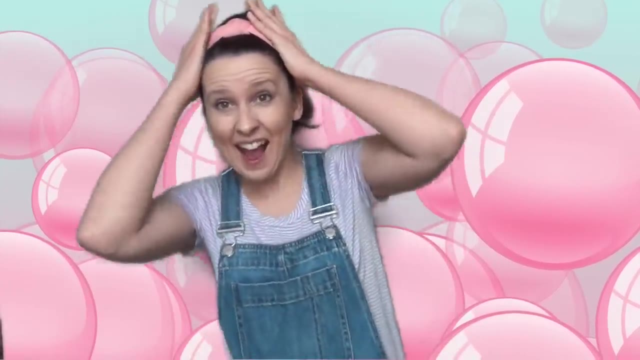 Icky, sticky, sticky, sticky bubblegum, Bubblegum Bubblegum. Icky sticky, sticky, sticky bubblegum Makes your hands stick to your head And you pull them, And you pull them. 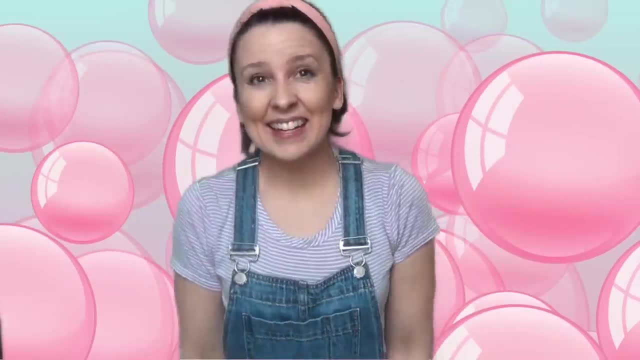 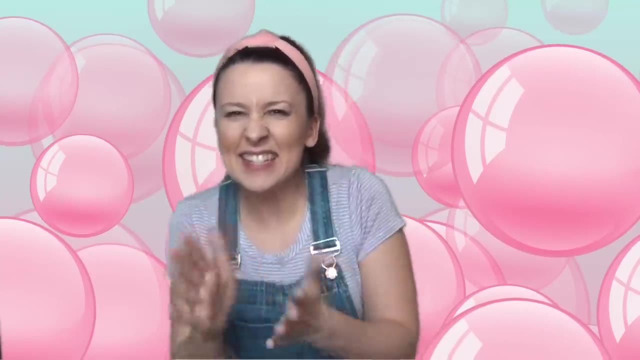 And you pull them away. Icky, sticky, sticky, sticky bubblegum, Bubblegum Bubblegum. Icky, sticky, sticky sticky bubblegum. Makes your hands stick to your elbows And you pull them. 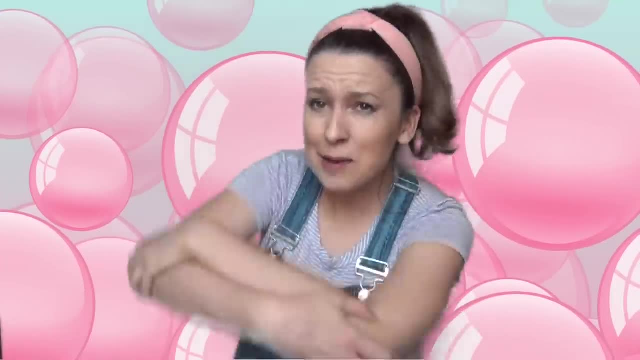 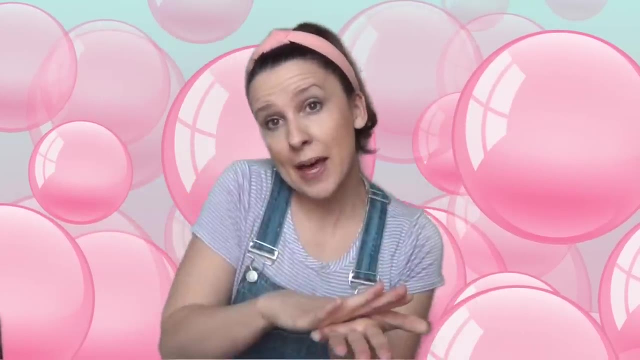 And you pull them, And you pull them away. Icky, sticky, sticky, sticky bubblegum, Bubblegum Bubblegum. Icky, sticky, sticky, sticky bubblegum Makes your hands stick to your tummy. 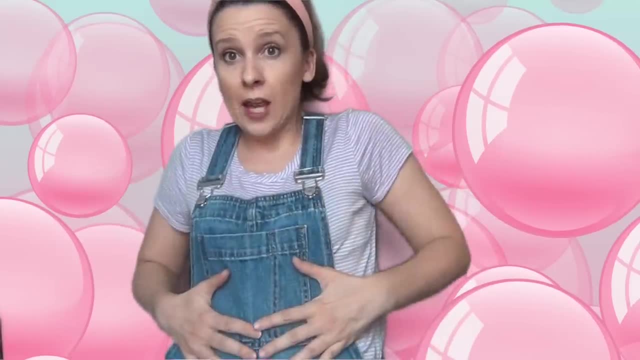 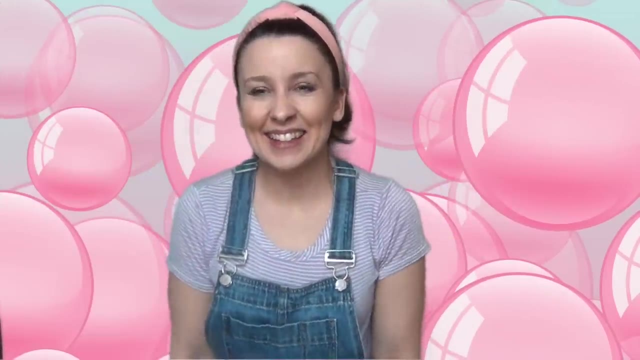 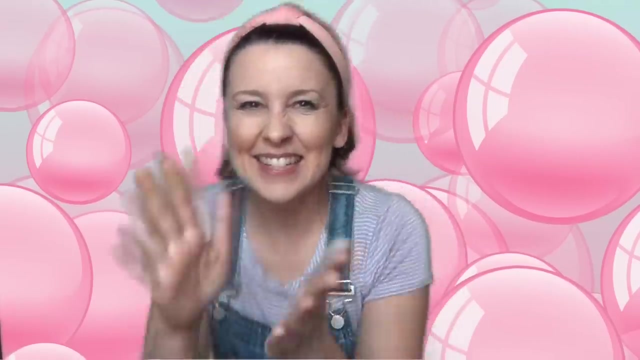 And you pull them, And you pull them, And you pull them away. Icky, sticky, sticky, sticky bubblegum Bubblegum Bubblegum. Icky, sticky, sticky, sticky bubblegum bubblegum bubblegum. icky, sticky, sticky, sticky bubblegum makes your hands stick to. 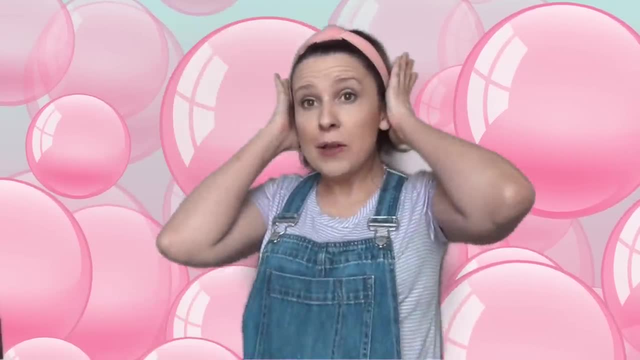 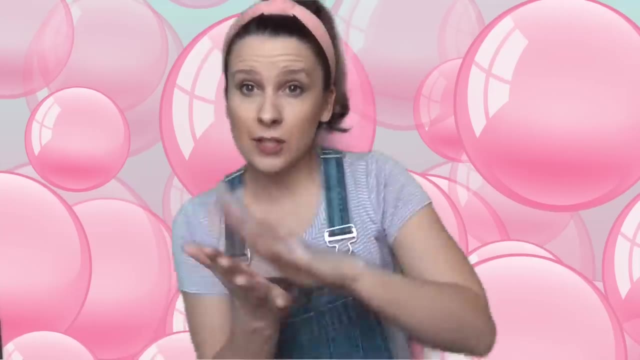 your ears And you pull them, and you pull them, and you pull them away. Icky, sticky, sticky sticky bubblegum, bubblegum bubblegum, icky, sticky, sticky sticky bubblegum makes. 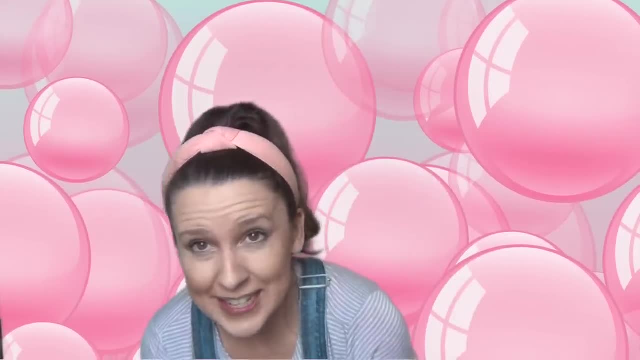 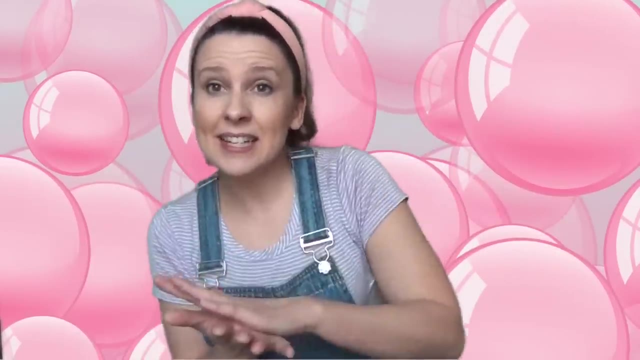 your hands stick to your knees. Are they on your knees? And you pull them, and you pull them away. Icky sticky, sticky sticky bubblegum, bubblegum bubblegum, icky sticky sticky. 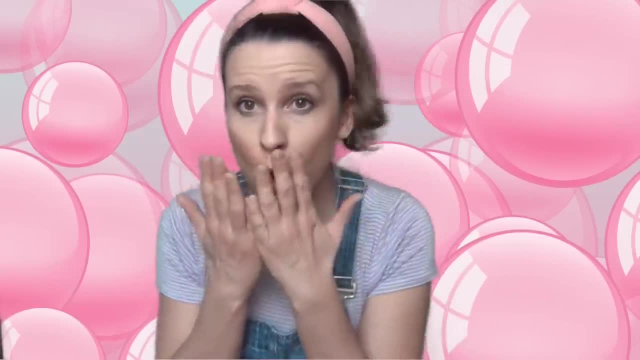 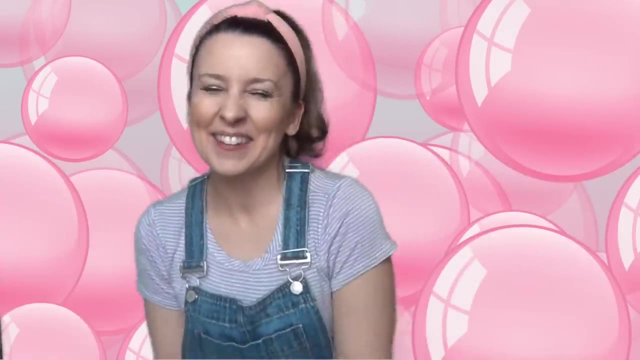 sticky bubblegum makes your hands stick to your mouth. Ba-do-ba-ba, ba-ba-ba-ba, da-ba-do-ba-ba-ba. Icky, sticky, sticky, sticky bubblegum bubblegum. 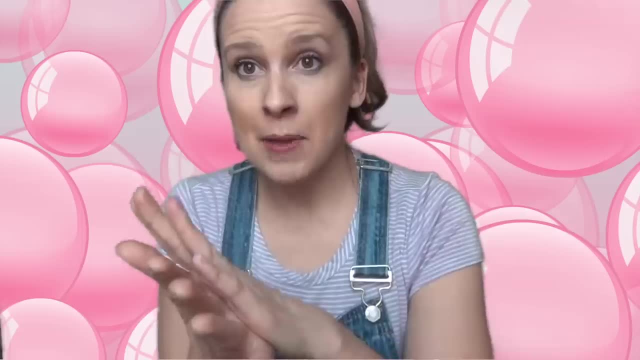 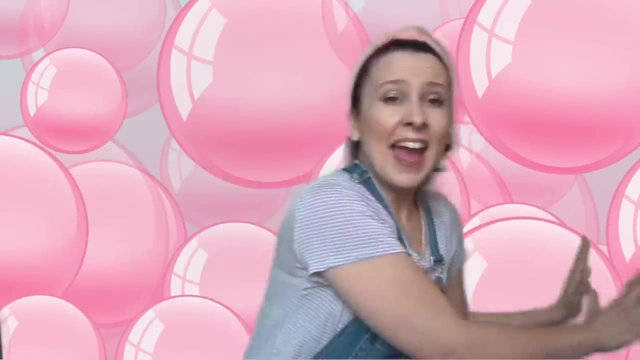 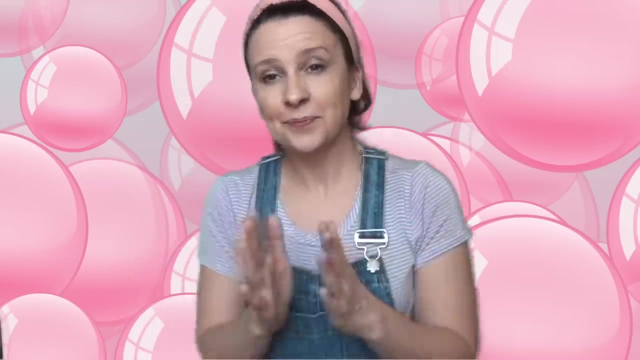 bubblegum. icky, sticky, sticky, sticky bubblegum makes your hands stick to your grown-up. Put them on your grown-up And you pull them, and you pull them, and you pull them away. That was so fun. One more time: Icky, sticky, sticky, sticky bubblegum. 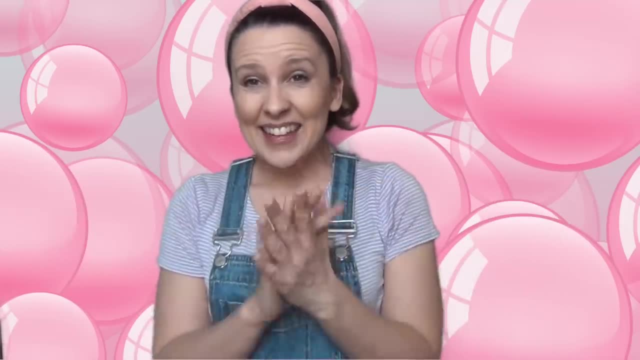 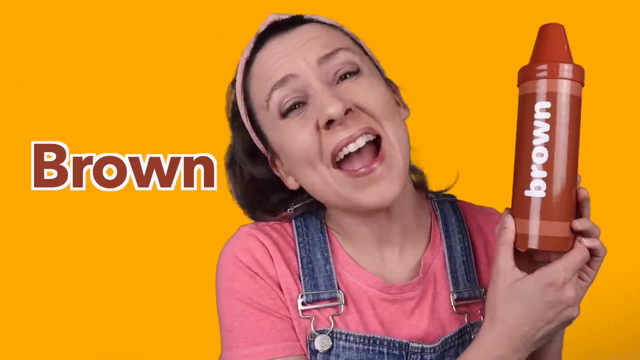 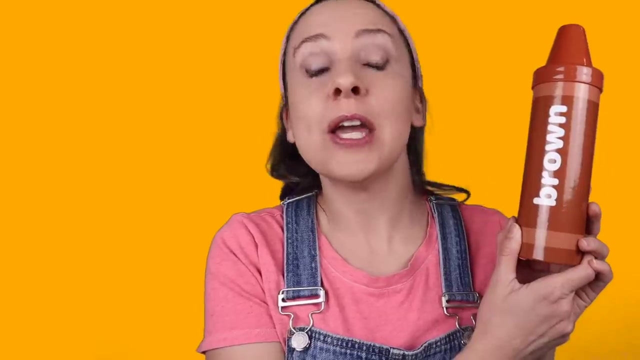 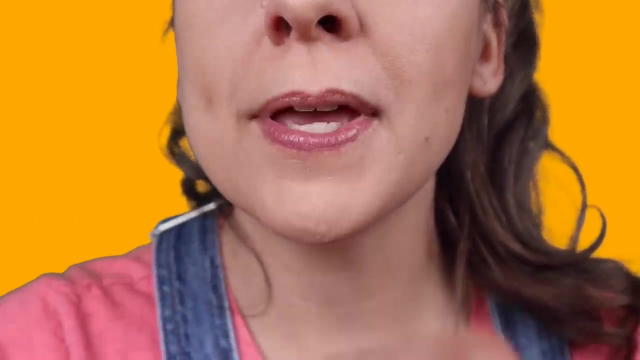 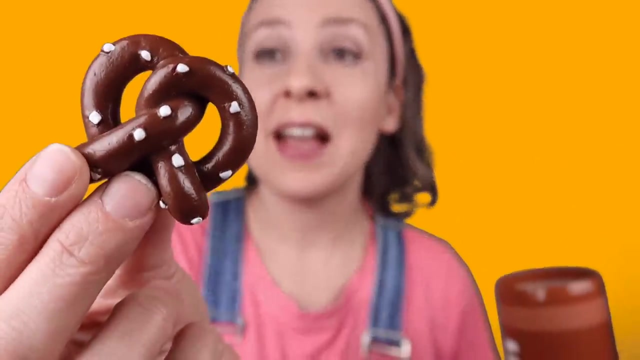 makes your hands stick to your. Yay, That was so much fun. Our next color is brown, Brown. Wow, Let's see what's inside the brown crayon. Can you say: open, Open, Open, It's opening. It's a brown pretzel. Pretzels are so yummy. 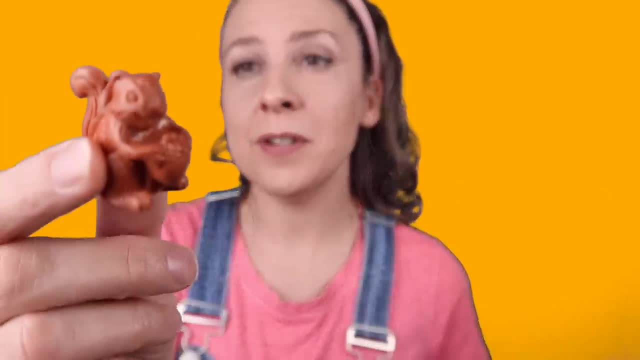 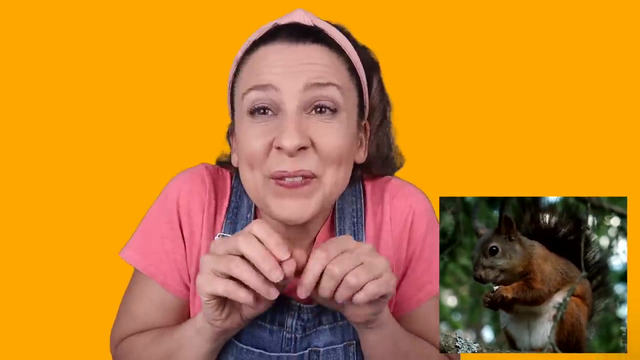 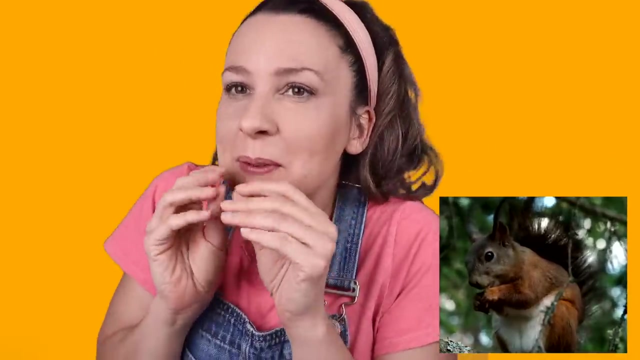 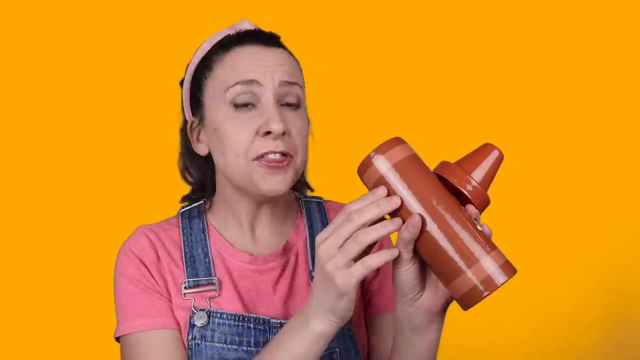 Oh wow, It's a little pretzel. It's a little brown squirrel with a little brown nut. Can you pretend to be a little squirrel eating nuts? Let's be a squirrel eating nuts, Eee-ee, Eee-ee, Eee-ee, Eee-ee, Eee-ee. Hmm, I thought I had a cookie in here Where. 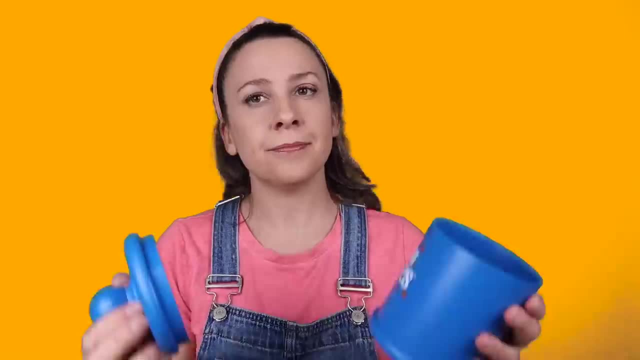 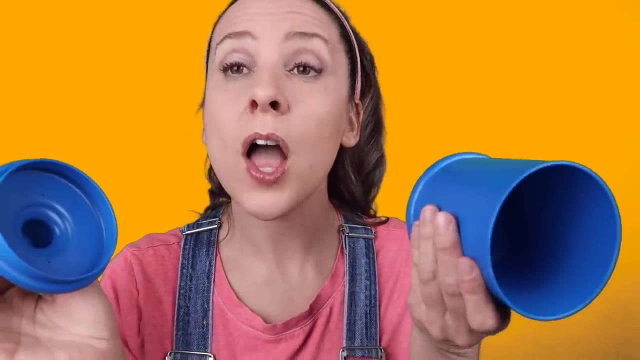 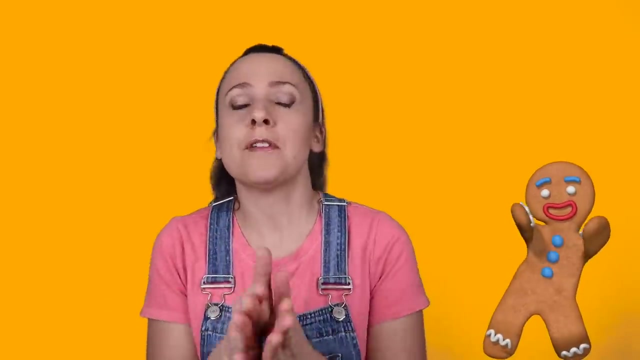 could it be? Maybe it's in the cookie jar, Oh, Uh-oh, Can you say that? Uh-oh, The cookies are missing. Hmm, Who stole the cookies from the cookie jar? Ms Rachel stole the cookies from the cookie jar. Who me? Yes, you couldn't. 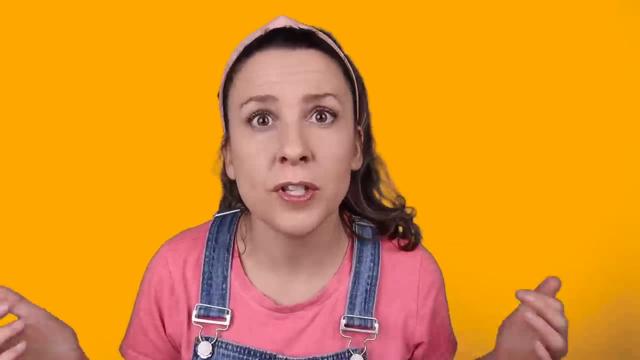 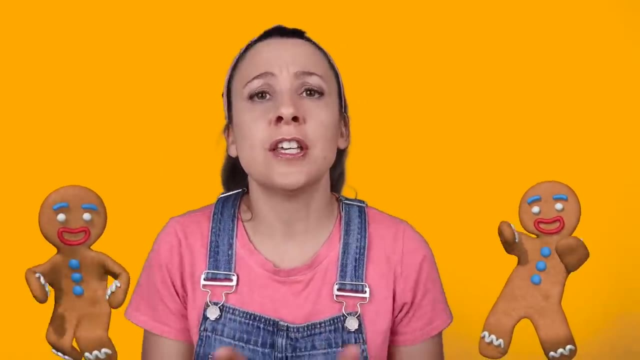 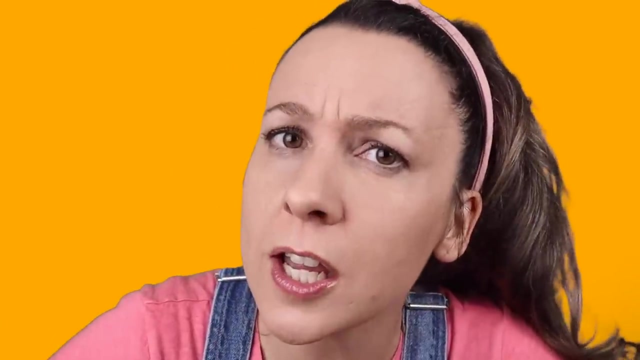 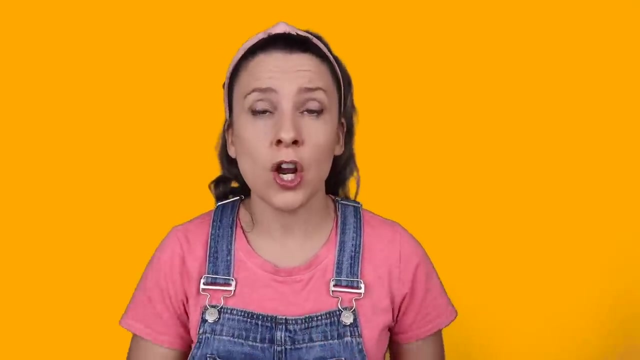 be, Then who? Who stole the cookies? Was it you Who stole the cookies from the cookie jar? Yes, you couldn't be. Then who? Hmm, Do you think it was David Dogg Who stole the cookies from the cookie jar? David Dogg stole the cookies from the cookie jar. Who me? Yes, 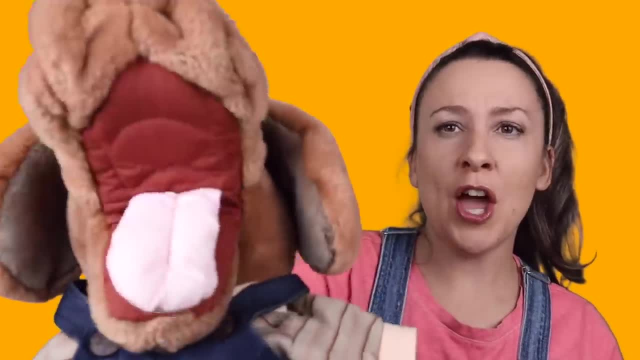 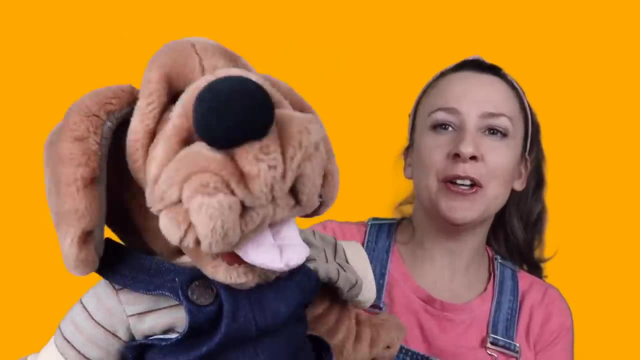 you couldn't be, Then who? Okay, It was me, David Dogg, you took the cookies. Yeah, I'll give them back. Aw, thanks, David. Thank you, You're welcome. I love you so much, That's nice. 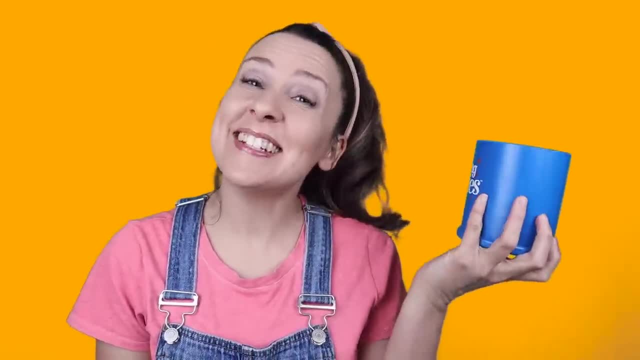 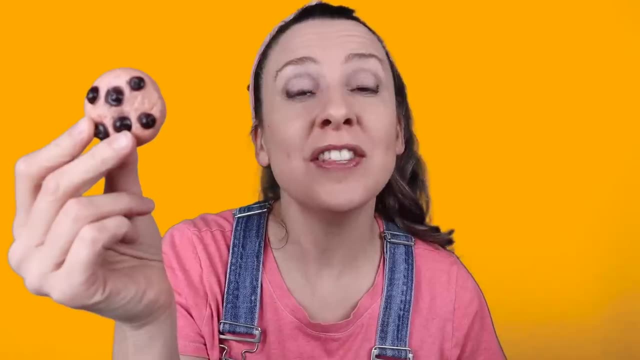 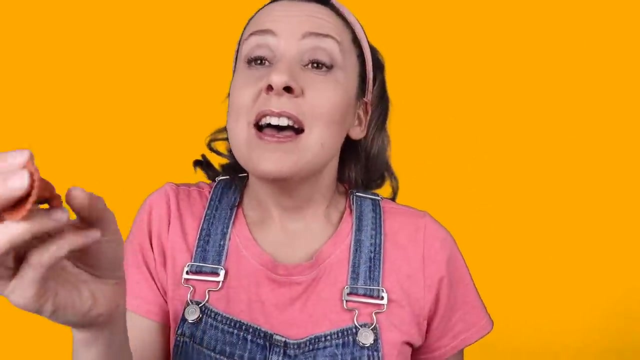 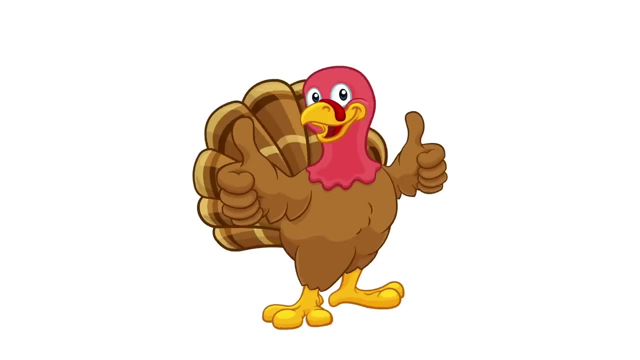 Yay, David Dog, put the cookies back in the jar. Look, A brown cookie with chocolate chips, Yummy. Next it's a little brown turkey. Turkeys say gobble, Gobble, gobble, gobble, Gobble, gobble, gobble. 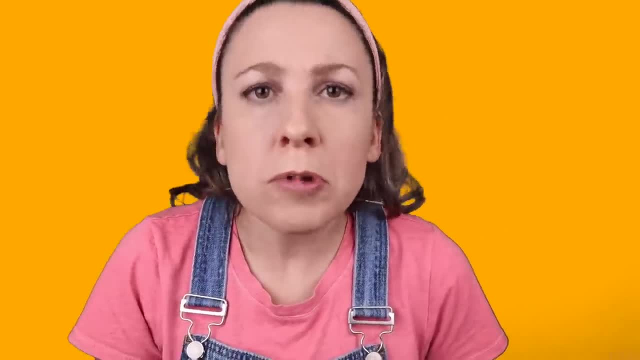 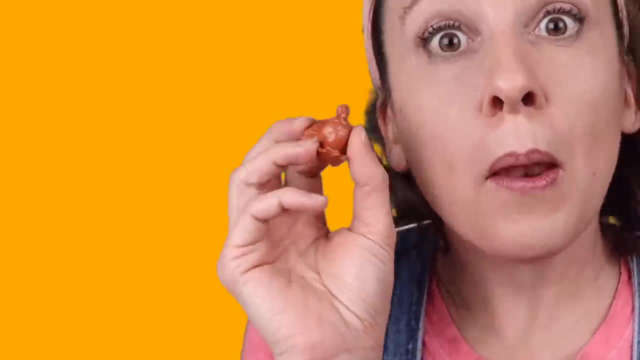 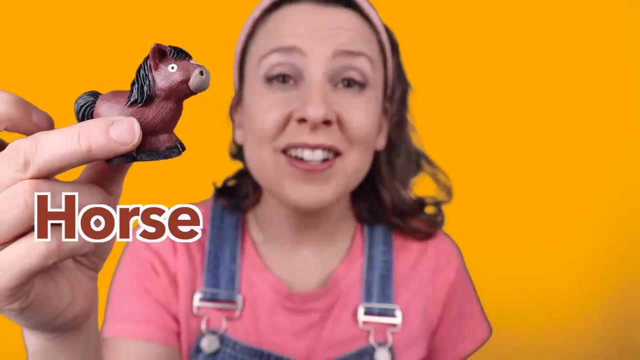 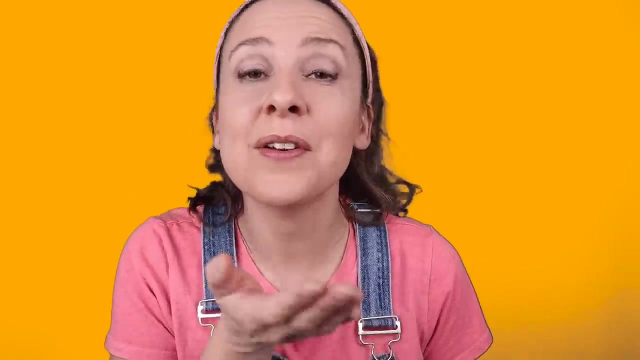 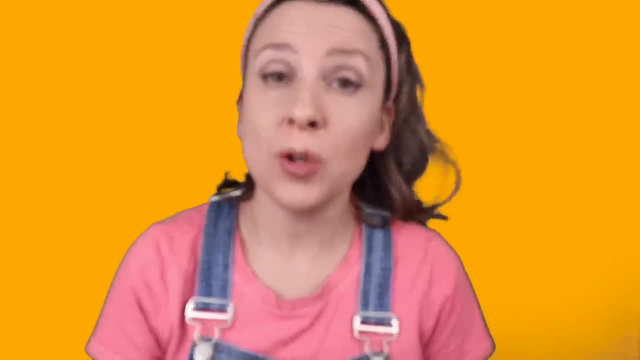 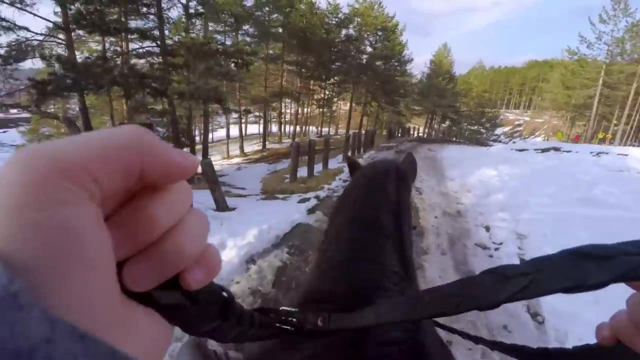 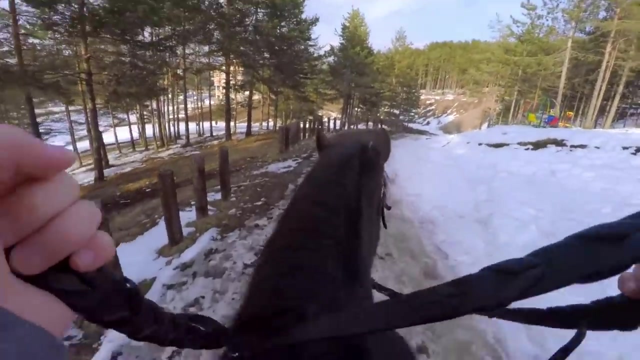 H, h, h, h, h. horse. What does a horse say? Knee knee, knee. Sometimes, when you ride a horse, you say yee-haw. Can you say that? Yee-haw, yee-haw? 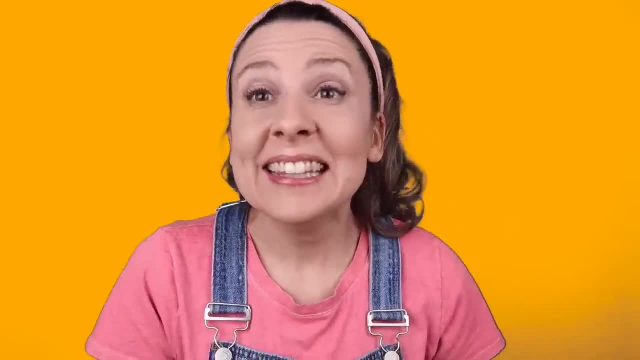 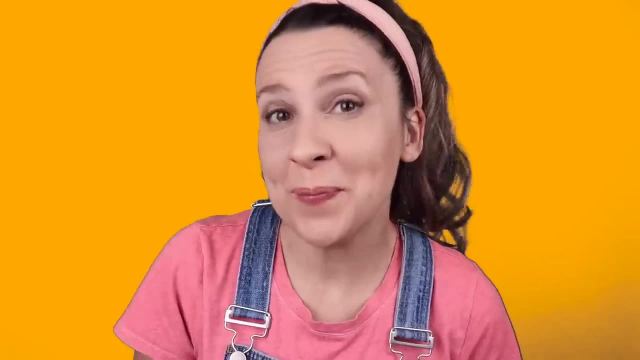 Let's pretend we're riding on a horse. Hey, let's sing. She'll Be Comin' Around the Mountain. Can you pretend to gallop like a horse around the room? She'll be comin' round the mountain when she comes. 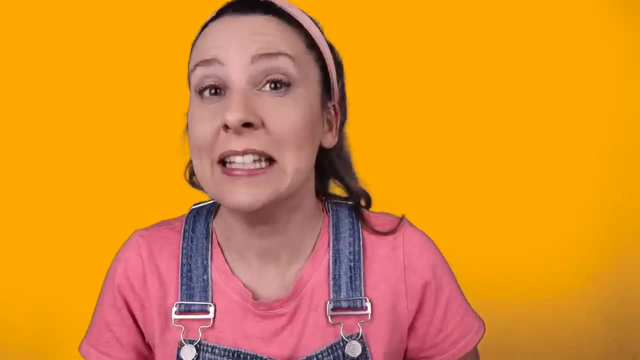 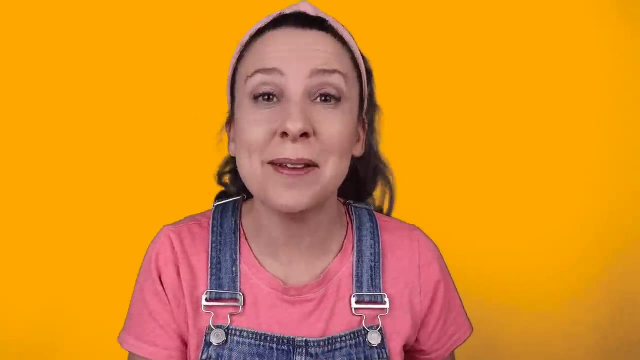 Yee-haw, she'll be comin' round the mountain when she comes. Yee-haw, she'll be comin' round the mountain. She'll be comin' round the mountain. She'll be comin' round the mountain when she comes. 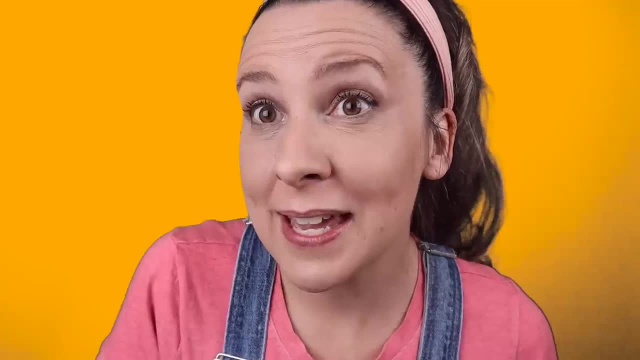 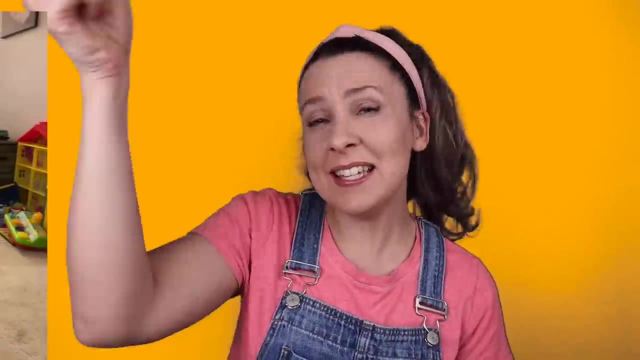 Yee-haw, she'll be riding six white horses. when she comes Yee-haw, she'll be riding six white horses. when she comes Yee-haw, she'll be riding six white horses. She'll be riding six white horses. 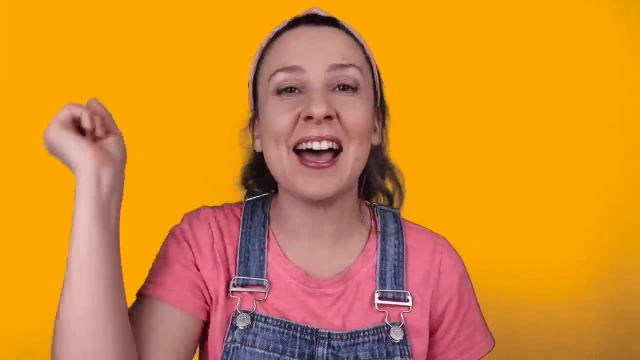 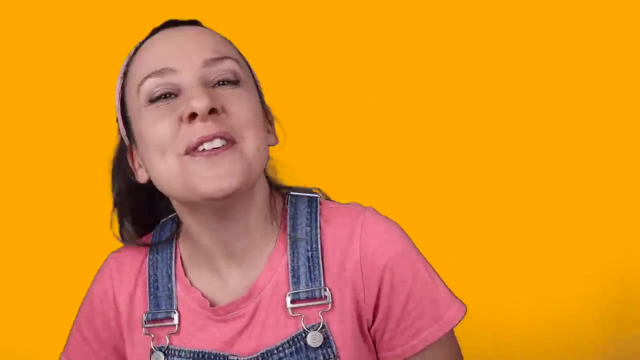 She'll be riding six white horses. when she comes Yee-haw, we will all go out to meet her. when she comes Hi babe, we will all go out to meet her. when she comes Hi babe, we will all go out to meet her. 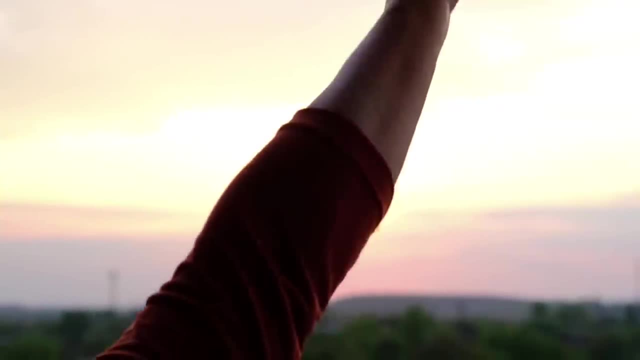 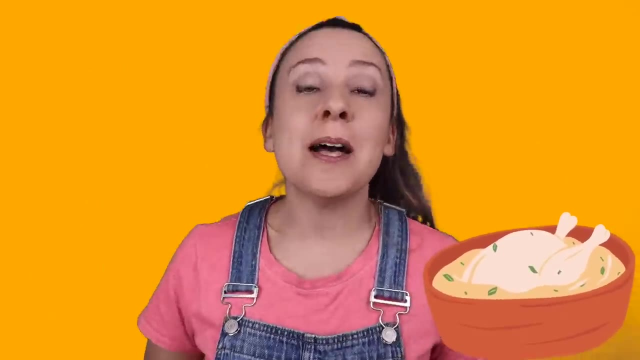 We will all go out to meet her. We will all go out to meet her when she comes. Hi, babe, we will all have chicken and dumplings when she comes. Yum, yum, We will all have chicken and dumplings when she comes. 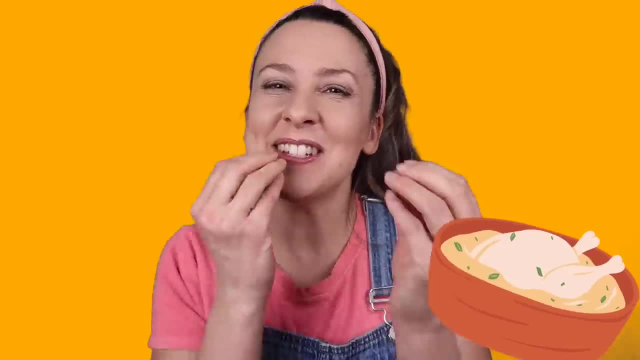 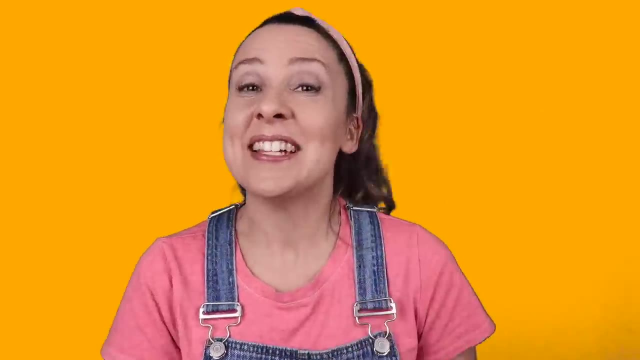 Yum yum, We will all have chicken and dumplings. We will all have chicken and dumplings. We will all have chicken and dumplings when she comes. Yum yum, Yay. That's a great song, Oh wow. 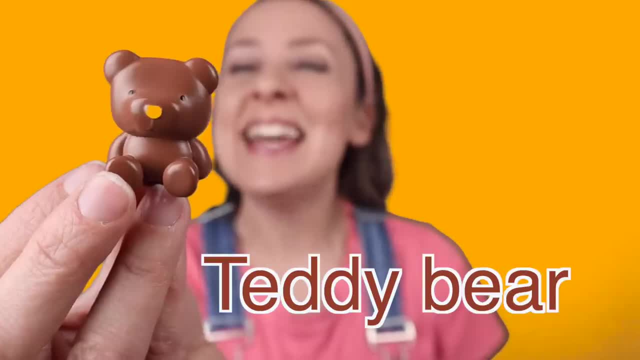 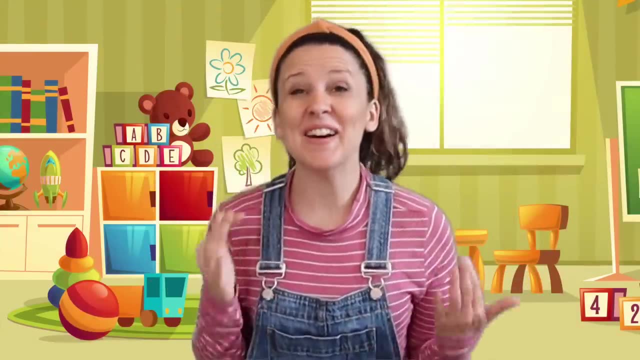 It's a little brown teddy bear, So cute. Do you have a teddy bear? Wow, If you want, you can get out your teddy bear for this rhyme: Teddy bear, teddy bear, turn around. Teddy bear, teddy bear, touch the ground. 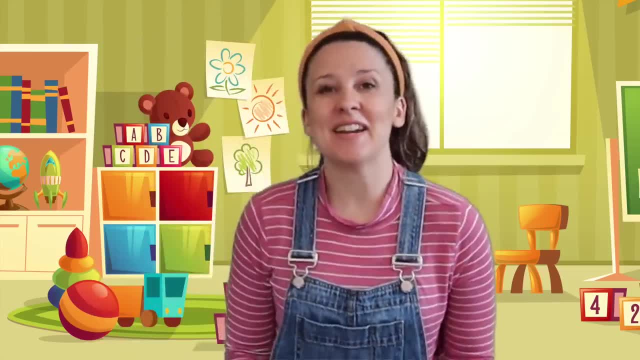 Teddy bear- teddy bear, reach up high. Teddy bear- teddy bear, touch the sky. Teddy bear- teddy bear, bend down low. Teddy bear teddy bear, touch your toes. Teddy bear teddy bear, go to bed. 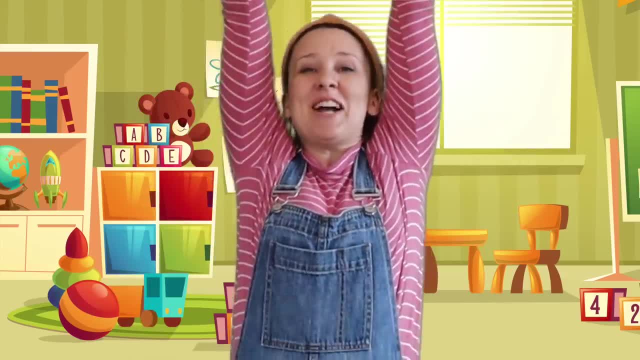 Teddy bear, teddy bear, rest your head. Teddy bear, teddy bear, touch your toes. Teddy bear, teddy bear, go to bed. Teddy bear, teddy bear, rest your head. Teddy bear, teddy bear, go to bed. 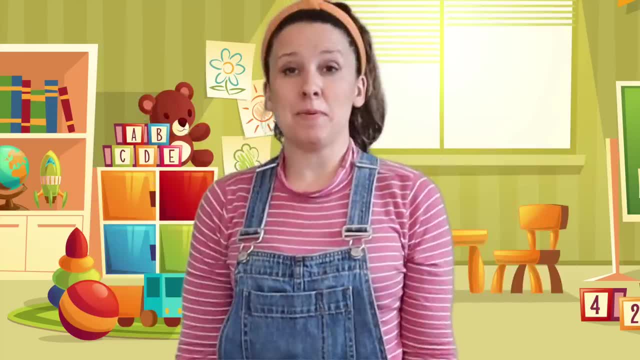 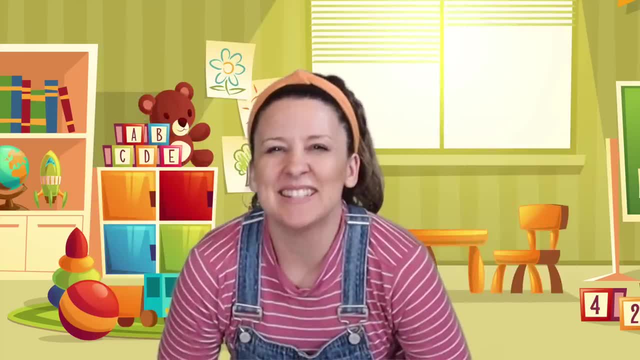 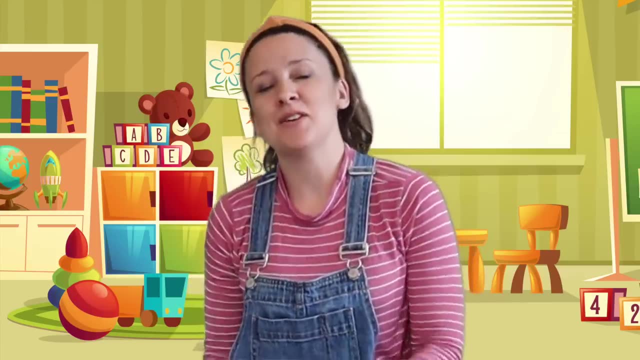 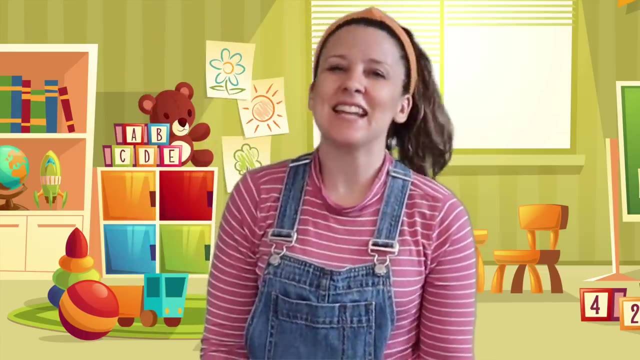 Teddy bear, teddy bear, go to bed. Teddy bear, teddy bear, touch your toes. Teddy bear, teddy bear, go to bed. Teddy bear, teddy bear, rest your head. Teddy bear, teddy bear, turn off the light. 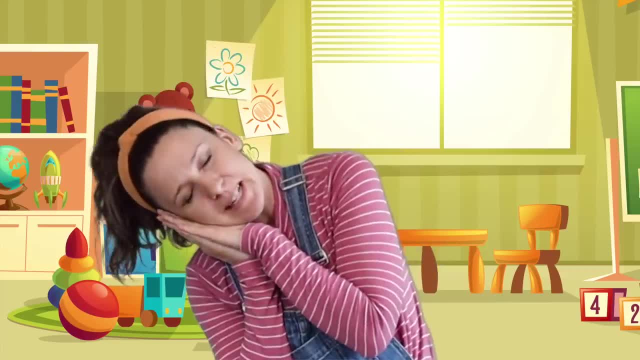 Click Teddy bear. teddy bear say good night. Oh, the teddy bear is so tired. Pretend to go to sleep or put your teddy bear to bed. Ding, ding, ding, ding, ding. That's our alarm clock. 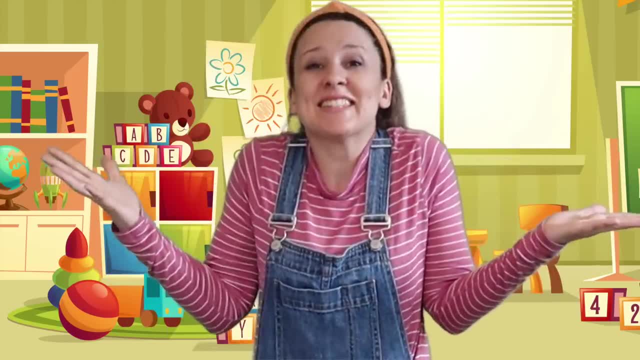 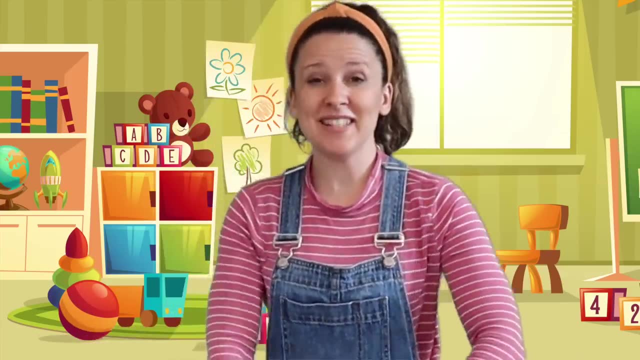 Next one, Next one, Next one clock. We have to get up and sing more songs. Teddy bear, teddy bear, find your nose. Teddy bear, teddy bear, touch your toes. Oh, touch your toes, Teddy bear, teddy bear, touch. 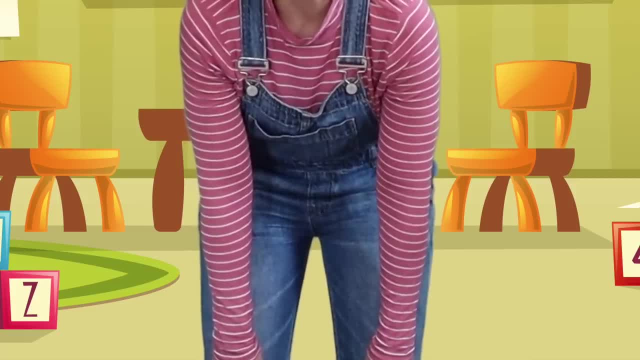 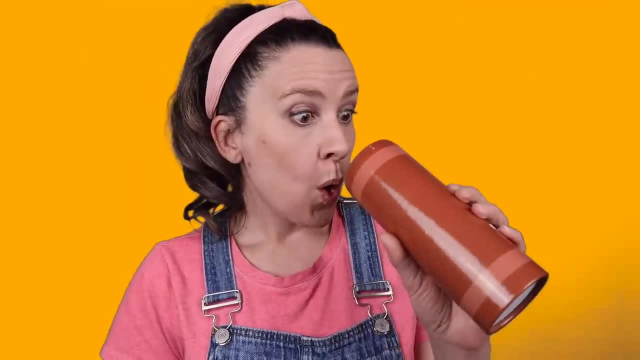 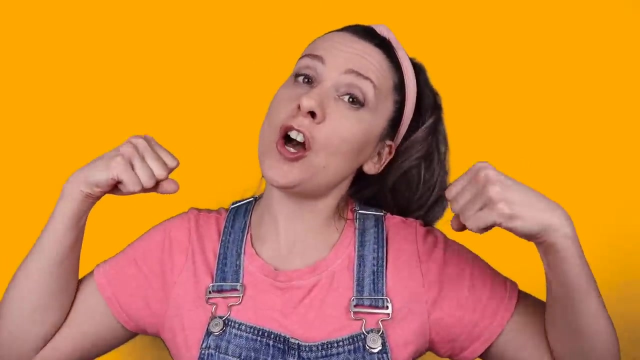 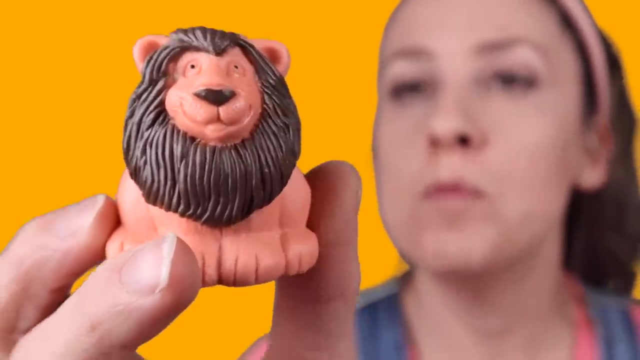 your knees. Are you touching your knees? Teddy bear, teddy bear, sit down, please. Are you sitting down? Good job, Oh, it's a big strong lion. I'm a big strong lion, I'm a big strong. 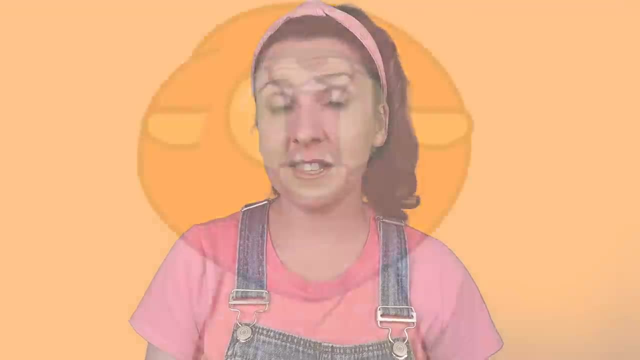 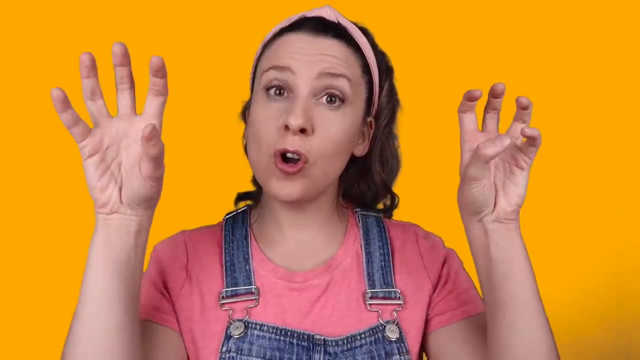 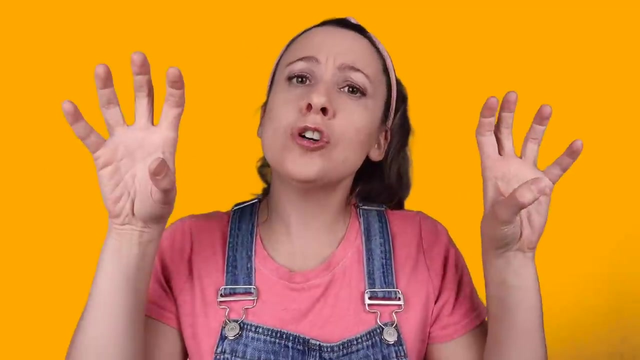 lion Roar. Can you roar like a lion? Roar, Roar, Roar. Good job, Roar. Oh, you scared me, That was such a big roar. Can you do it again, Roar? Oh, you scared me, That was a. 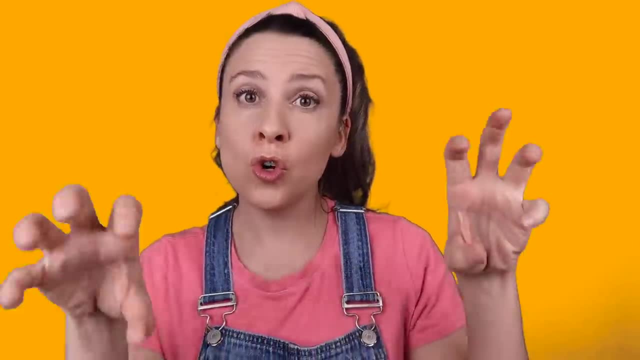 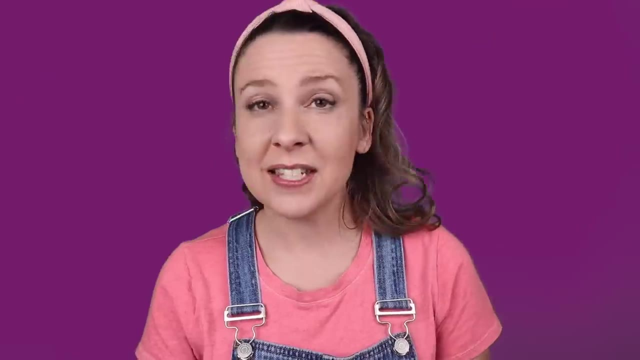 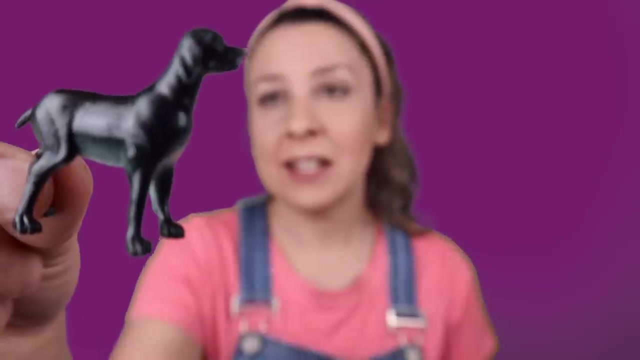 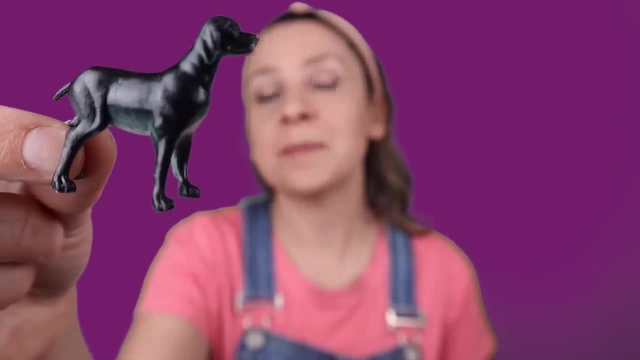 big roar. Can you do it even louder? Roar? You scared me Just for pretend That was silly. This is the color black. What color is this Roar Roar? Yeah, it's a black dog. A black dog, What does a? 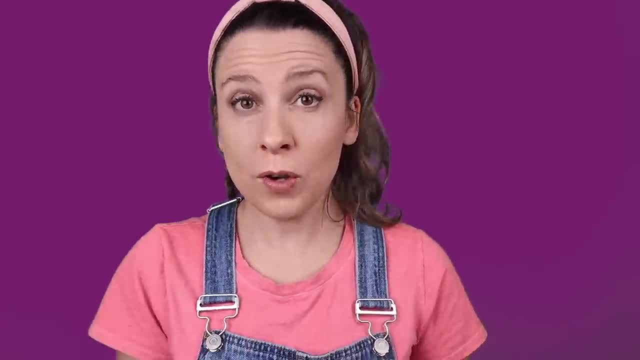 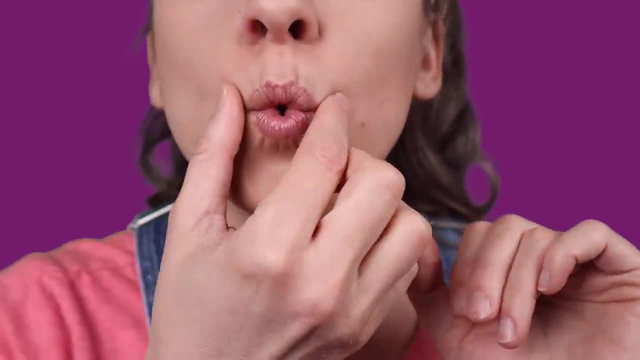 dog say: Woof, woof, woof, woof. Can you bark like a doggy? Woof, woof, woof, woof, Wooah, wooah, wooah. Good job barking. You bark just like me. 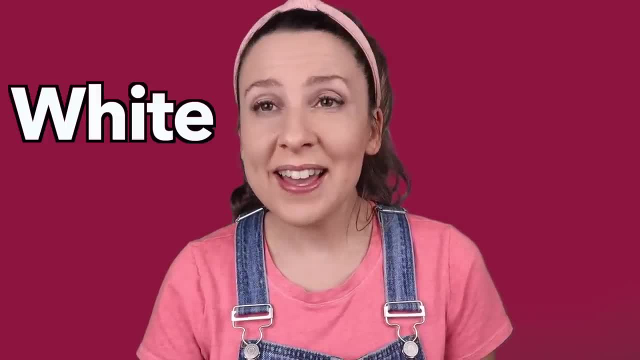 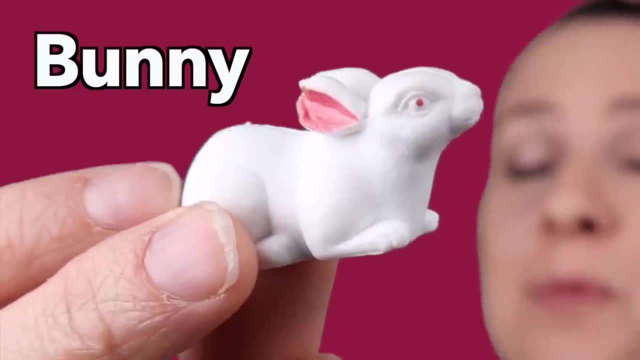 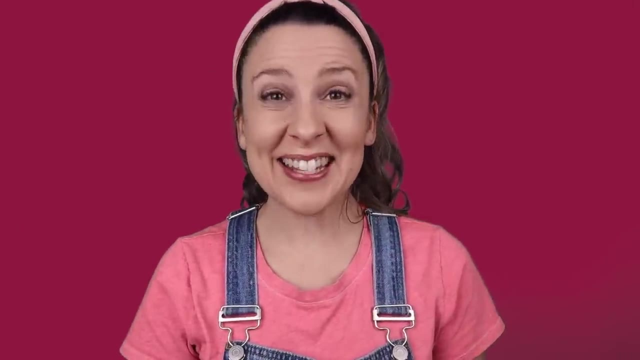 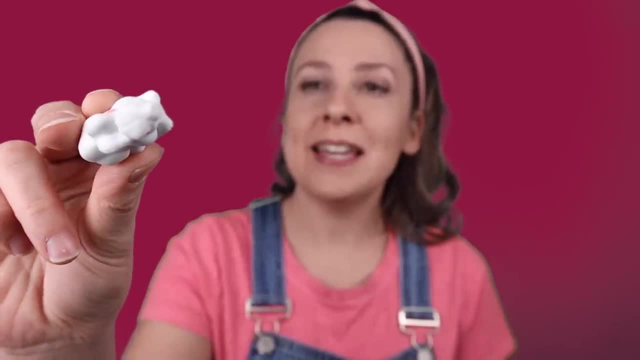 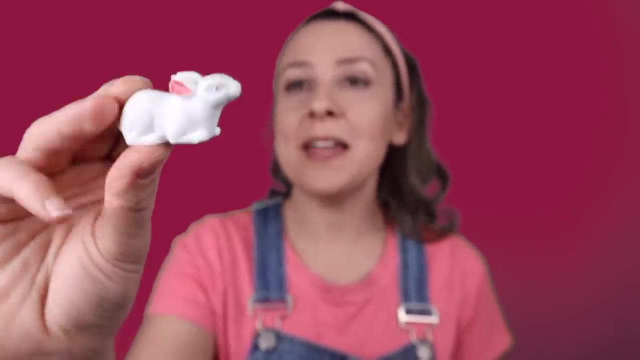 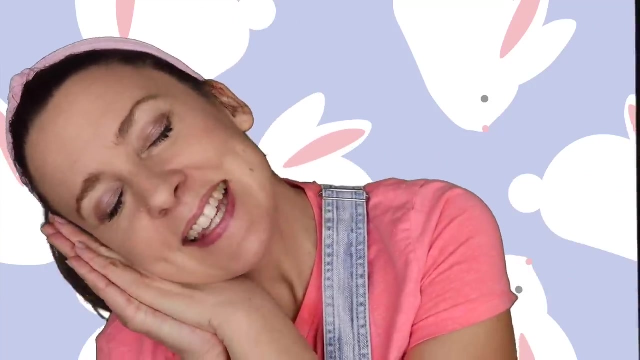 was silly. Good night bunny Shh shh, ding, ding, ding ding. It's your alarm clock. Oh, you have to wake up and hop. Let's pretend we're bunnies. See the bunny sleeping, till it's. 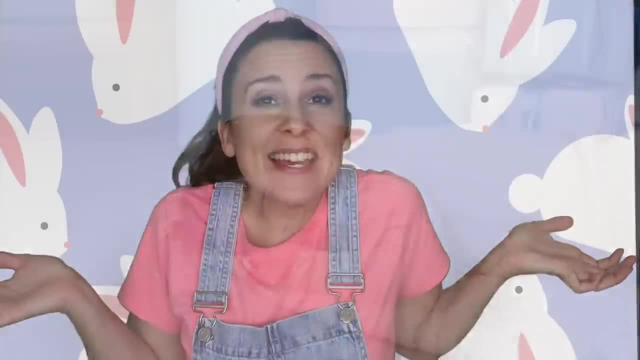 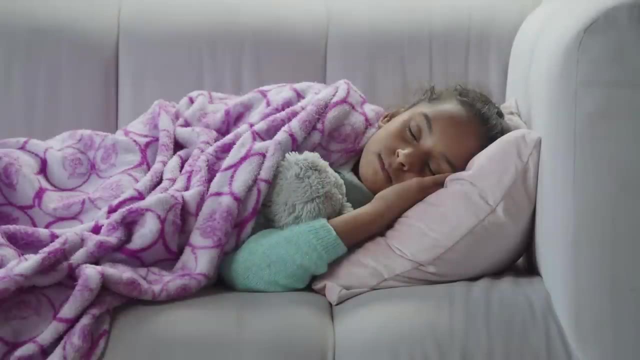 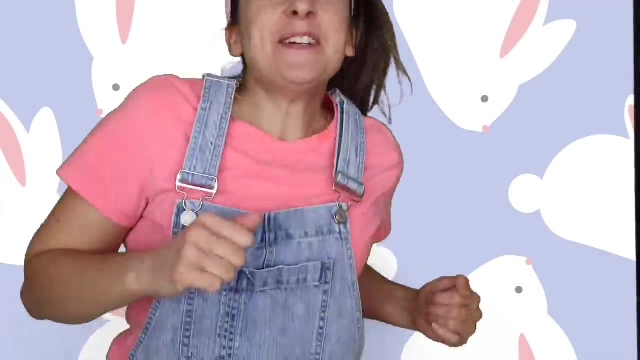 nearly noon. Shall we wake them with a merry tune. They're so still Are they ill. Wake up soon. Wake up, little bunnies, Hop, little bunnies, Hop, hop, hop, Hop, little bunnies, Hop, little bunnies mistakes. 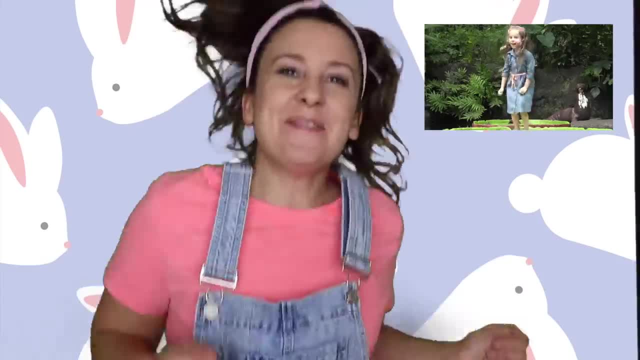 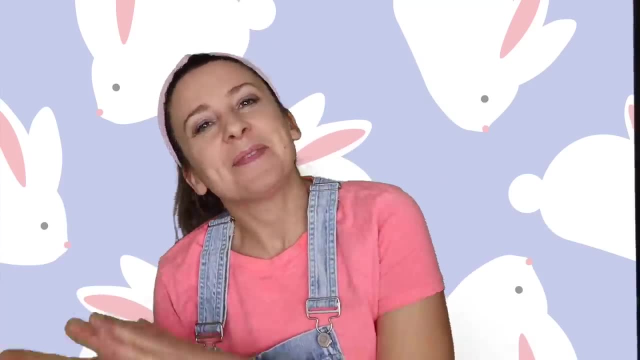 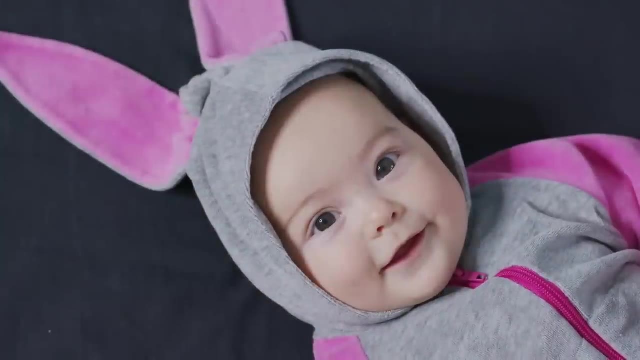 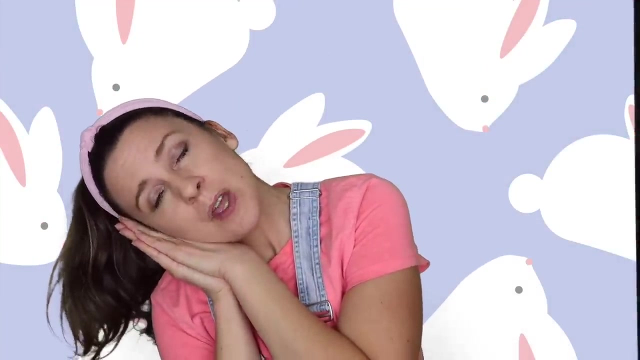 hop, hop, hop, hop. little bunnies, hop, hop, hop, hop. little bunnies, hop, hop, hop, hop, hop, hop and stop. let's go back to sleep. see the bunny sleeping till it's nearly noon. shall we wake them with a merry tune? they're so still, are they ill? wake up soon. wake up, little bunnies skip. little bunnies skip. 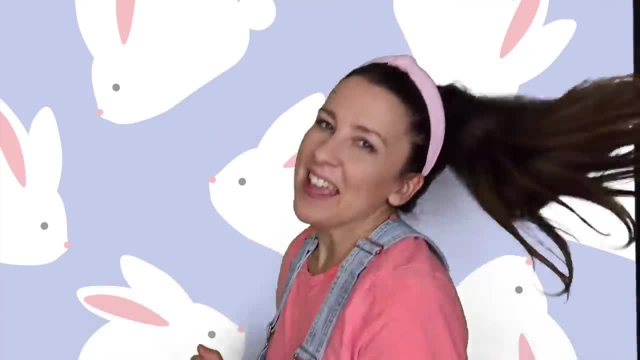 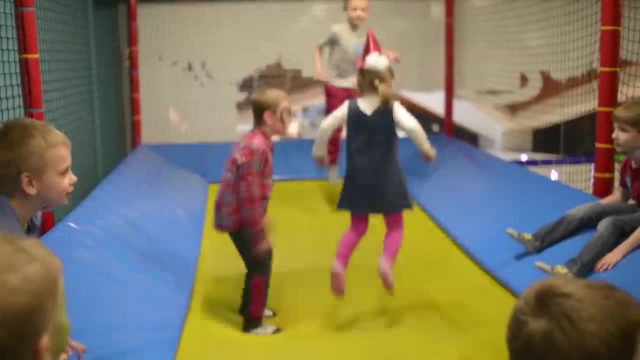 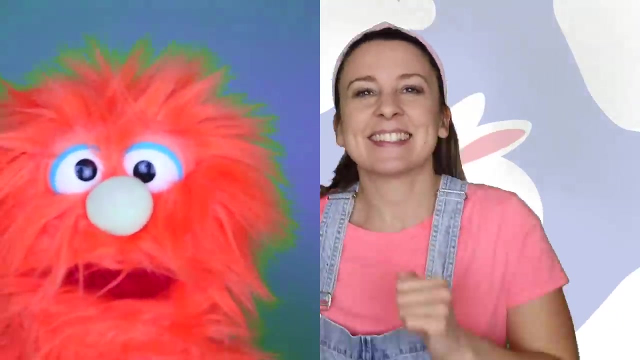 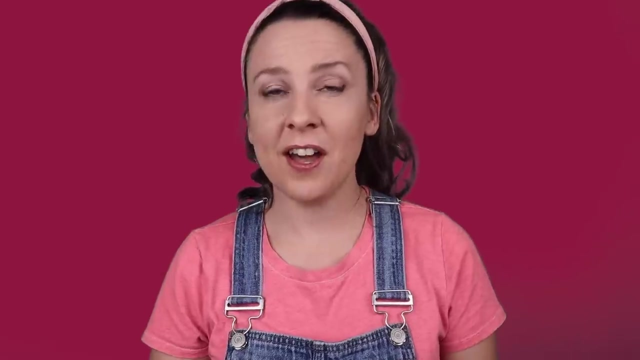 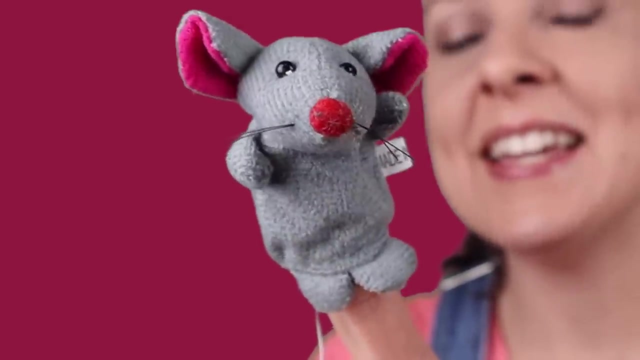 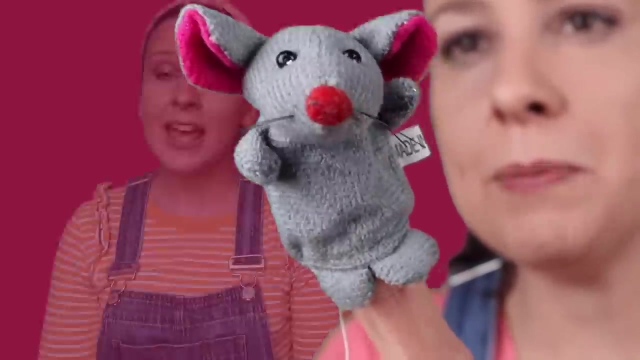 skip, skip, skip little bunny, skip, skip, skip, skip, little bunnies, skip, skip, skip, skip, skip, skip, stop, Yay, Great job. This color is gray. I have a little gray mouse. Can you squeak like a mouse? Squeak, squeak, Squeak, squeak. Can you pretend your little thumb is a mouse? 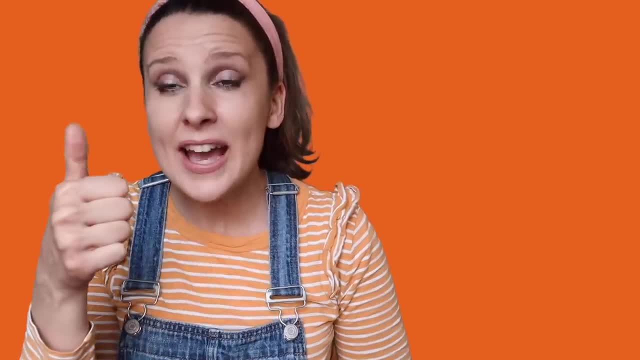 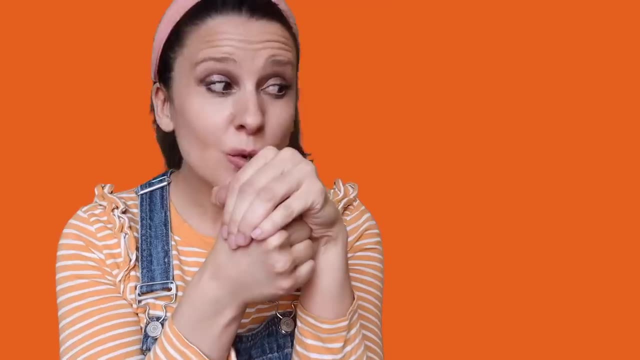 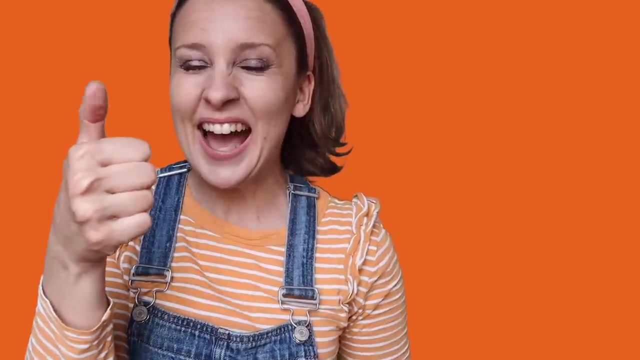 And your other hand's going to be the house. A quiet little mouse in a quiet little house, When all was quiet as quiet can be. Shh, shh, shh, Alphatee. What a silly mouse, Let's. 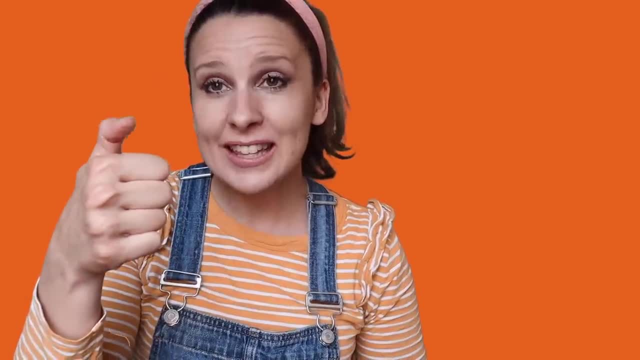 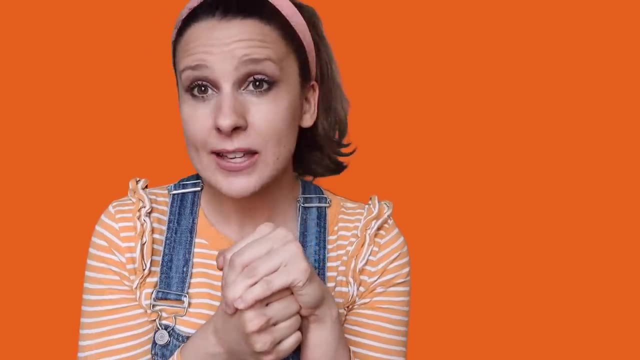 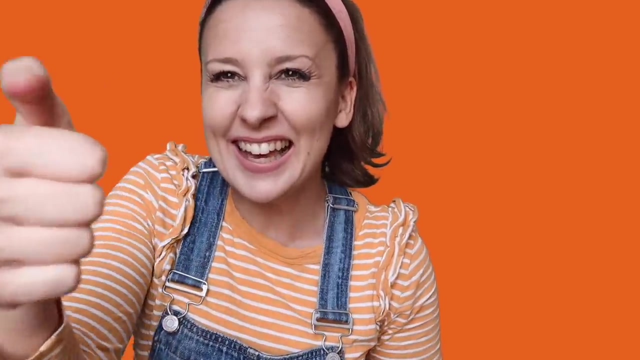 try that again. That was so silly. A quiet little mouse in a quiet little house, When all was quiet As quiet can be. Shh, shh, shh, Alphatee. That was so silly, The little mouse surprised. 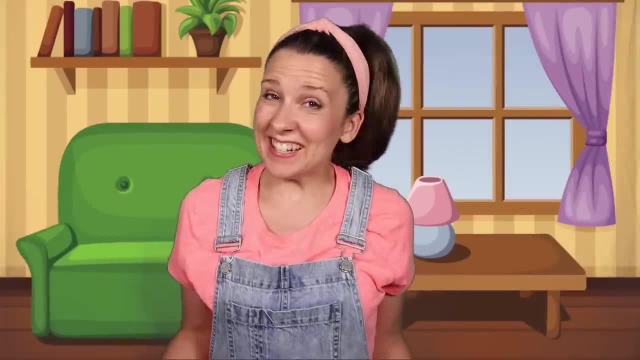 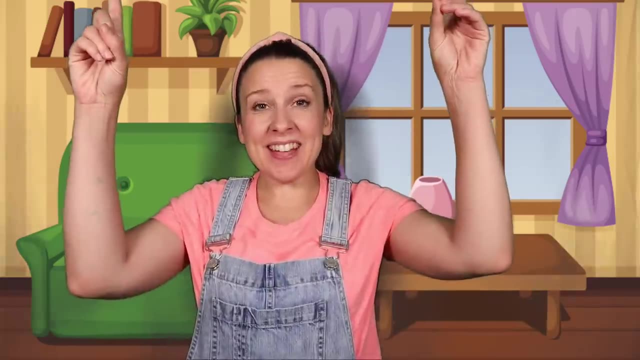 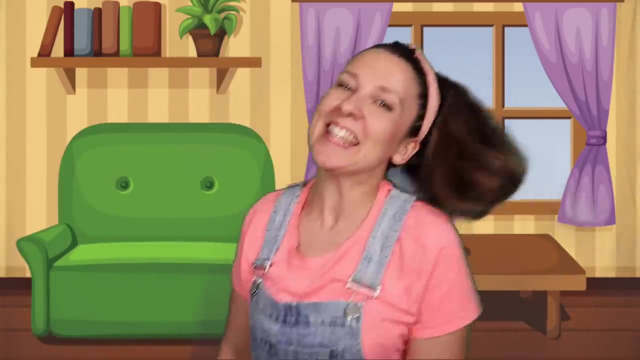 us Good job, Let's sing: Hickory Dickory Dock. Yay, Hickory Dickory Dock. The mouse went up the clock. The clock struck one. The mouse went down. Hickory Dickory Dock. Let's do it again. That was so much fun. 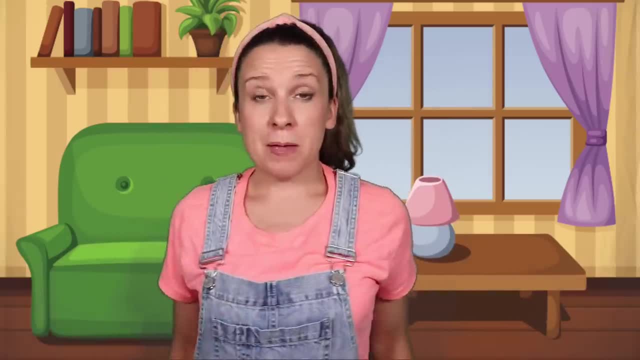 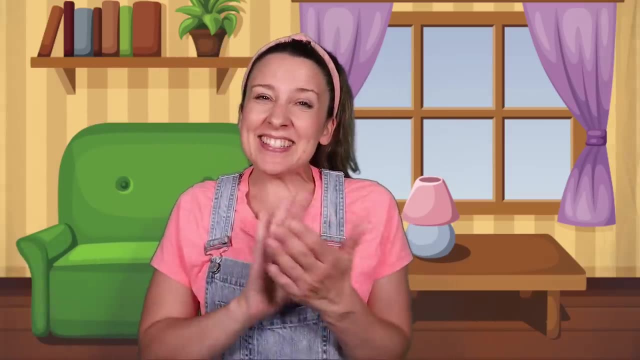 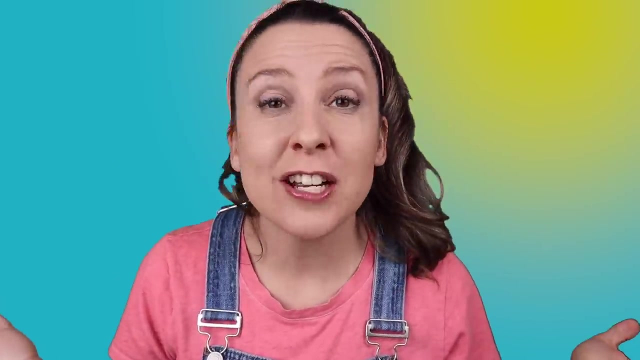 Let me hear you sing: Hickory Dickory Dock. The mouse went up the clock. The clock struck one. the mouse went down. Hickory Dickory Dock, Great job. Maybe if we make a fire truck sound really loud, another fire truck will come out, Weee. 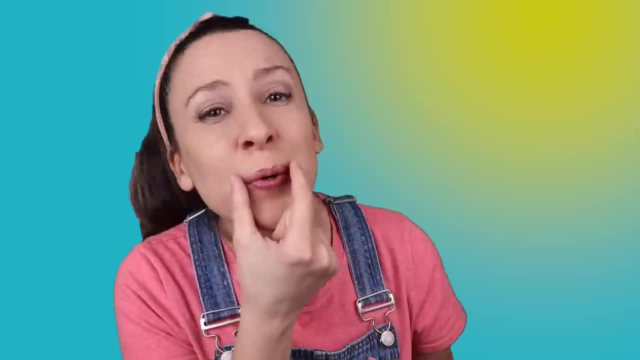 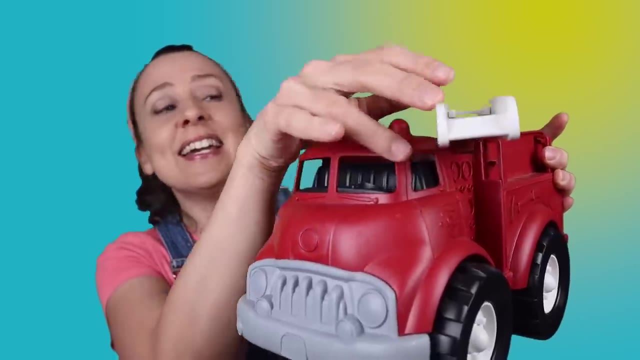 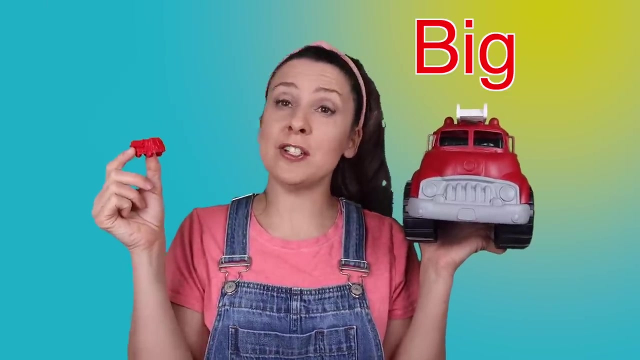 ception: Wow, A bomb chop, Weeee, Weeeee, Whoa, Wow, Whoo, Wow, Whoo, Whoa. Ahh Woo, Whoa, Whoo, Wow, big fire truck came out with a big ladder. Whoa, This fire truck is big and this fire. 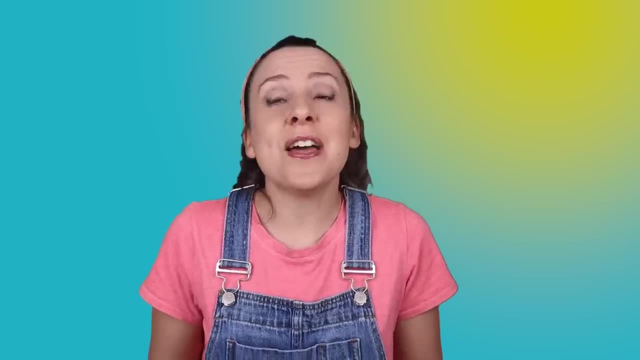 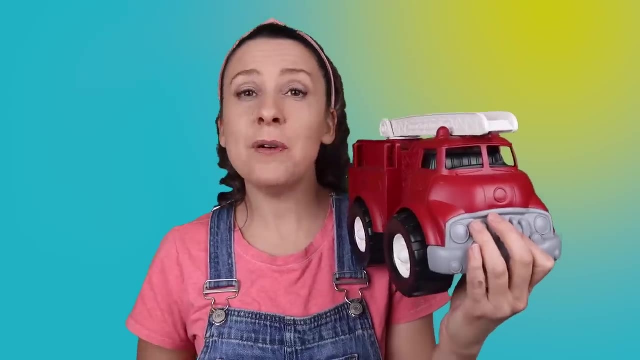 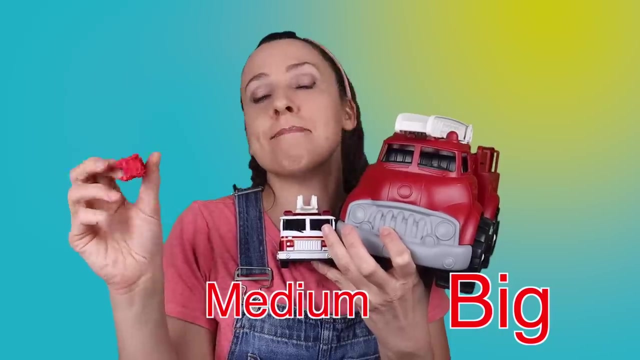 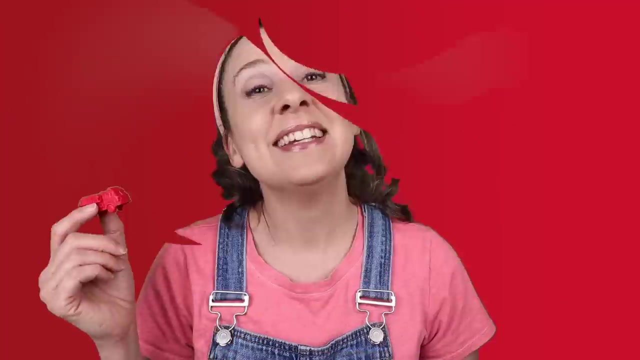 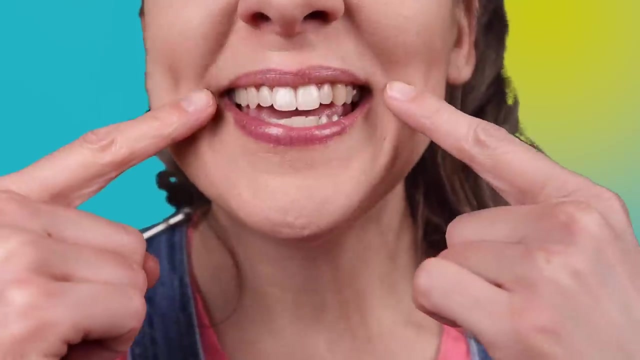 truck is small, I found another one, Whoa. So now we have big, medium and small. So small, Big, medium and small. Wow, Now let's make it go slow. Wee-oo, Wee-oo, Wee-oo. 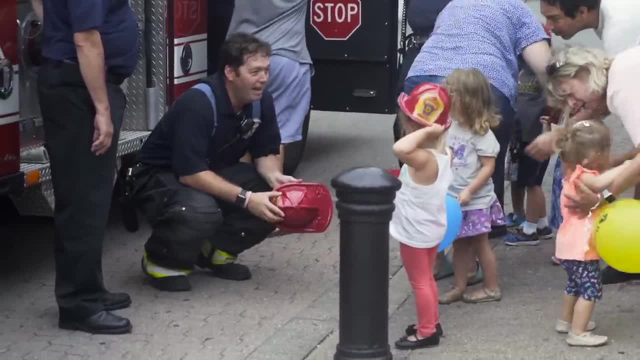 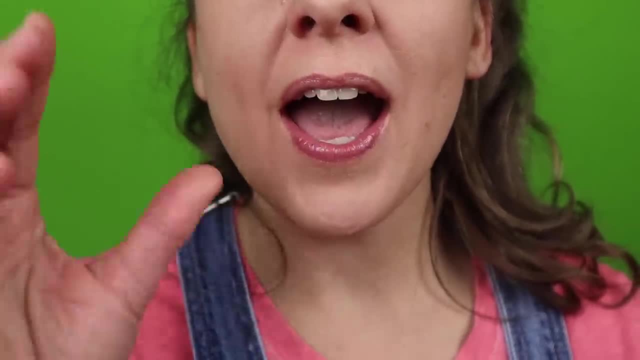 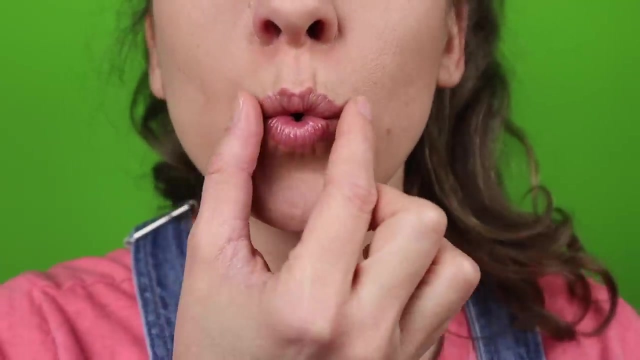 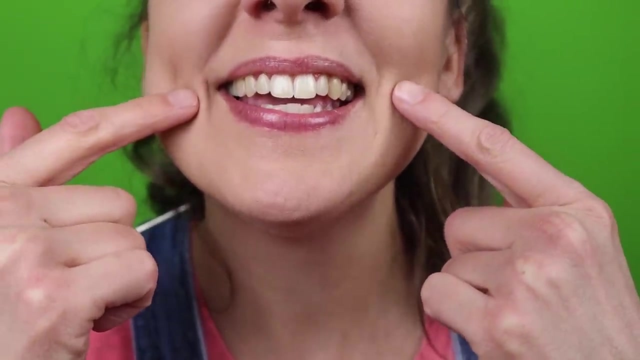 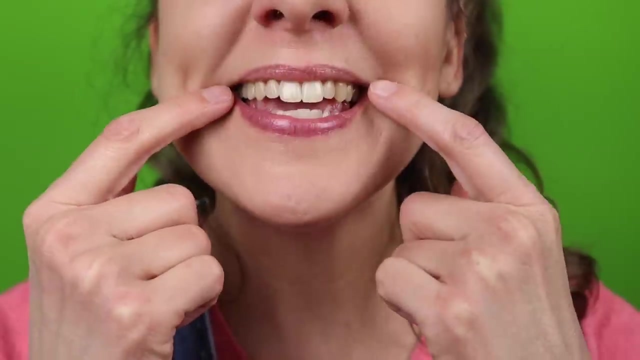 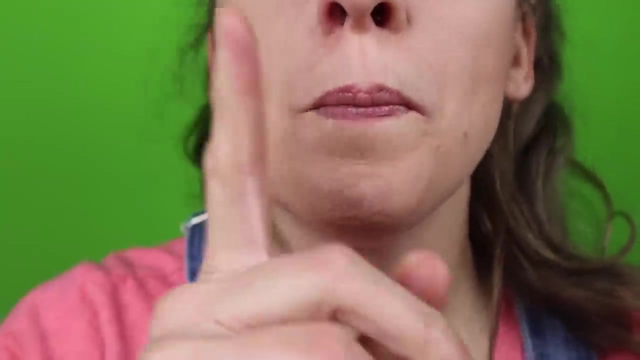 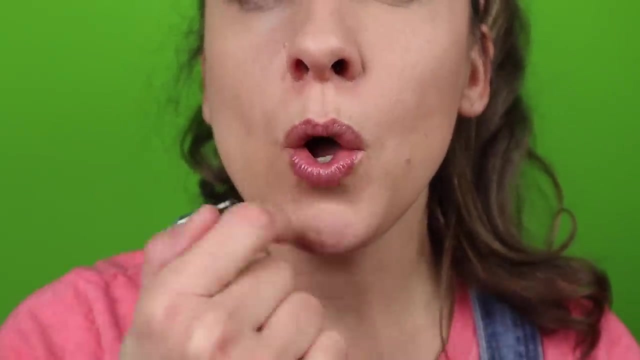 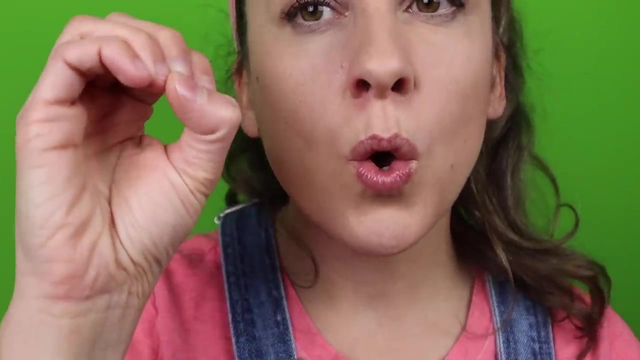 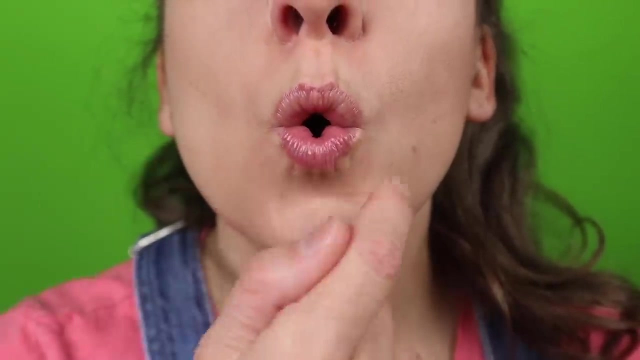 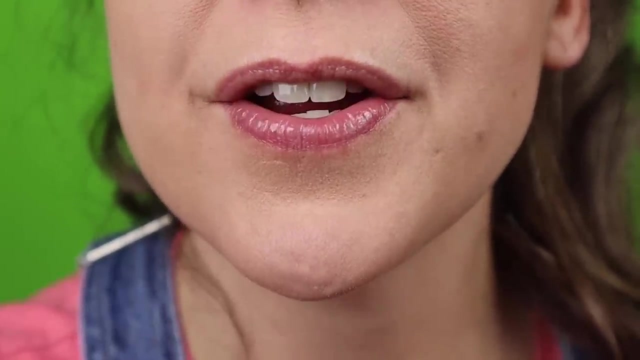 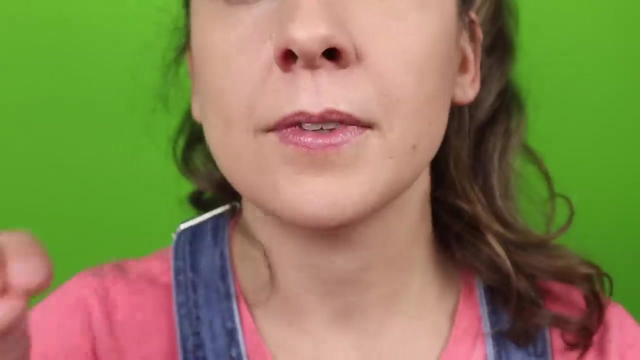 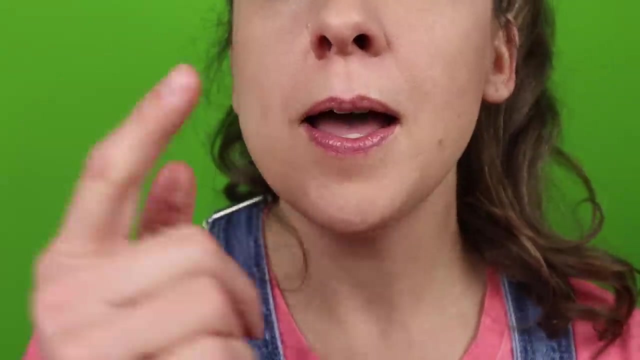 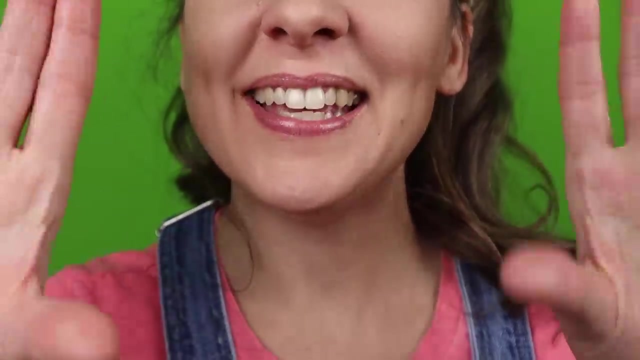 Wow, Wow, Wow, Yummy, Yummy, Yummy, Open, Open, Open, Open, Open, Open open, go, go, go go Water, water, Up, up, up, up, Yeah, yeah, yeah. 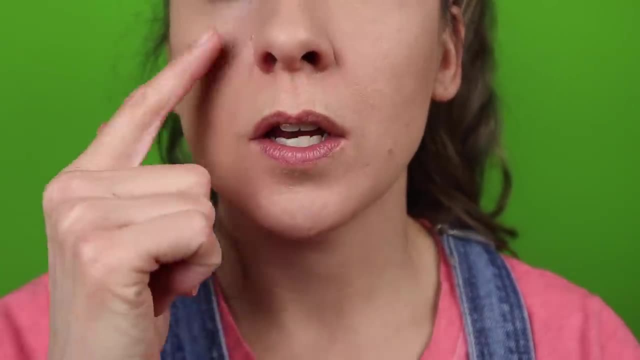 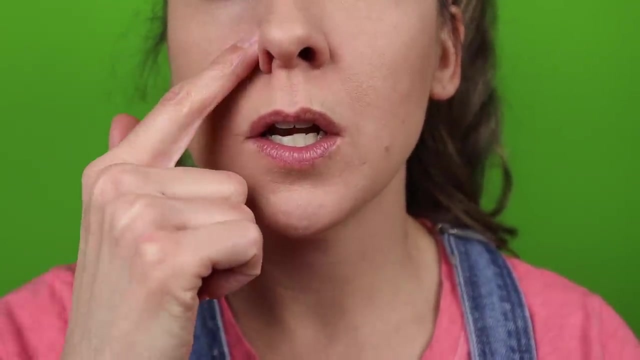 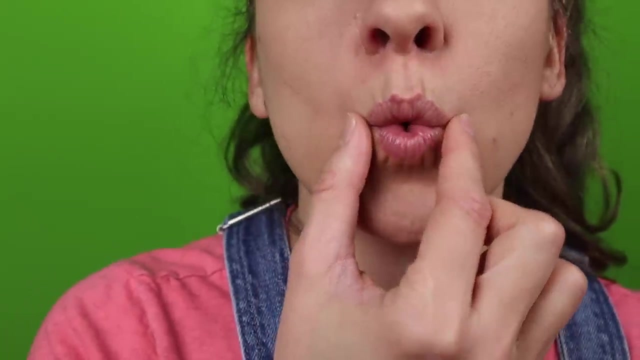 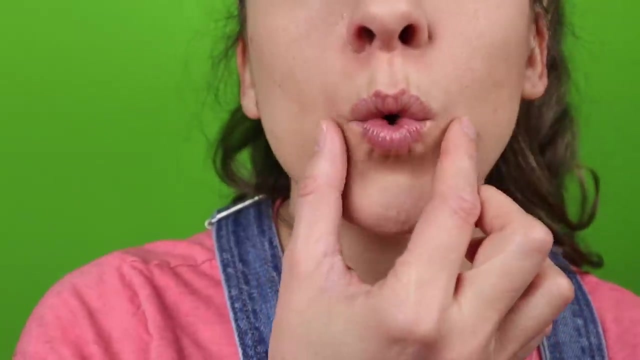 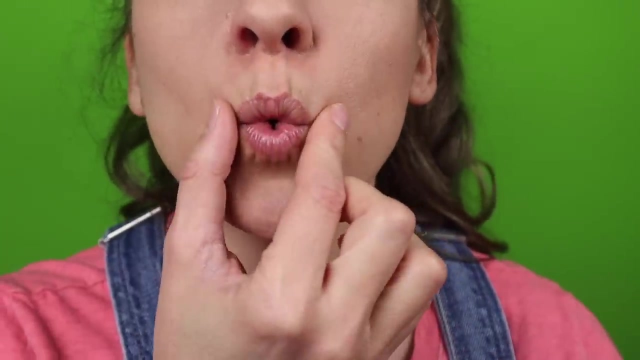 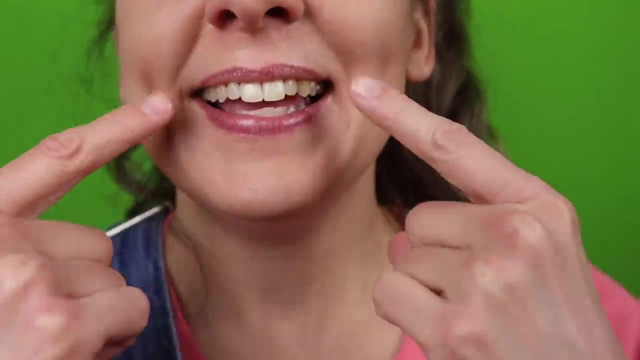 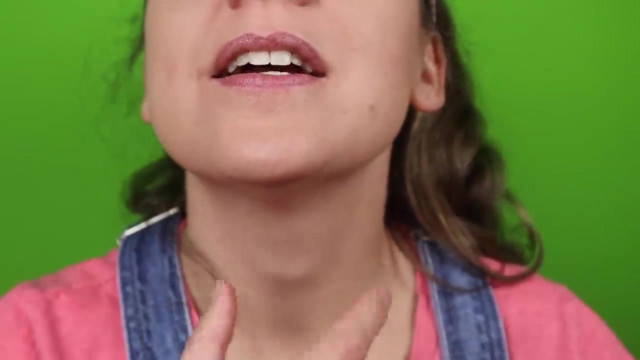 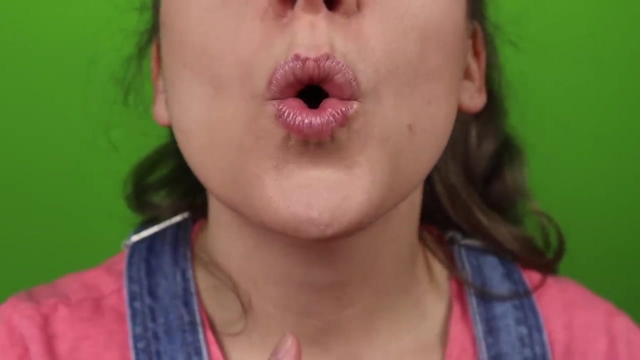 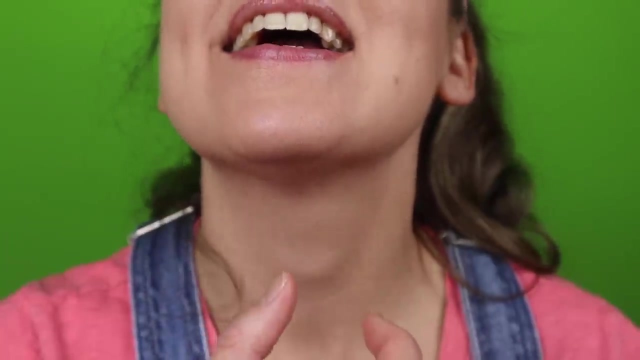 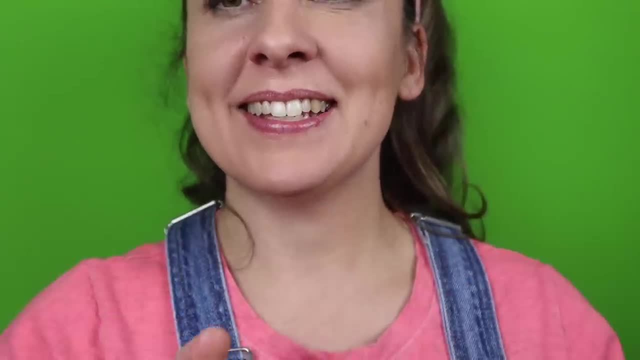 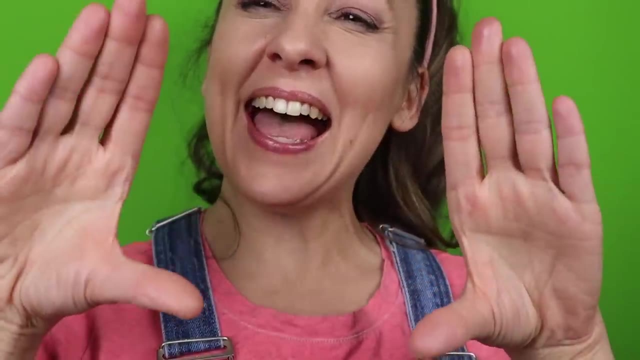 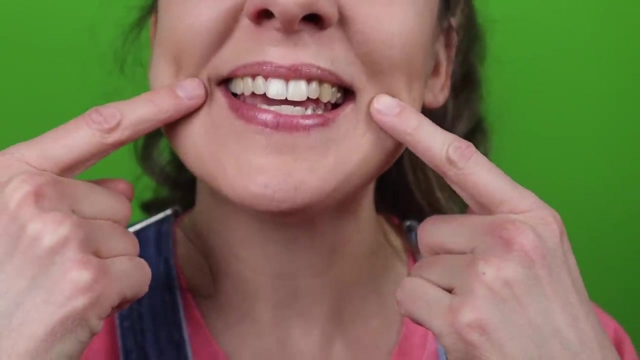 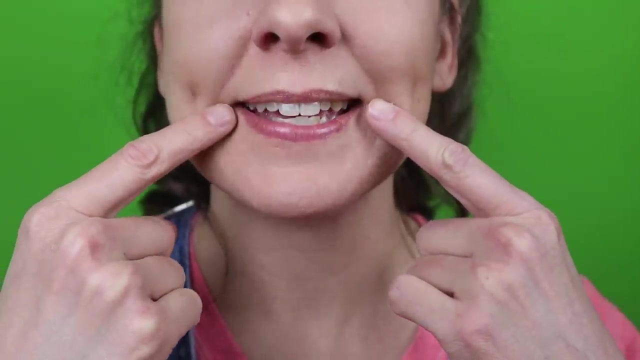 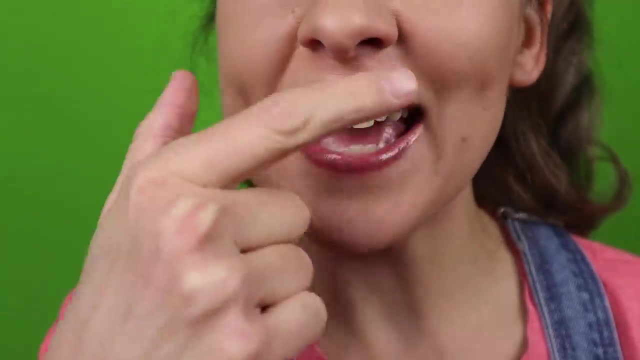 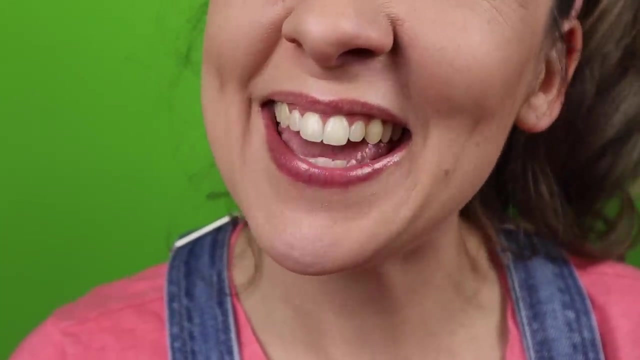 Yee-haw, yee-haw, yee-haw, yee-haw, yee-haw, M-me, m-me, me, m-me, m-me, me, R-red, r-red, red, red. 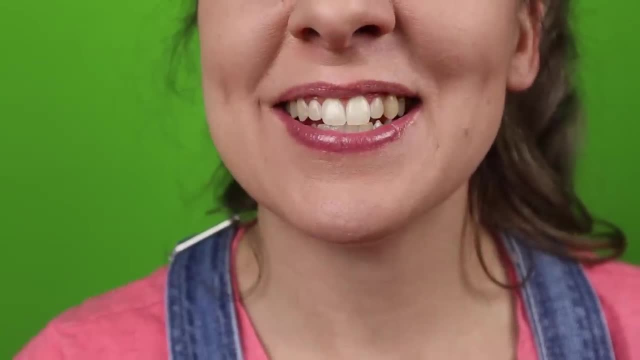 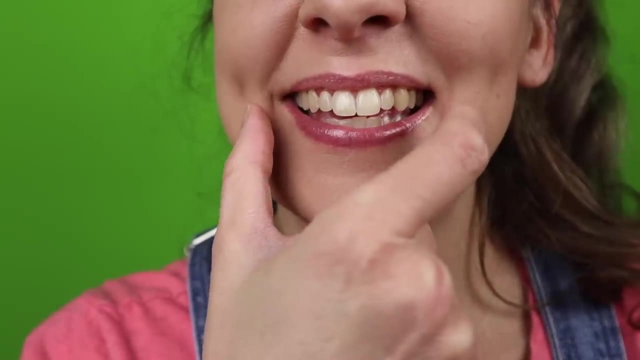 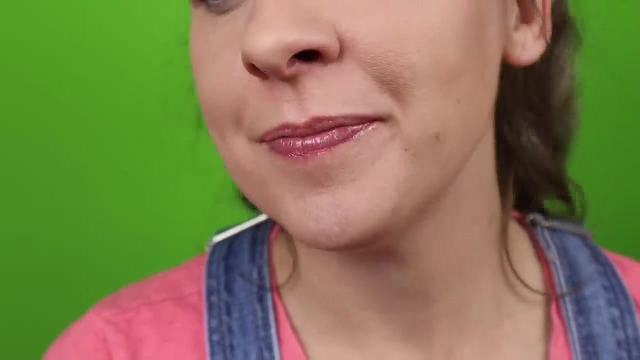 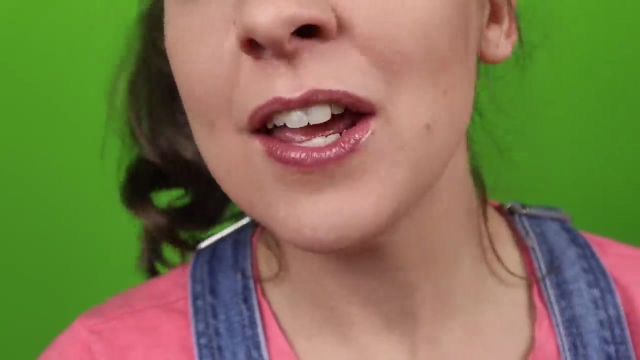 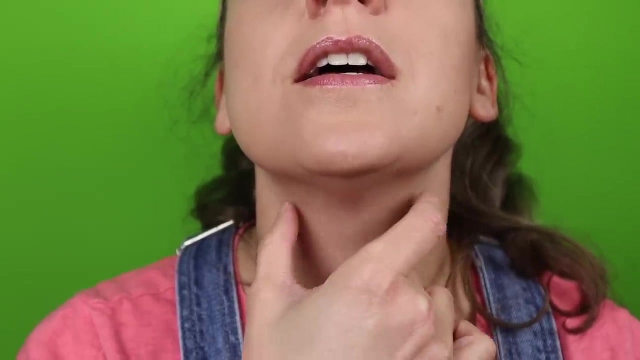 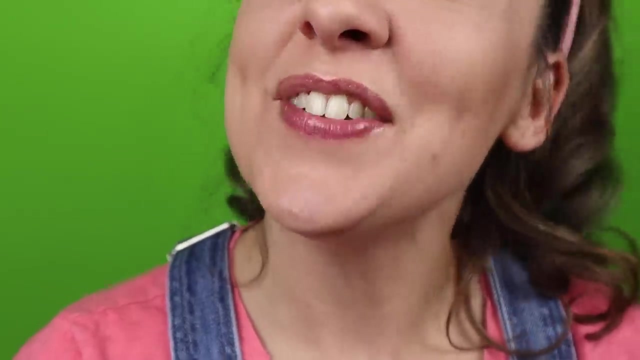 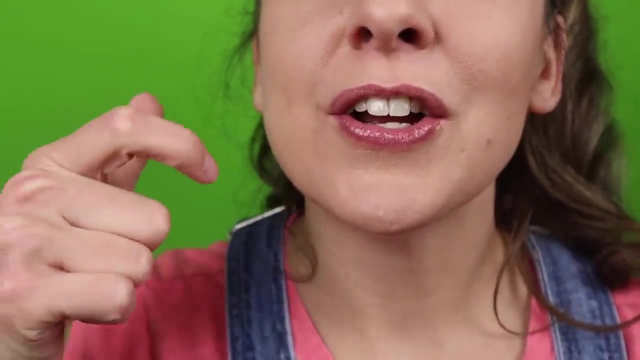 Orange orang, orange, orang, Yeel-le-o, yeel-le-o, yeel-le-o, Yeel-le-o. Yellow, red, orange, g, g, g, green, green, green Red starts with R, r, r, r, r, r r. Yellow starts with Y, y, y y. green starts with G, g, g, g, g, g, g. blue starts with B, b, b, b. blue blue. blue purple starts with P, p, p, p, p p. purple starts with: